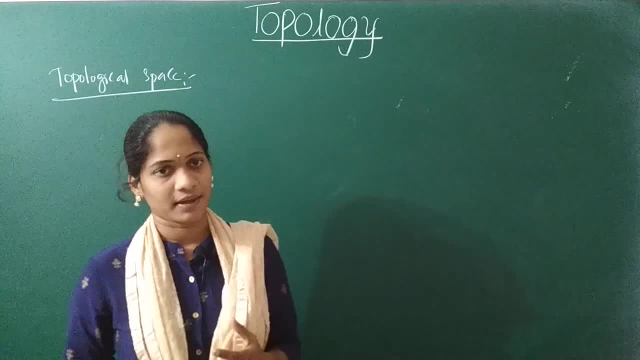 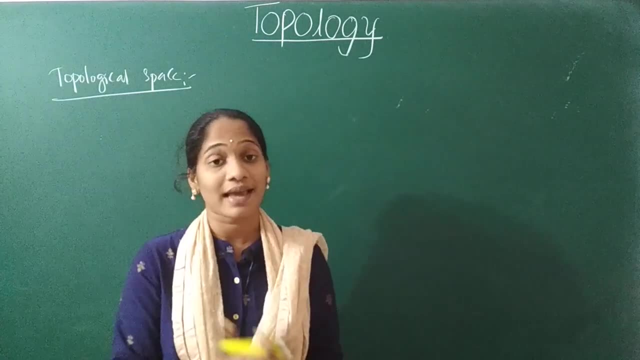 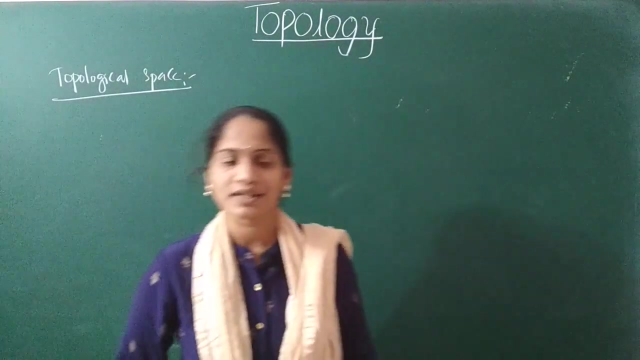 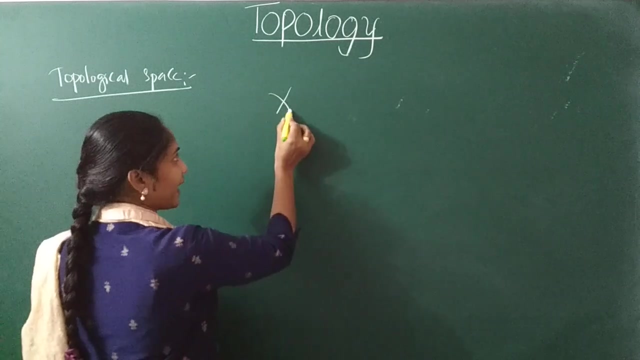 definitions here. it is some theoretical, theoretical and matters definitions. with a grip under them, it is very easy to go through the proofs or, in some definitions, examples, right. so the first definition is that topological space. what is that topological space for that? let us discuss some overly. what is a topological space here? let us consider x. what is x here? x is nothing but it. 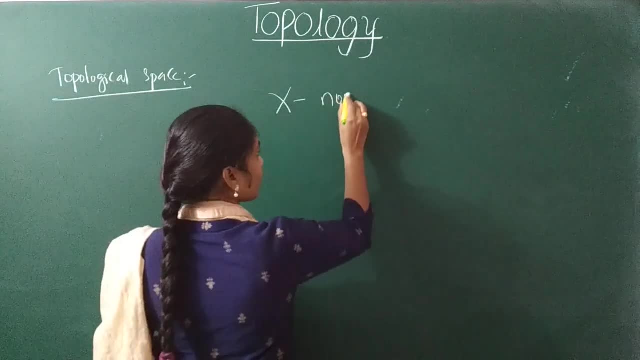 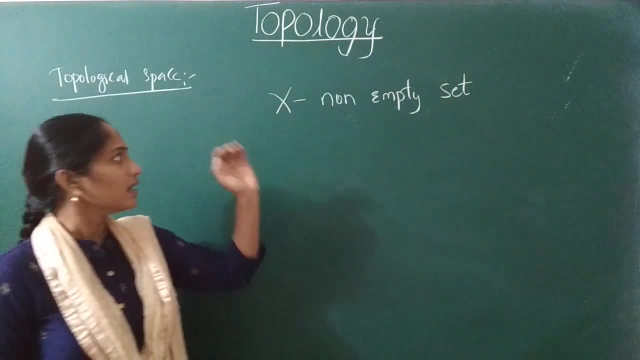 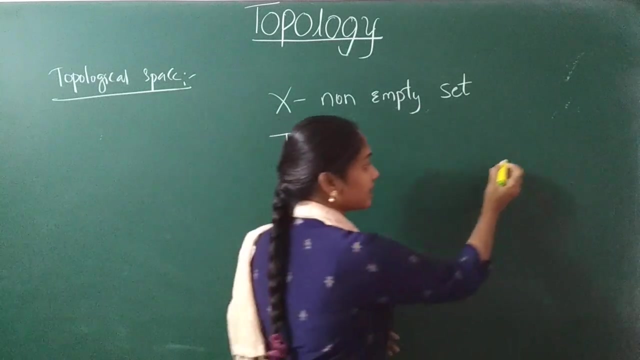 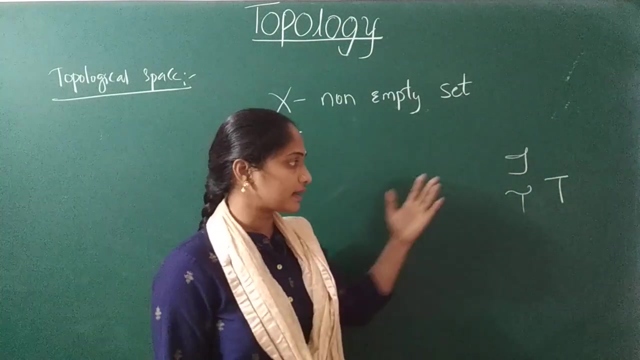 is a non-empty set. non-empty set. right here i'm considering some x. next i'm considering t. what is t here? in some textbooks it it may be represented like cap some i, or else like this, or else by dark d. if you go to any siemens like 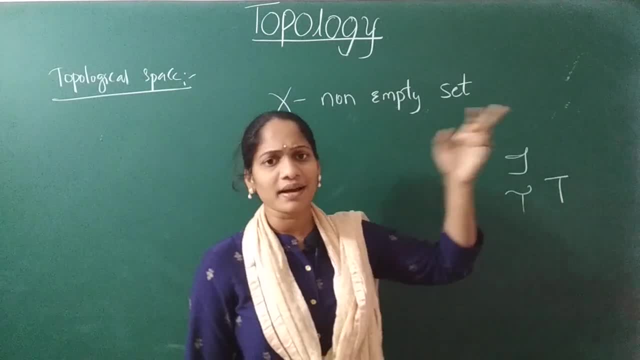 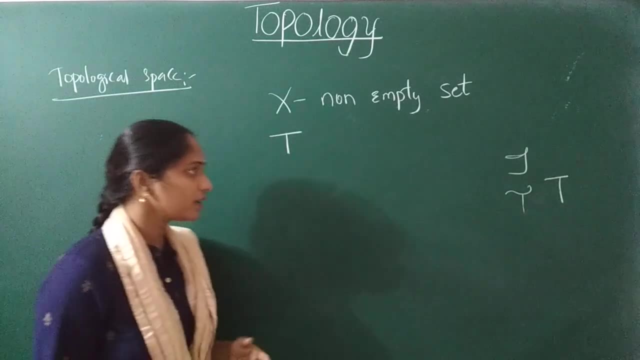 textbook. um, you can still observe like dark t in some other textbook, like malik you can see here. so these, these types of notations represented, maybe you can observe. so here i am representing the topology by t here. what is this topology by t here? what is this topology by t here? what is this topology? 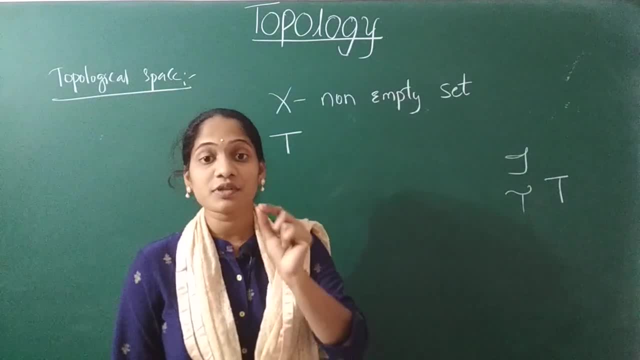 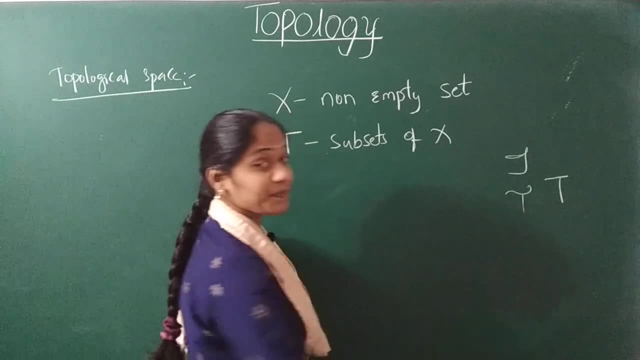 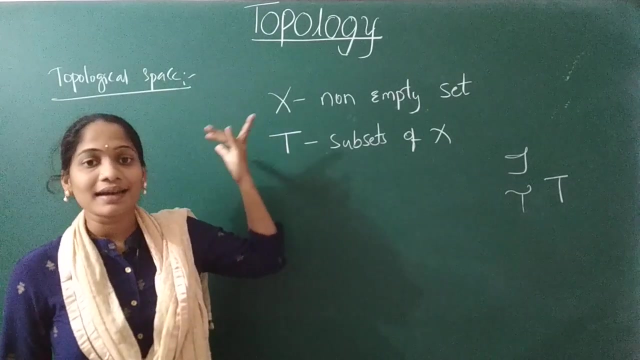 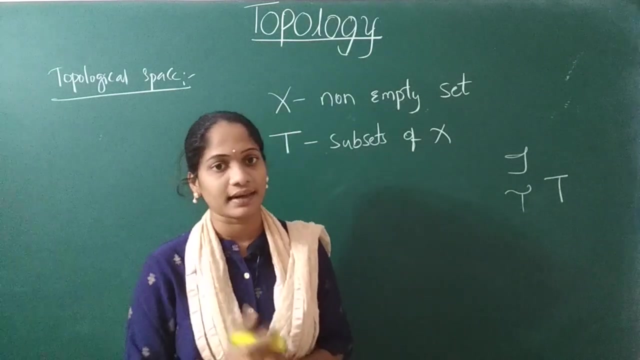 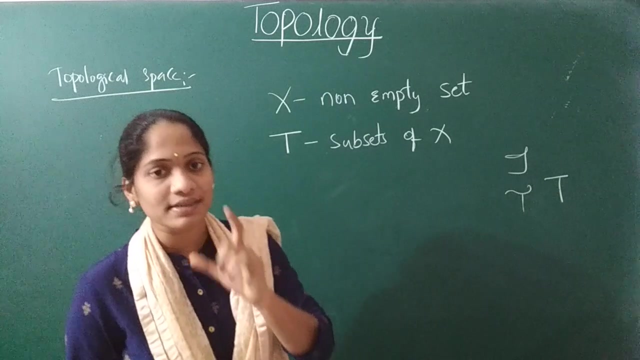 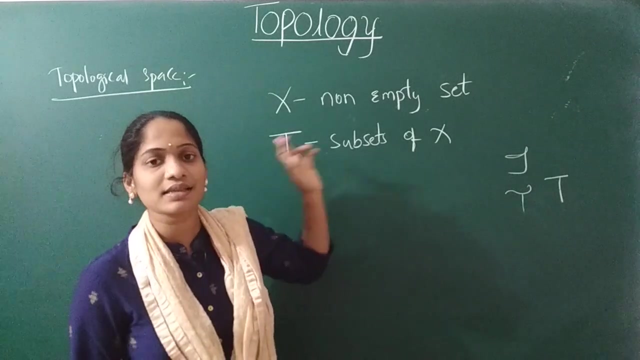 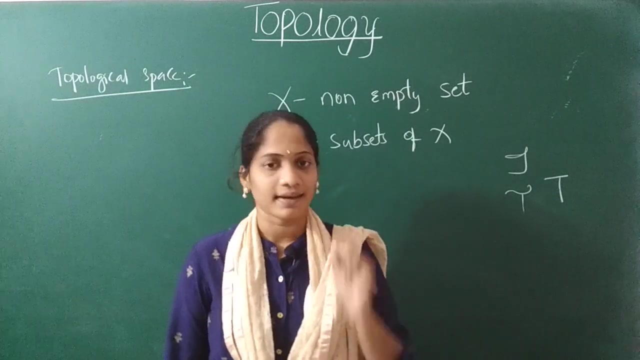 what is this? this t is the subsets of x. what is t here? subsets? have you got it here to know about the topological space that you have to consider a set right and next you have to consider some t. what is t? it is the subsets of x, and that t is known as the topology on x if satisfy some three conditions. the first: 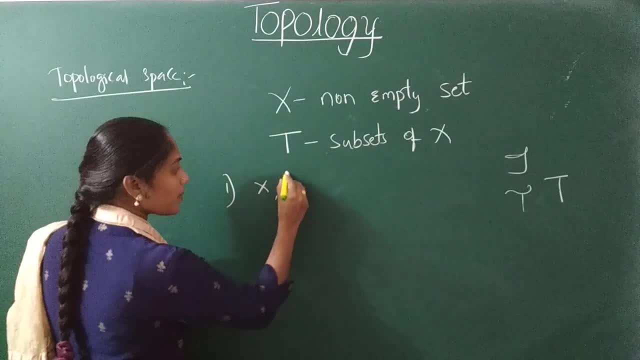 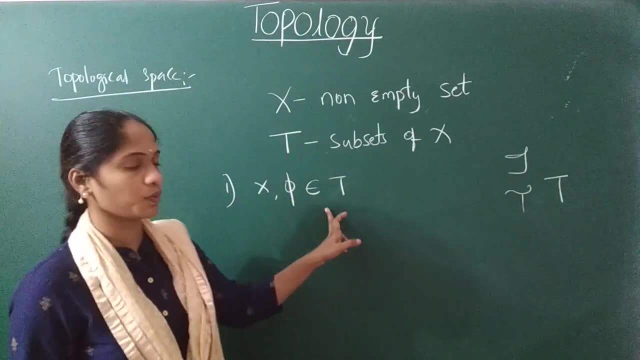 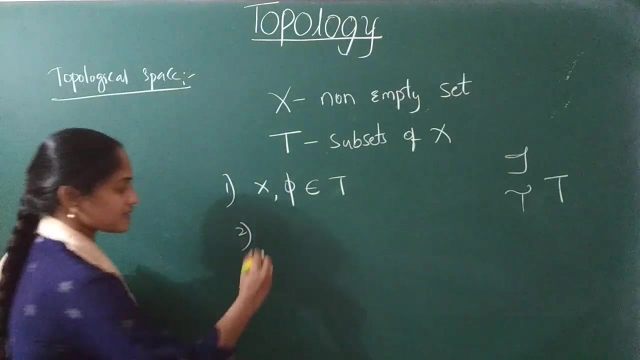 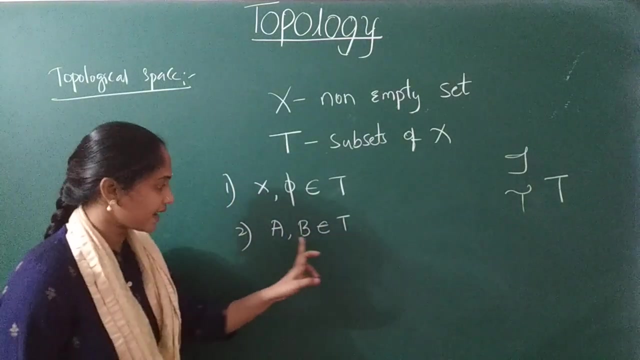 condition is that x comma pi should belongs to t, got it. what is the first condition? x comma pi should belongs to t. coming to the second one, if so, now let us see. the second point is that you have to consider two sets. which belongs to tau, got it. you have to take two sets that belongs to tau and. 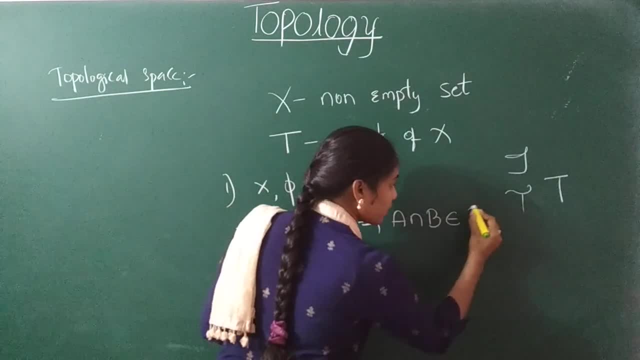 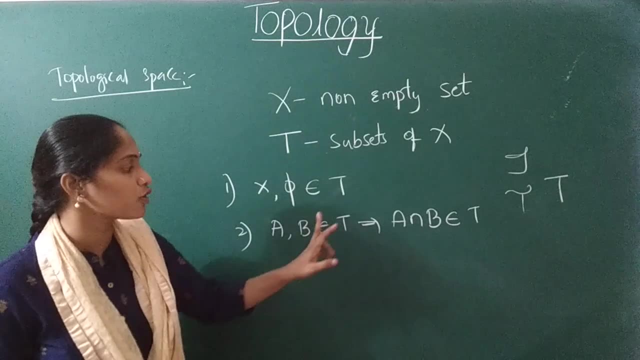 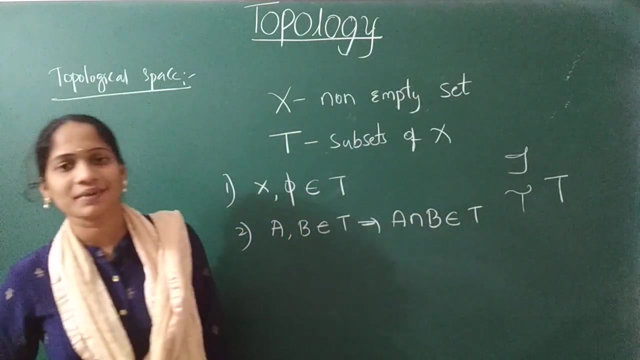 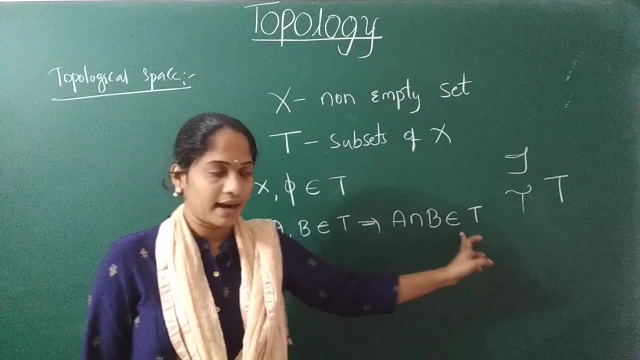 here. its intersection should also belong to tau. got it here. you have to consider two sets, that two sets should belongs to tau and the intersection should also belongs to tau. right, and in similar, theoretically, what you have to say: finite intersection of tau is again a member of tau. and then you take two sets of tau and that set of two intersections should also be in tau. 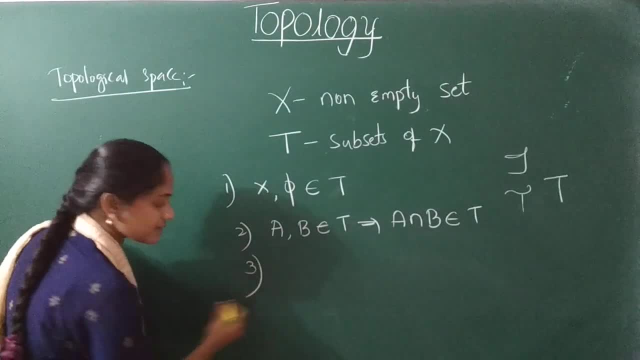 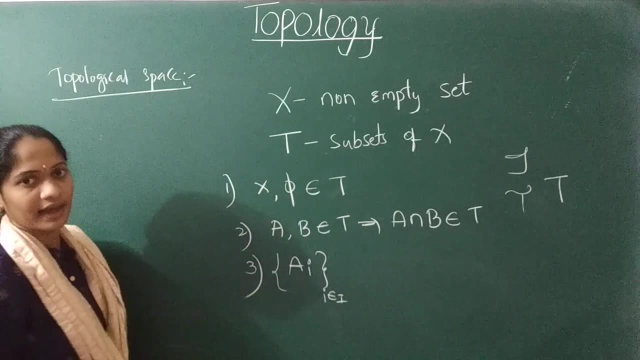 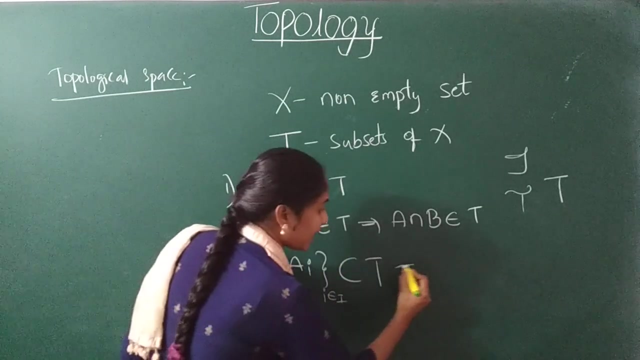 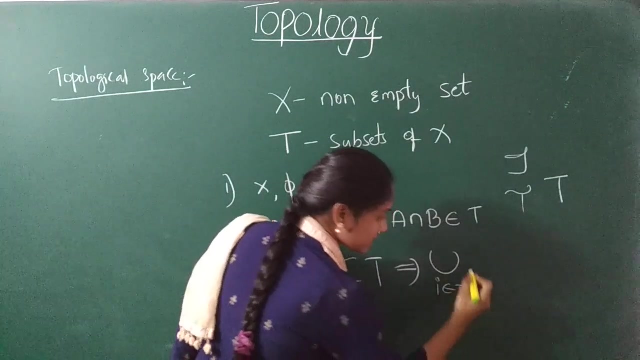 that is the finite intersection. and the third is that if you consider arbitrary, i belongs to index set i. if you take some collection of sets a, i's, which are all subsets of tau, and that implies their union, arbitrary union, here i goes to the index set i, arbitrary. 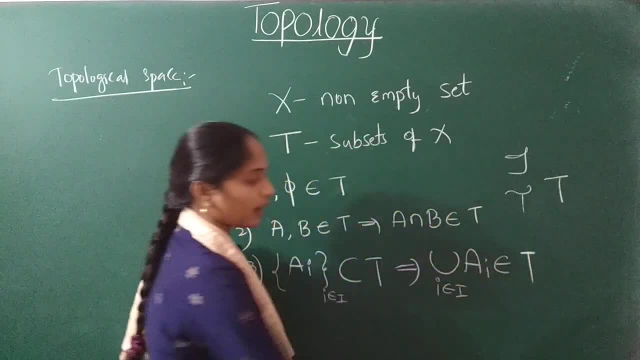 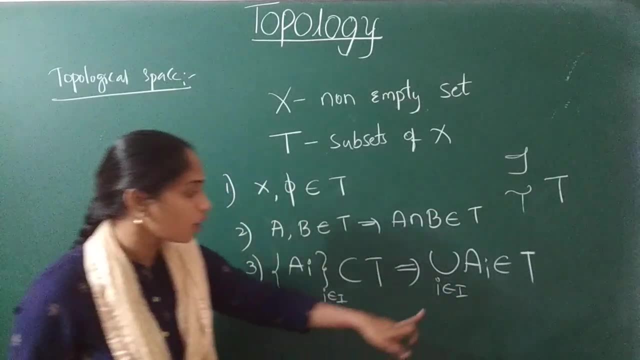 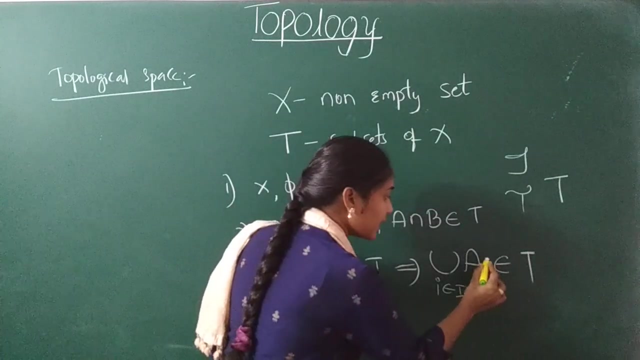 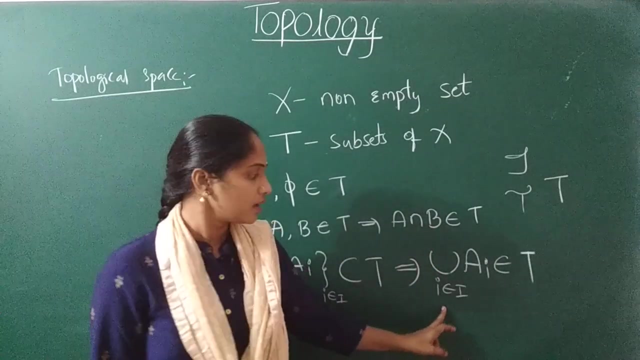 union of this should also belongs to tau, got it? if you take some collection of members of tau, their arbitrary union. why you representing the word arbitrary? because this small i belongs to capital. i means that index is set, not finite intersection, a more finite tundali union, cochesi, arbitrary right, so alami. 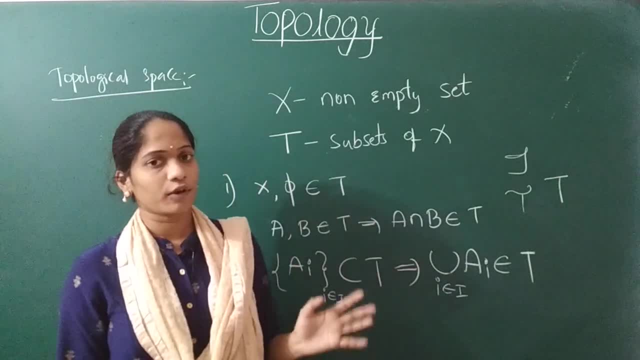 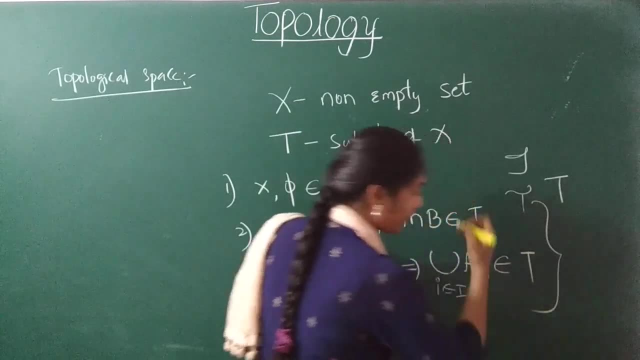 this is the theoretical, theoretical definition of topology. if you, if you will solve some example, it will be clear. so now, what you have to do, this is, you have to remember, is that this is the finite intersection and this is the f on placed Ö is the joining matrix and this is the 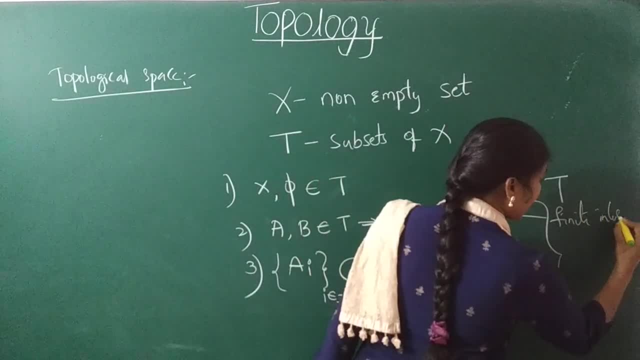 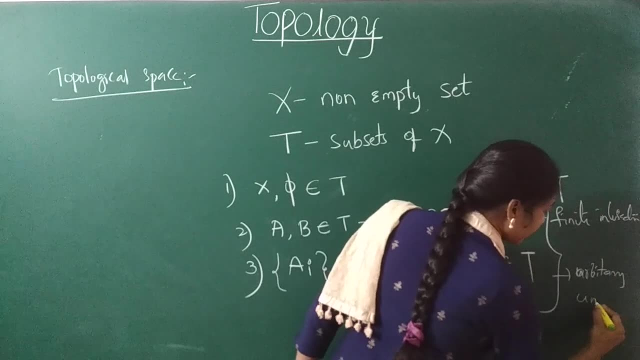 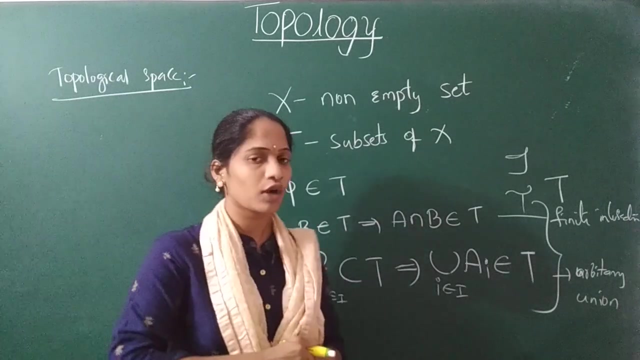 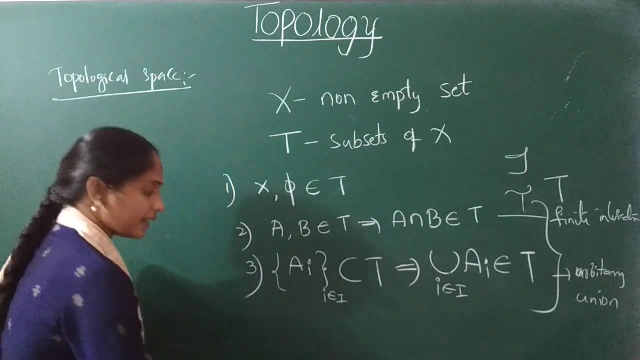 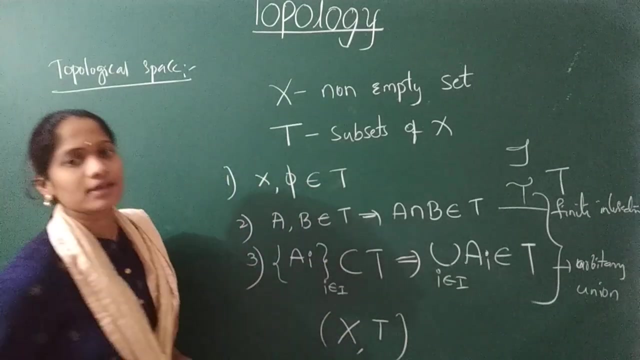 the organisation. that means let's write the finite intersection if quantify is equal to zero. If it will be clear for you what is an algebraic structure Here, X, the non-empty set, X, Equibed with tau, is known as the topological space. 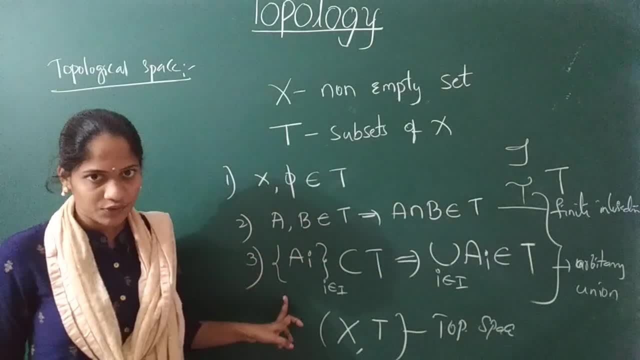 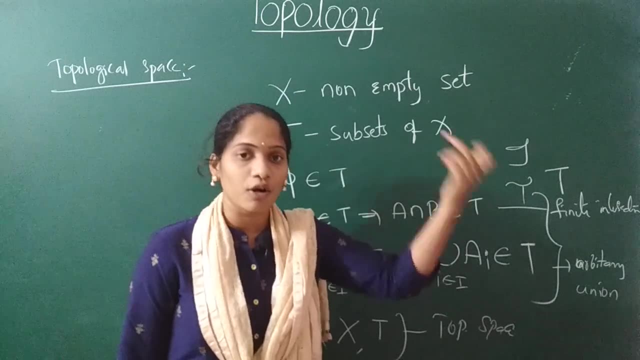 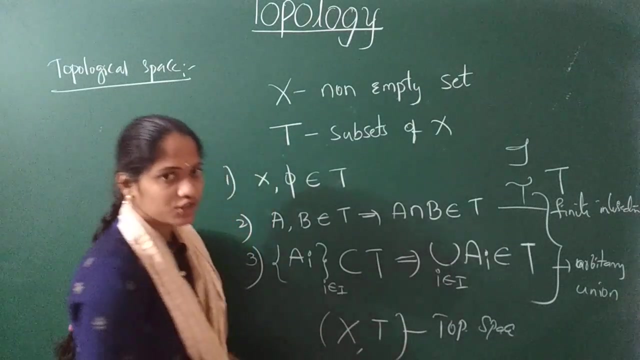 Got it. If these three conditions are satisfied, This tau will be there, right? That tau is your topology on X. What do we call it Topology on X? When it satisfies these three conditions With X, this structure, algebraic structure, is known as topological space. 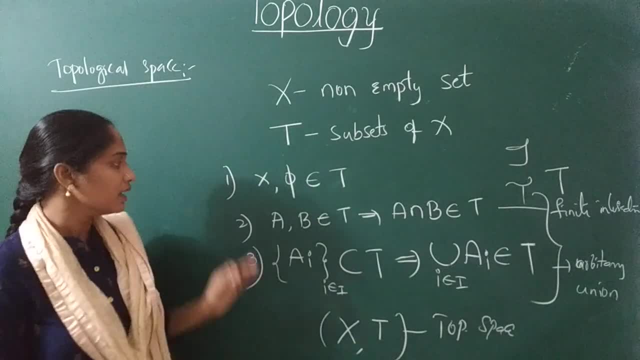 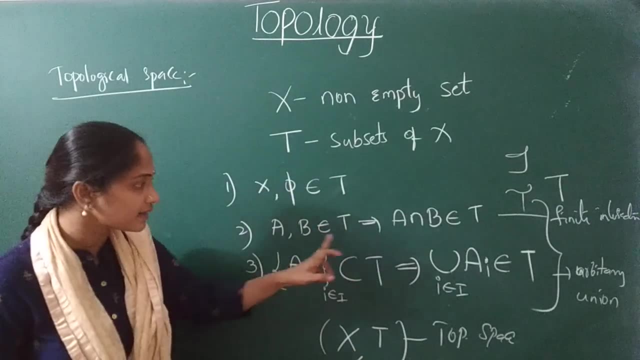 So this is your topology definition. You have to remember is that The first one, X, pi, that is, the non-empty set, should belongs to tau. The finite intersection, the finite intersection of member of tau is again a member of tau. 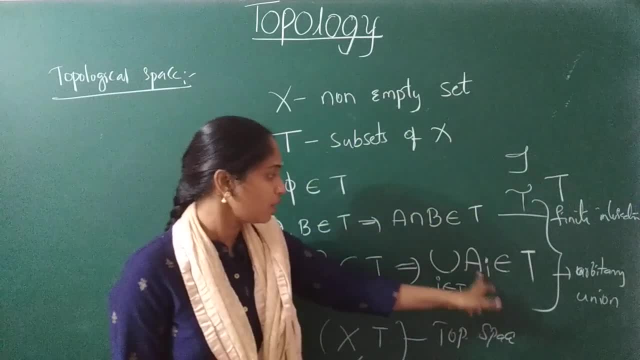 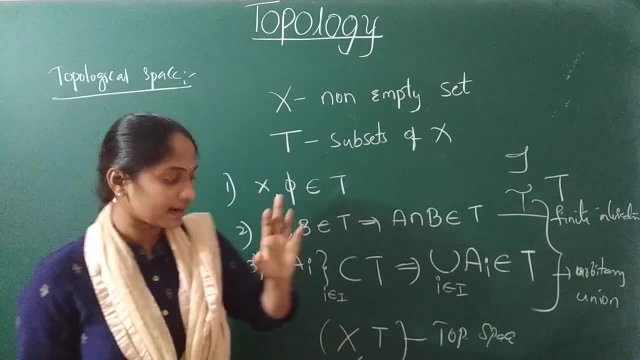 Orbitary union of member of tau is again a member of tau If these two three conditions are satisfied. This tau is known as a topology on X, And the algebraic structure X with equipped with the tau, that is, three, is known as a topological space. 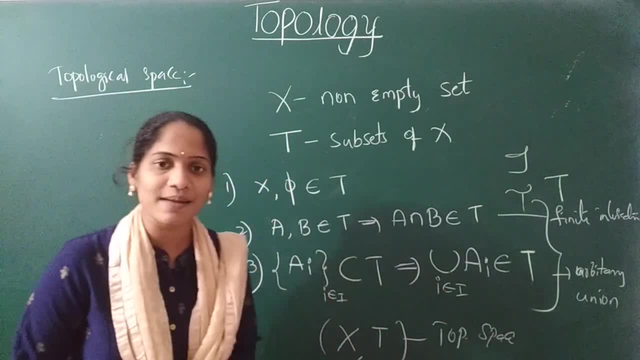 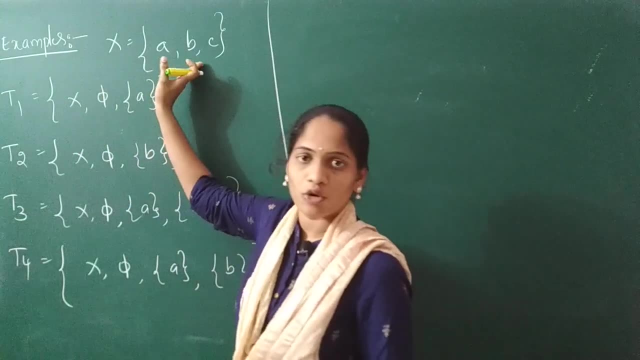 So this is your definition. let us discuss some examples. it will be clear for you, right? So here let us see some examples. I have taken X. this is any non-empty set which is considered in the elements A, B, C. 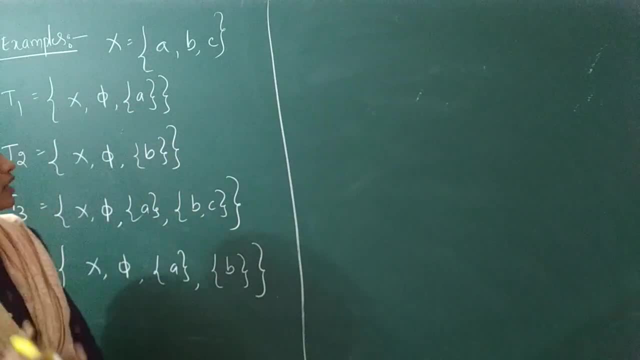 A B C, not A B C, A B C. there are three elements in the set X. Now I am considering some T4, that is four topologies, that is four sets. these are all. 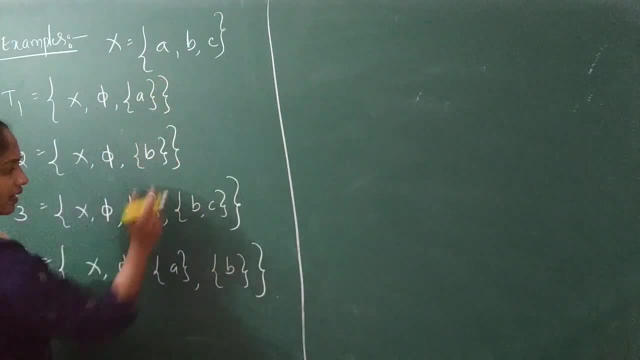 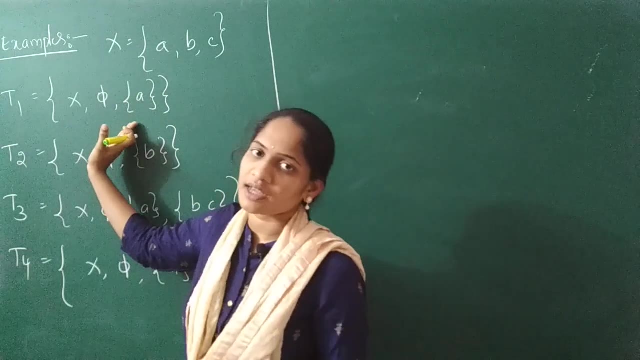 See all these subsets. singletons are AN, B, AB. We have already said T, that is which is taken in the topology and what all we need to do. There are subsets here for X, right. First we have to look at it. 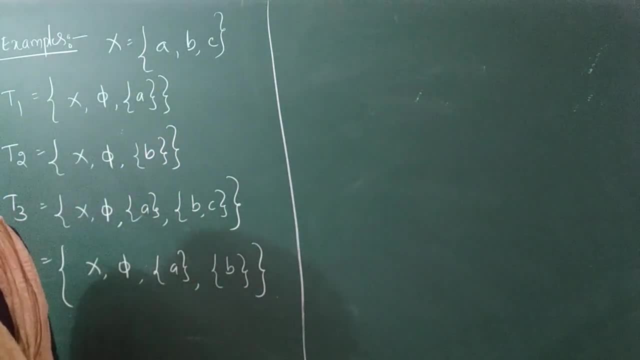 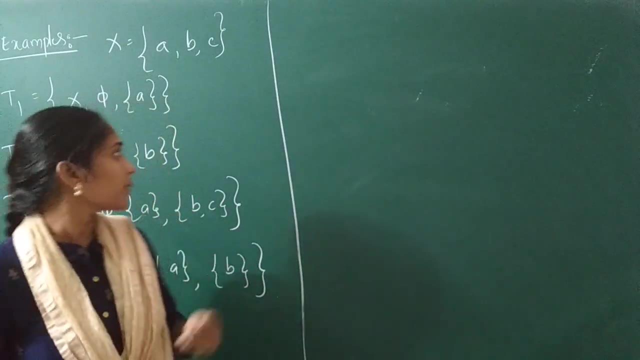 Yes, these are all subsets of X. Now, what is next? we have to prove that These taus are topologies or not. For that what we have to do for every tau. For that what we have to do. 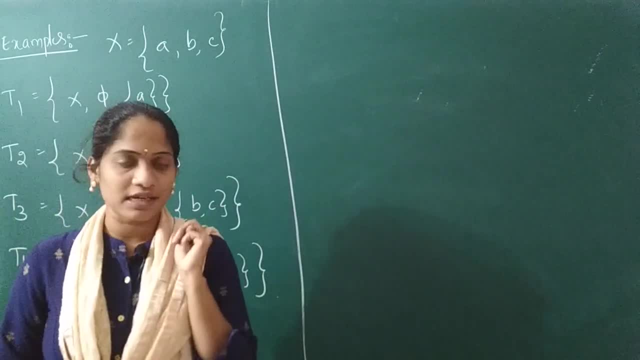 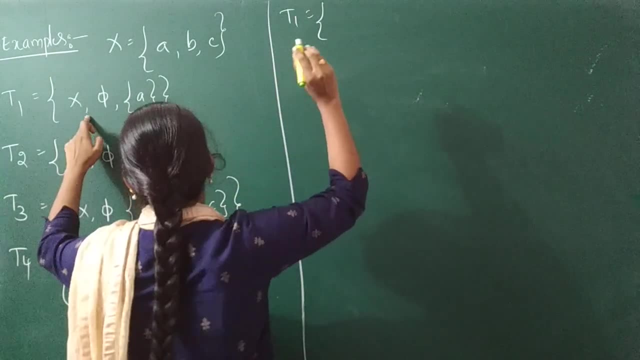 What you have to do in each set is to check if the three conditions are satisfied or not. So let us take the first one, T1.. What is that T1?? How many elements are there? Sets are there? subsets, are there x, pi and singleton set A? 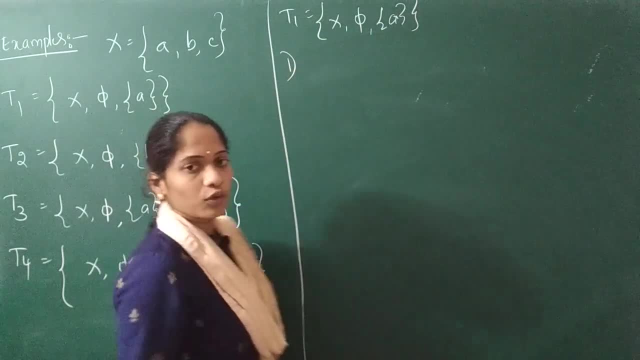 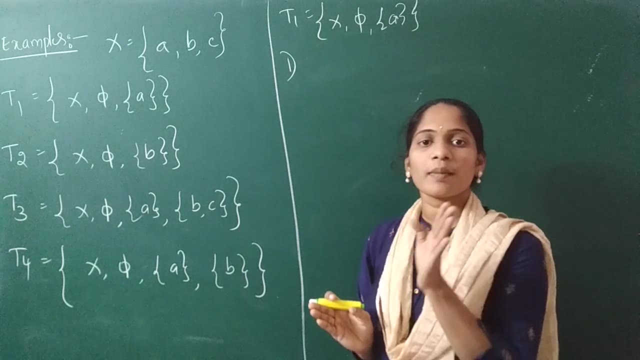 The first point. what is that first point? To prove this, T1 is topology on x or non. the first condition is that x, pi belongs to tau or not. Here here, T1 is there tau 1.. So tau 1 should not be there, right? 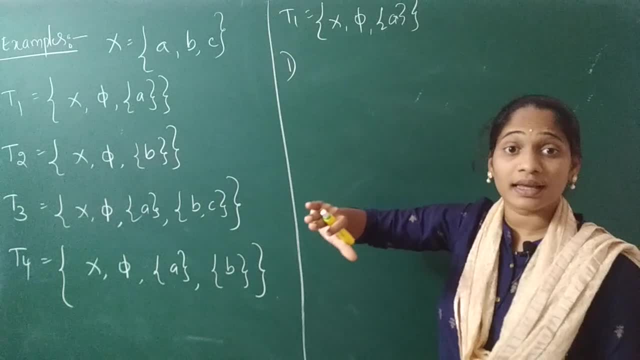 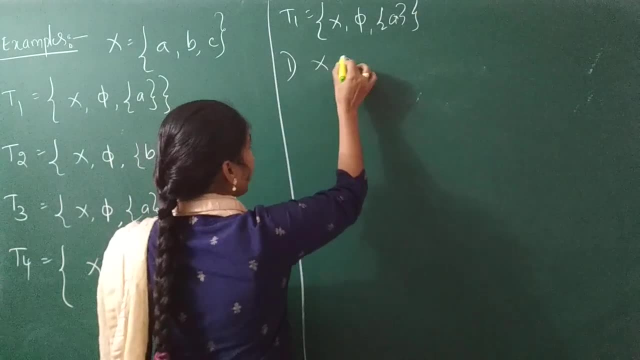 So T1 is there In T1,. what should be there in T1?? x pi should be there. right Check. is there x pi? Yes, so it is clear that the first condition, x pi, belongs to tau 1.. 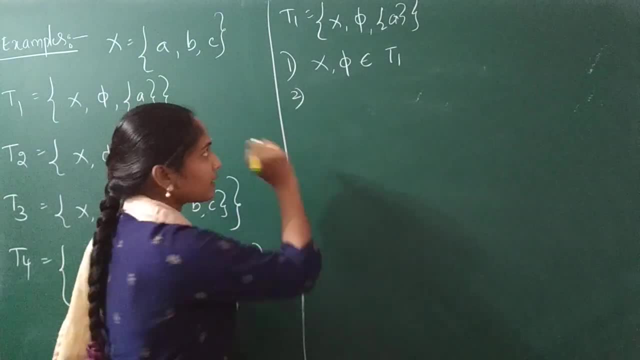 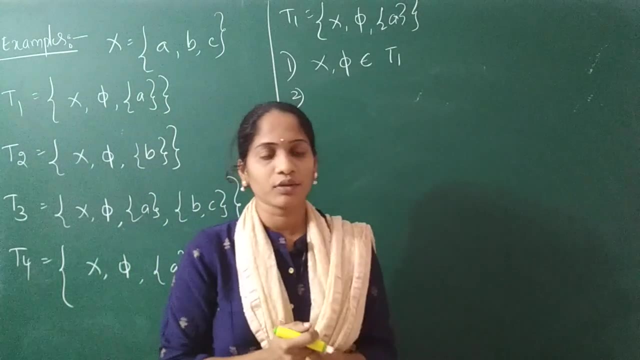 Yes, the first condition is satisfied. So next, the second condition is that finite intersection. You have to take Any two sets. finite means not taking once, three, four. You have to check for any two sets For that intersection. also you have to see if it is in tau 1 or not. 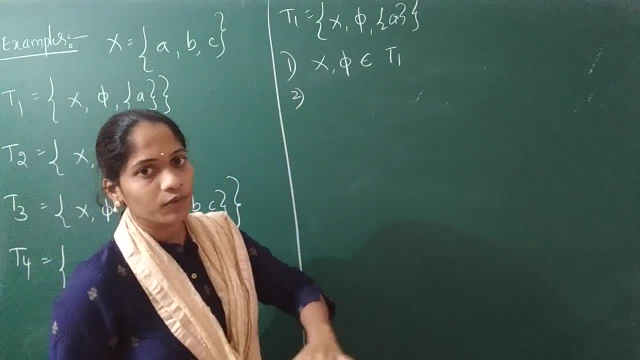 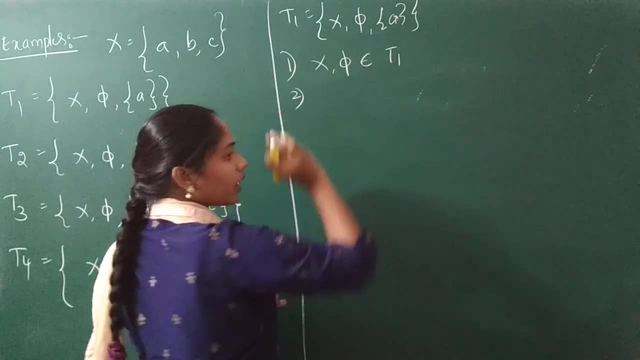 So I will do it one by one for your clearness. Next, we have to do directly, right. So now first, what you have to do. You have to take two sets and you have to do the intersection X, x, intersection pi, right. 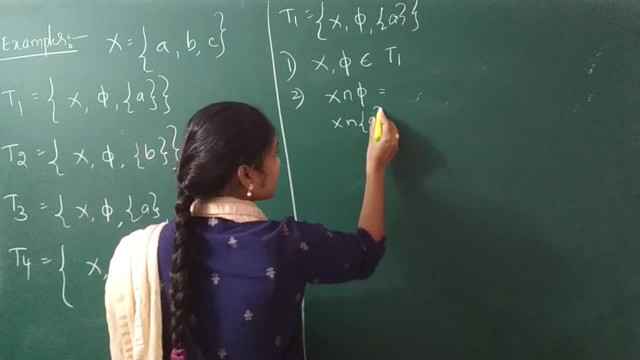 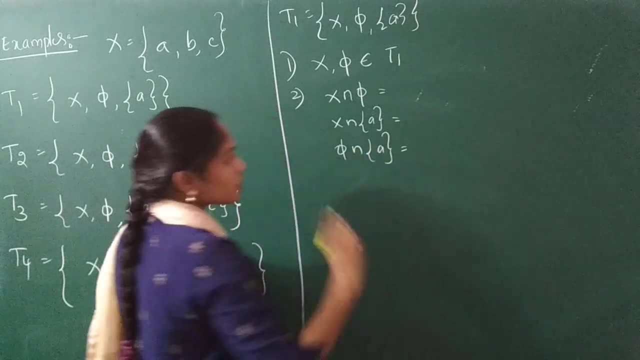 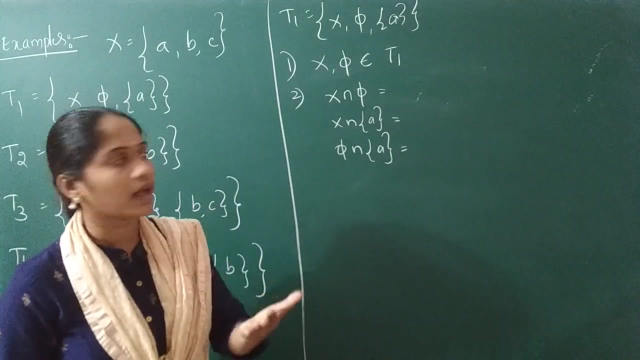 Next, x- intersection, singleton set A. And next, what you have to do, Pi- intersection, singleton set A. So what you have to do is you have to take two sets and you have to consider the intersection. Okay, You have to check if the intersection is in T1 or not. 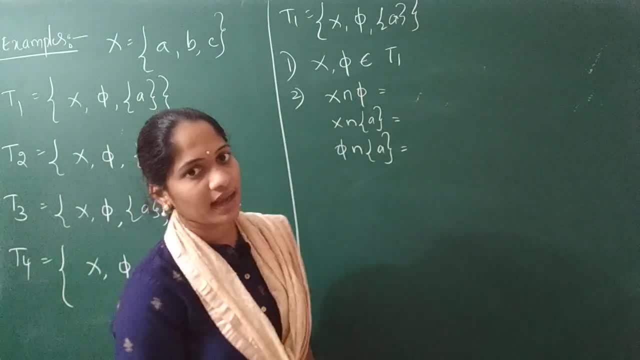 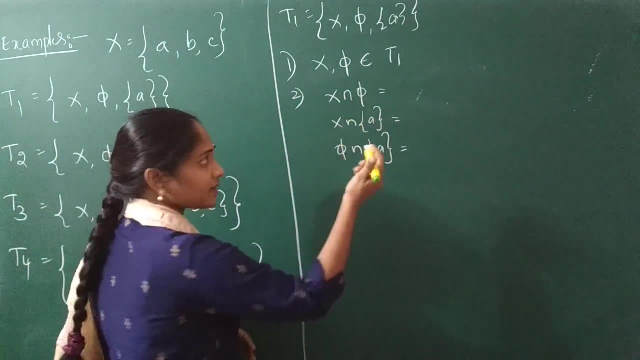 So what is that? x, intersection, pi. And you have to remember that empty set is and subset of every set, right? So intersection, what is the intersection? We will get pi If you take the intersection x, pi. 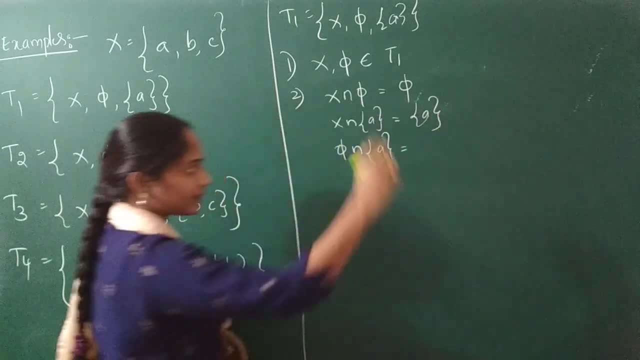 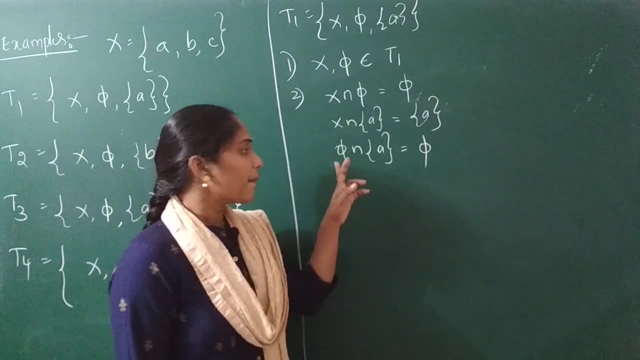 If you take the intersection x- pi, If you take the intersection x- pi, So there is a singleton set, A Pi intersection. this is pi. Just I have told you that pi, that is empty set, is subset of every set. 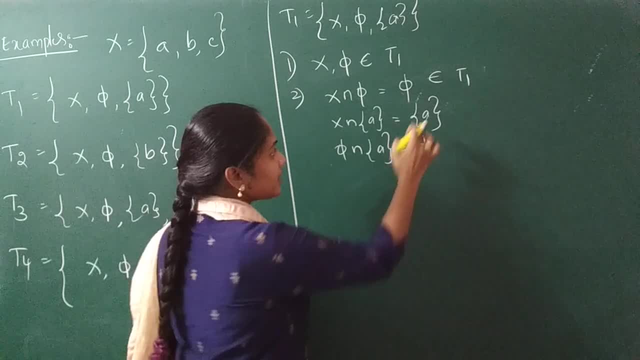 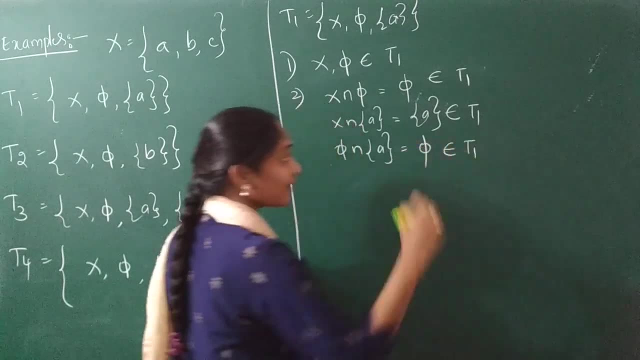 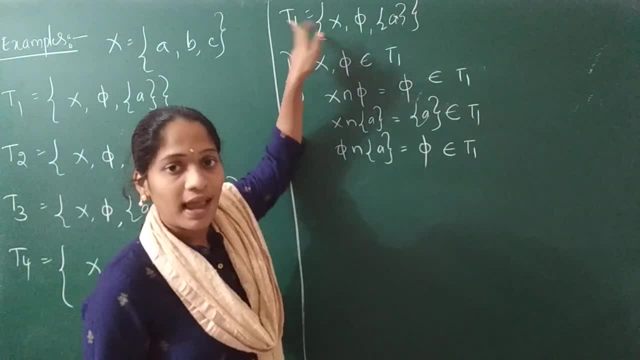 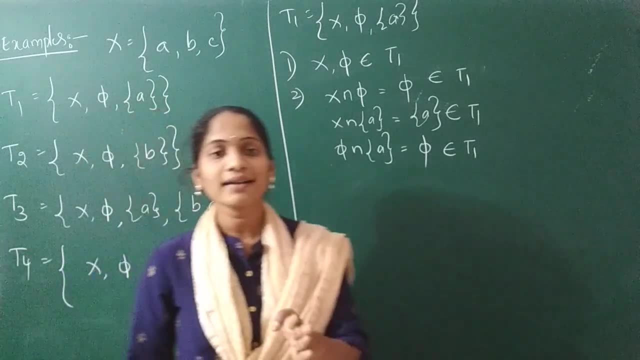 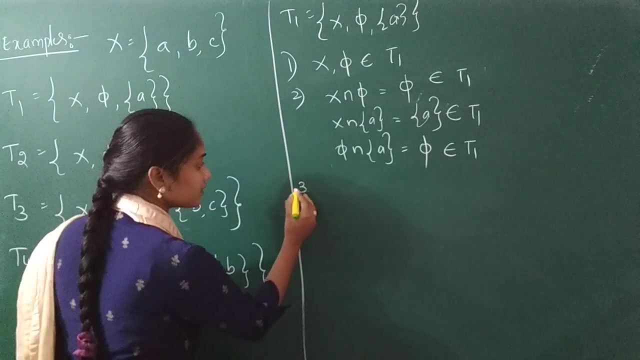 What is that? have taken the two sets which are belongs to tau 1 and their intersection is also belongs to tau 1. yes, the second condition is satisfied. what is that? finite intersection of members of tau is again a member of tau. is that clear for you? yes, let's check the third condition. what is the? 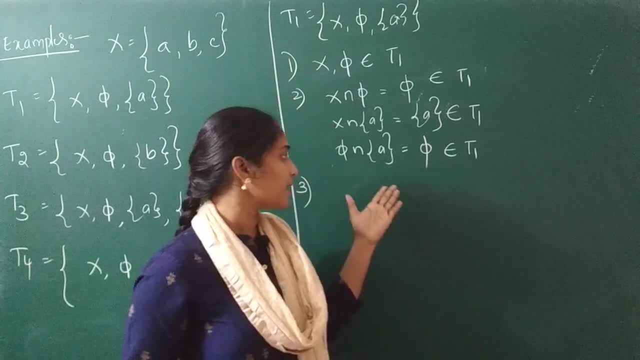 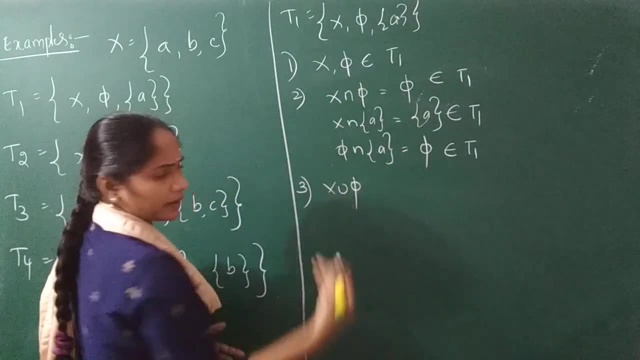 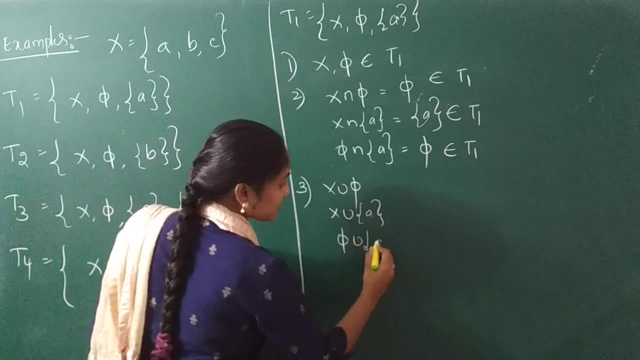 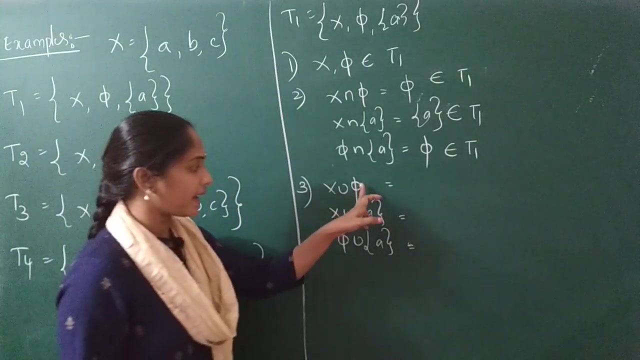 third condition: arbitrary union of same union. so please check, check that same same same. no, no here. intersection union, singleton set a. pi union, singleton set a. and next what is there? yes, these only three elements. now we are coming to the x. x is a universal set here, so you will. 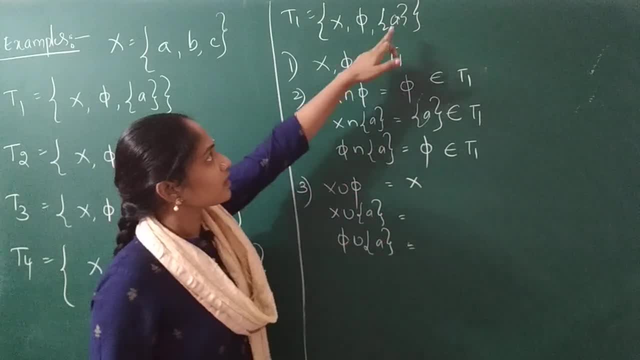 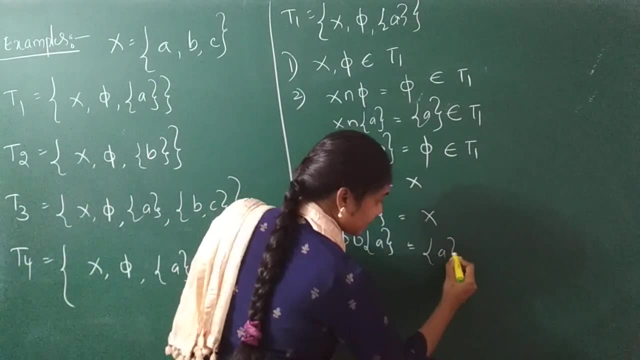 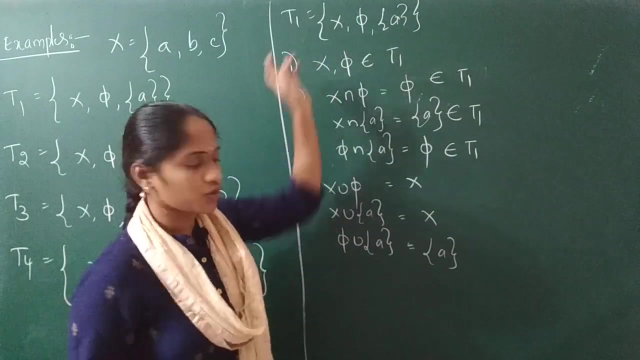 get in the x only singleton set a, a, another malia, excellent, only point: what you, what you have to write. this is x and pi union. pi is empty set, then the singleton set a will become a, a, x, x, which belongs to tau 1. singleton set a also belongs to tau 1, so their union is also. 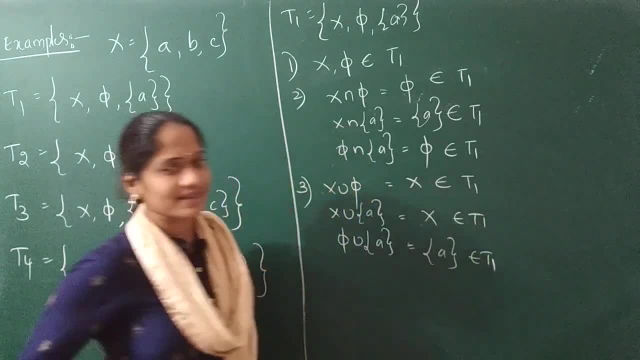 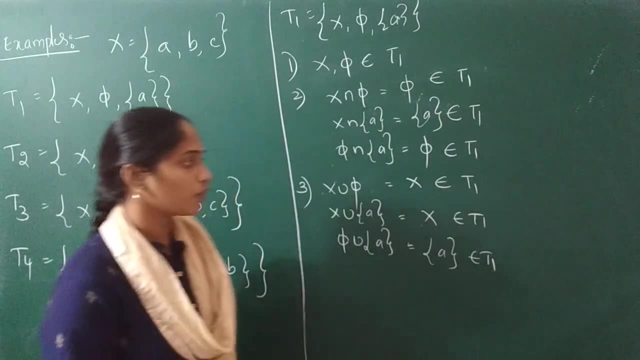 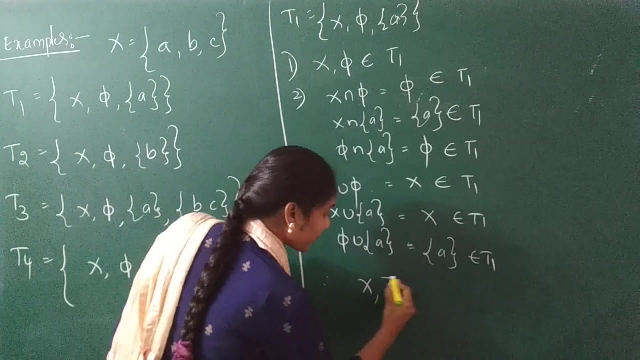 belongs to tau 1. yes, the arbitrary union of members of tau is again a member of tau. so what you can say? that the curve condition is also satisfied. then the algebraic structure x, equipped with tau 1, is a topological space. so in this way you have to. 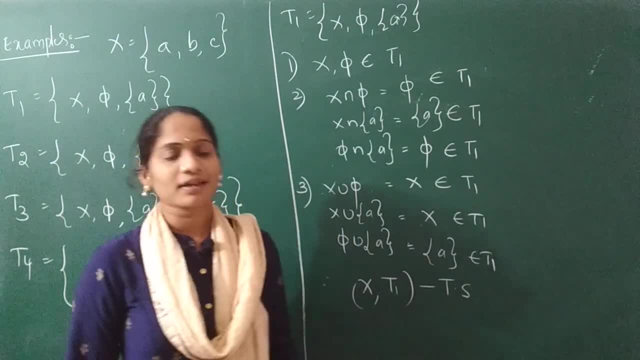 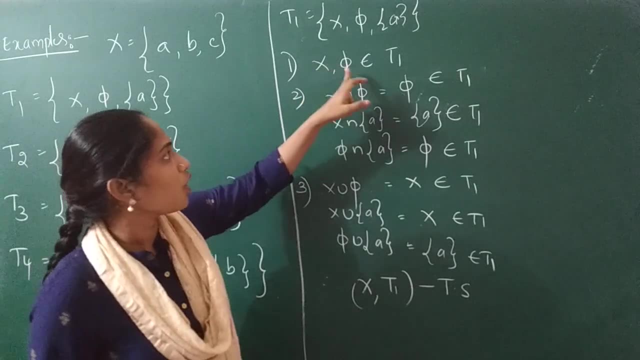 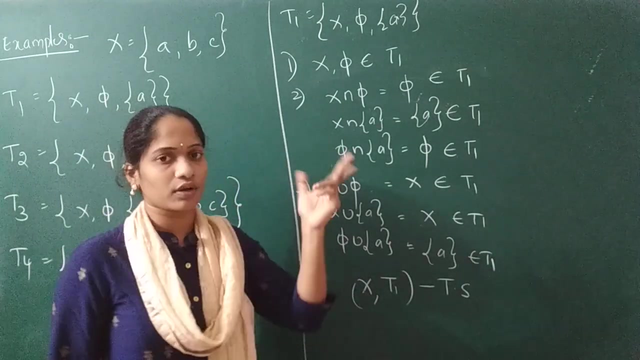 check out all these t force whether there are topology on X or not. what is the first condition? you have to check x comma pi. you can see here, you can know from x comma pi is in tau 1 or not. the second condition: A two, A set intervention is also in tau 1 again. 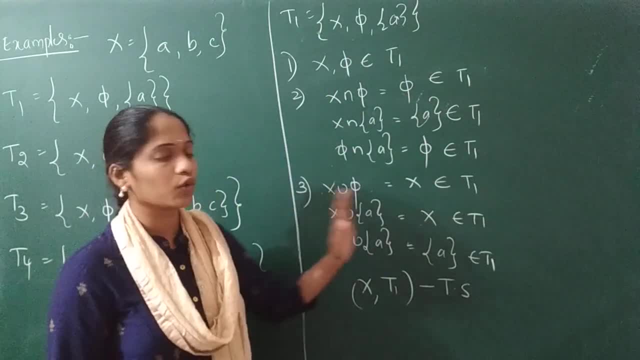 or not? third one is: what are these? union is also in tau 1 again or not. that is the finite intersection, arbitrary union. and at last you have, they are all הס. vegetable set is also in tau1 again or not. you have to check on this在p lasci Jerusalem here, this Pythagorean. 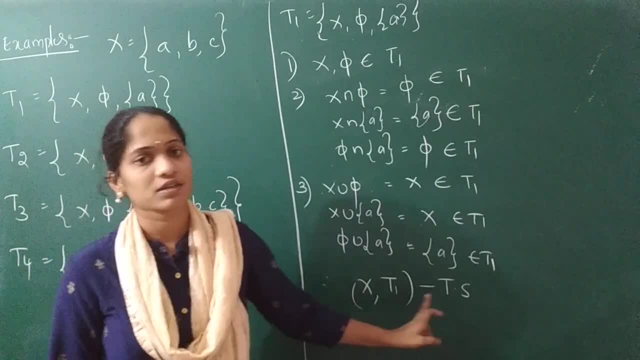 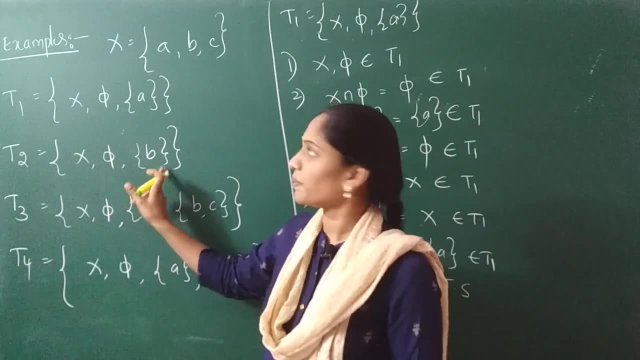 So what you have to say? the algebraic structure V, put with the T1, is a topological space. See the second example, tau 2. what is there? Same x, comma, pi and singleton set B. So same thing. in the, instead of A you can write B and you can check out all these conditions. 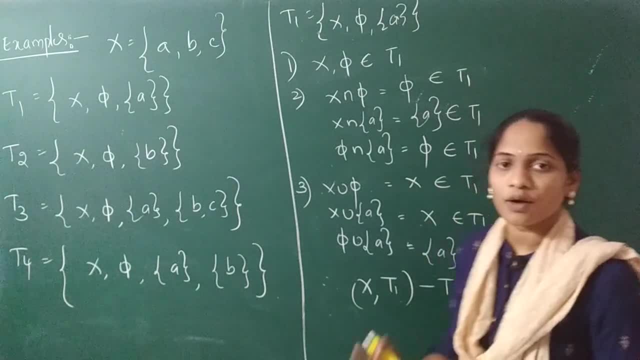 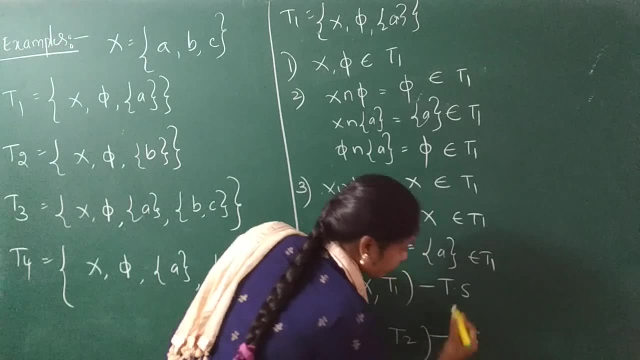 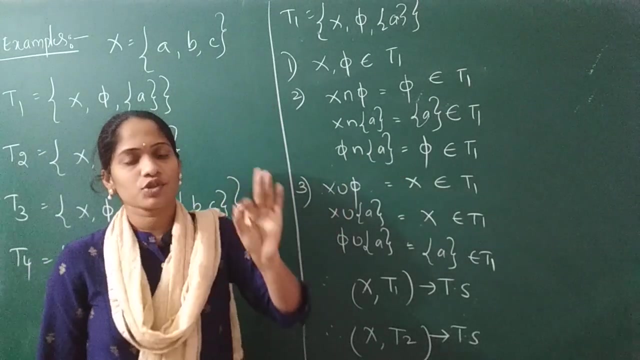 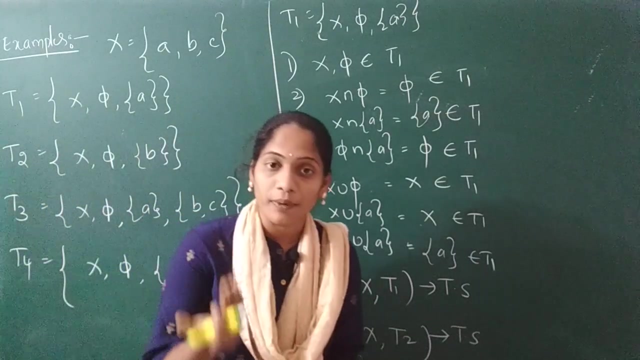 Then you can also conclude that x, put with the tau 2, is a topological space. Is a topological space? Same conditions, instead of the singleton set A, just you have to write the singleton set B. But coming to the third and fourth, whether they are topological space or not, you have to check out. 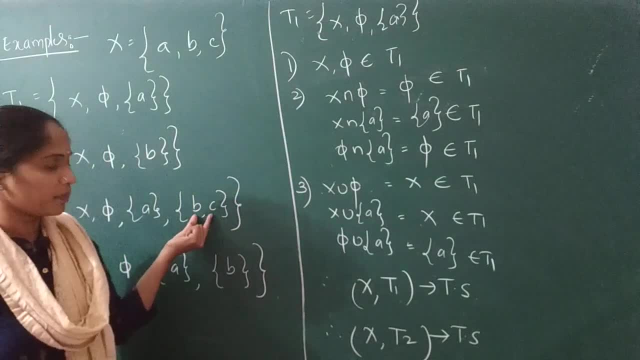 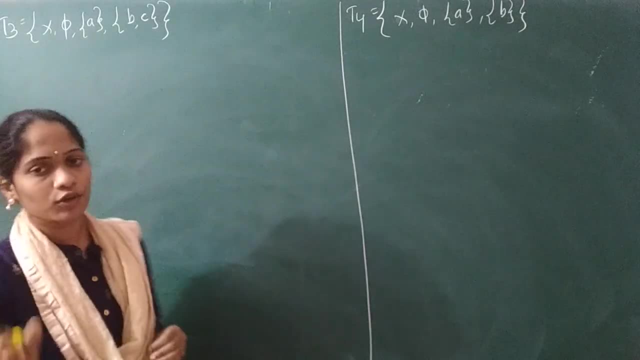 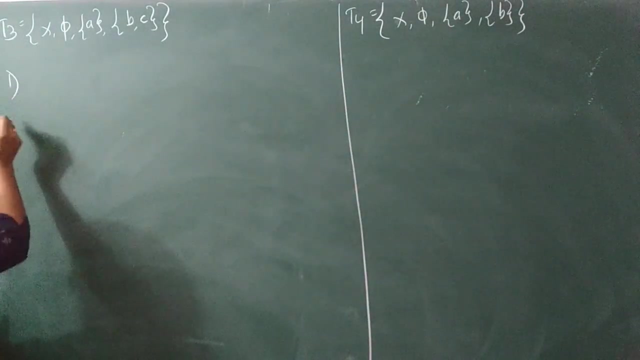 Because here you have, having the ordered pair V, comma, C. Let's see the third problem, Let us see tau 3.. So you may go through the, what is that? three conditions? So directly we can say that The first, What is the first condition. 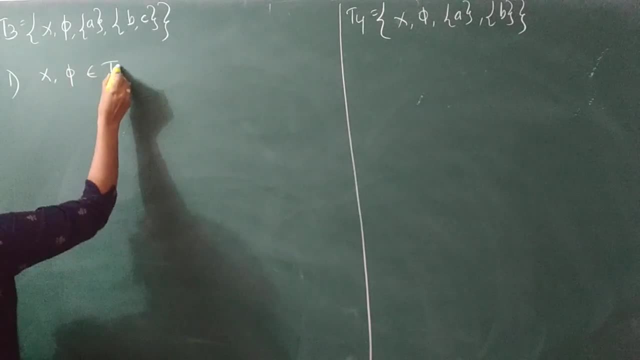 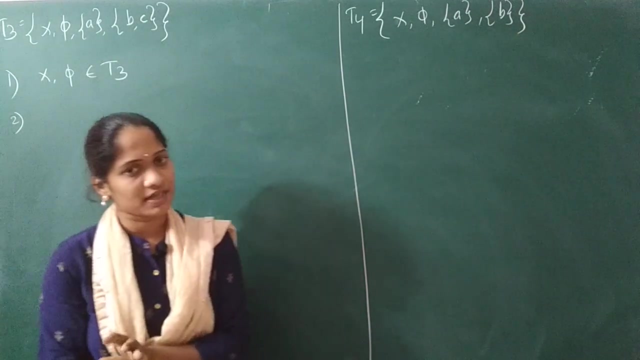 X comma pi. Yes, X comma pi R belongs to tau 3. First condition: If you go to the second condition. So here no need to do all by step by step. By observing these only you can directly say whether the second condition is satisfying or not. 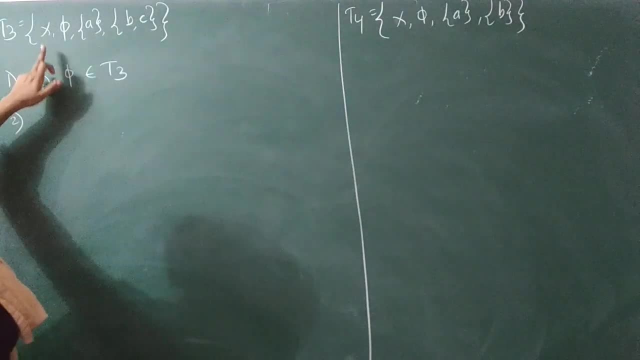 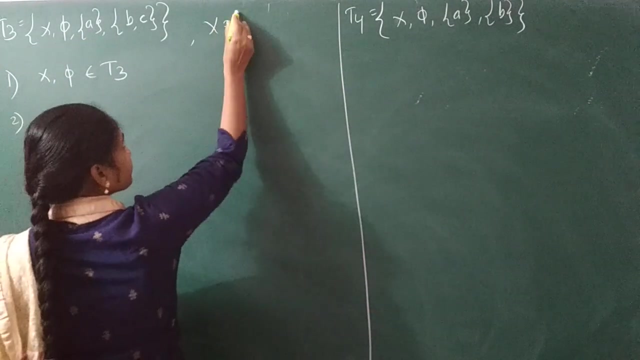 Because it is intersection, the common part. So now let's see: If you take this both intersection, it is pi. If you take this both intersection x, What is x here? A comma, b, comma, c is our x. If you take this both intersection, what is that? 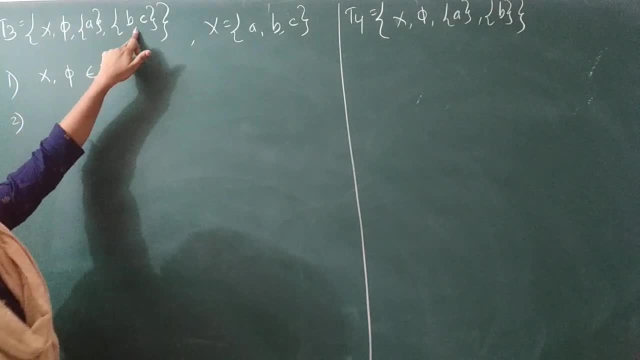 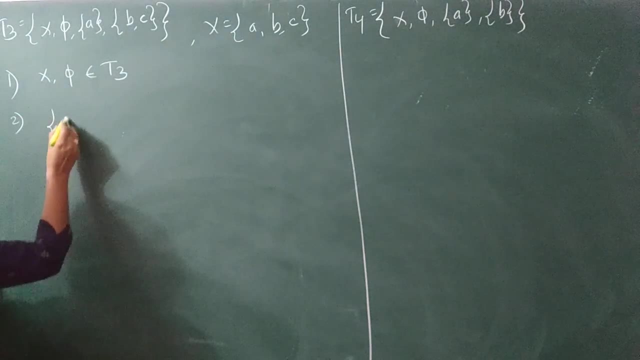 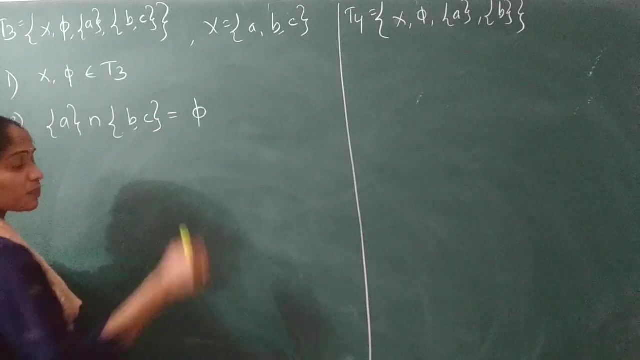 It will be a. If you take this both intersection, you can say b, comma, c. If you take this both intersection, there is no intersection path. Then what is it? If you take a intersection, b, comma, c, And what is that? Yes, the resultant set is pi. 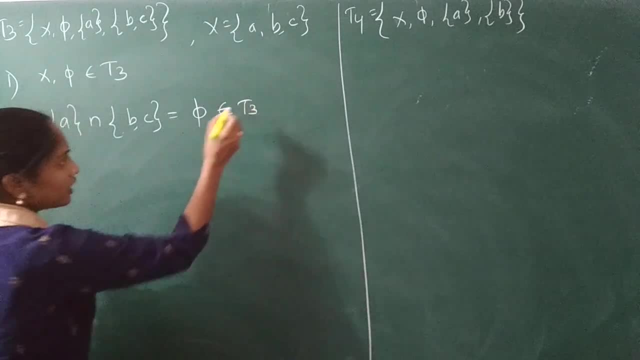 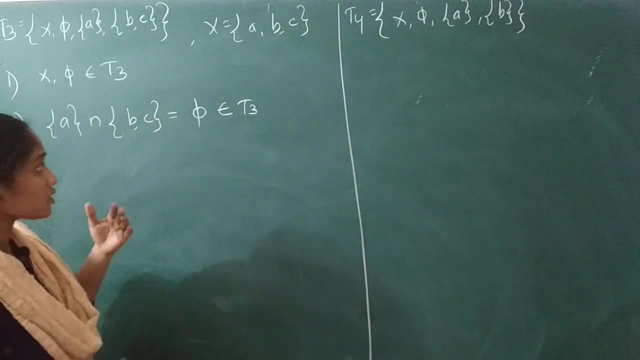 But pi again belongs to tau 3.. If you take any of two sets, If you do the intersection, The intersection is also resulting element. That is sorry. Set is also belongs to tau 3.. So what you can conclude? that the condition 2.. 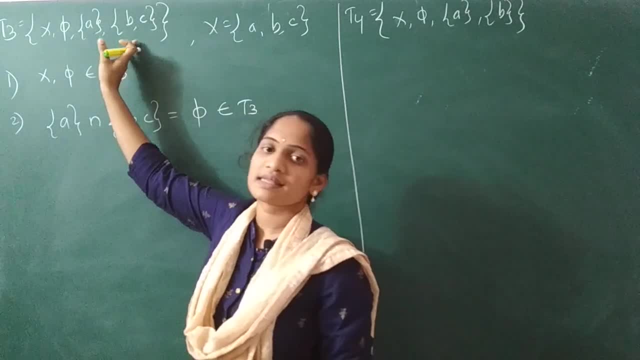 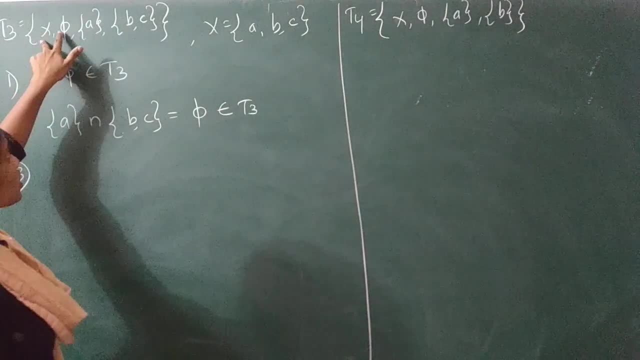 That is the finite intersection of member of tau. 3 is again a member of tau. So same here for applying the third is: If you take the union, If you take this both union, it is x. If you take this both, it is also x. 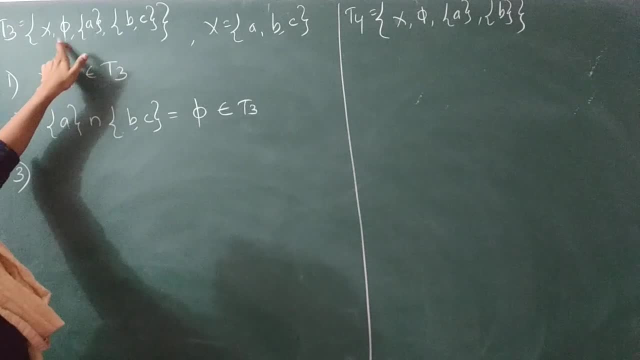 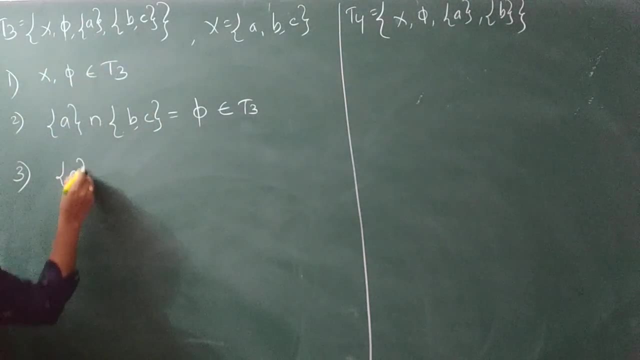 If you take, this is with both. this is also x. If you take the union of this, both things, It is a and b comma c. Right, But whenever, coming to here, this, A union, b comma c. And what is that? A comma, b comma c. 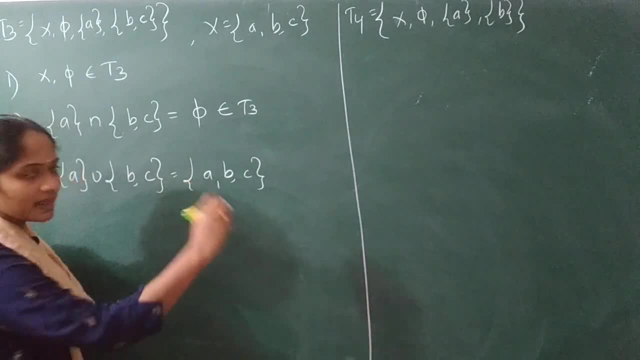 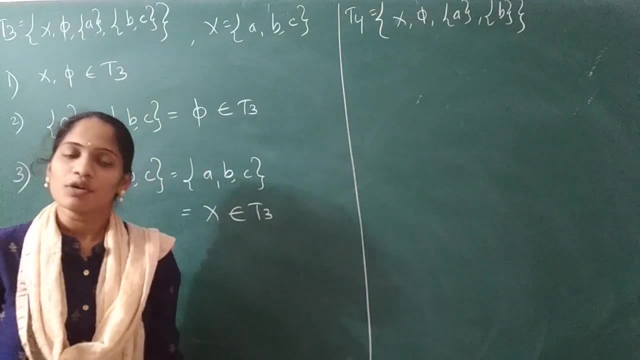 What is a? comma b, comma c? Yes, What is that? Our non-empty set x, which is again belongs to tau 3.. So in this way you have to do the conditions Right. So here what you can conclude: that 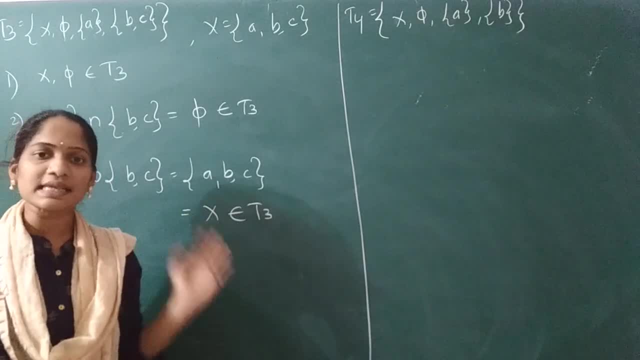 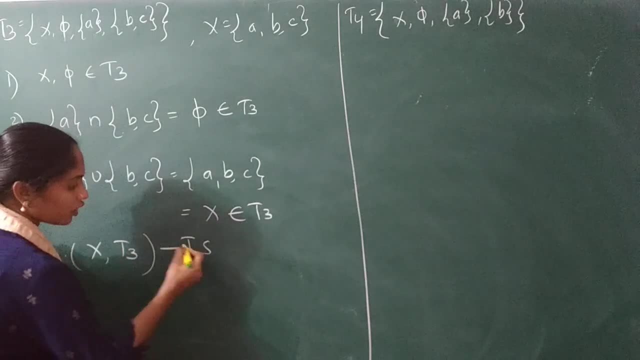 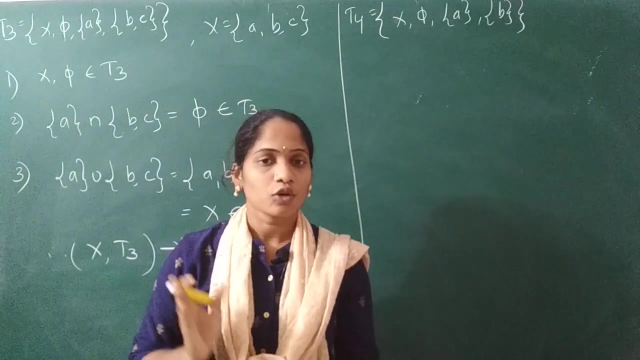 Orbiter union of members Of tau 3 is again a member of tau 3.. So our conclusion: algebraic structure is a topological space. So in this way you have to do given topology, Given set is topology on x or non. 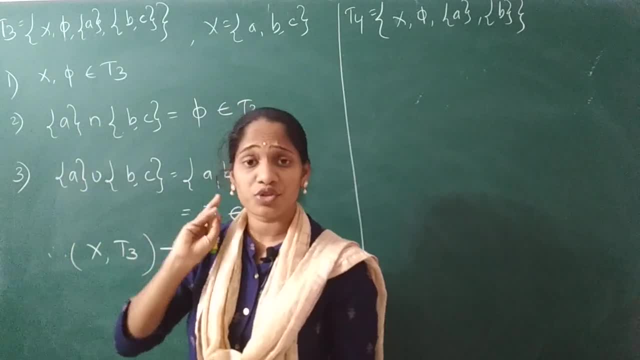 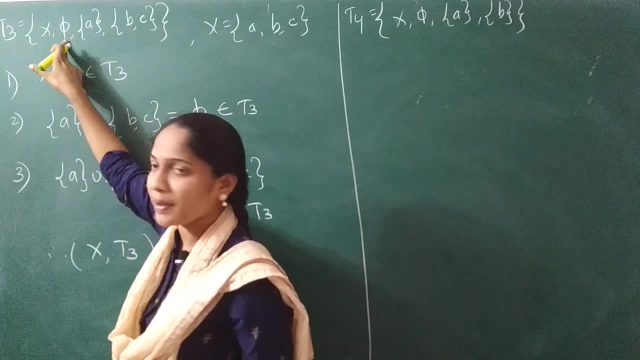 By checking the three conditions carefully. You have to check for each and every two sets. You have to do for these two, These two and these two, And you have to take pi And you have to do these two And you have to do these two. 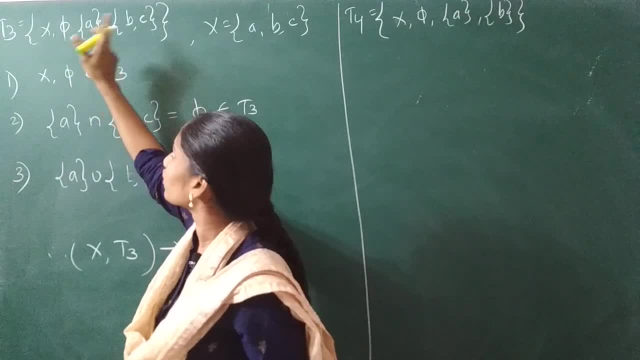 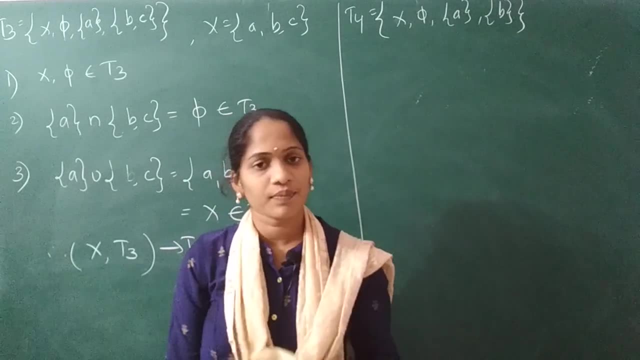 And these two Intersection. If you take this set And you have to do intersection with For each and every two elements, Two sets, You have to check the intersection And also same the union. So now come to t4.. 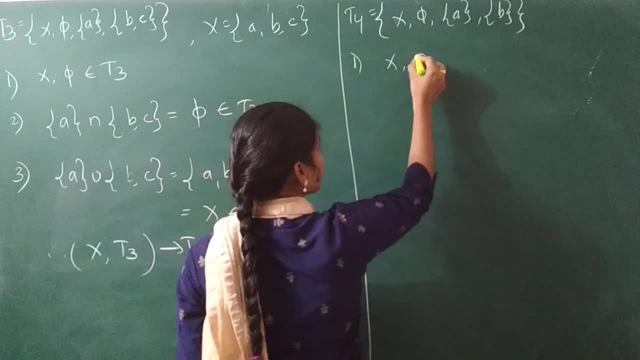 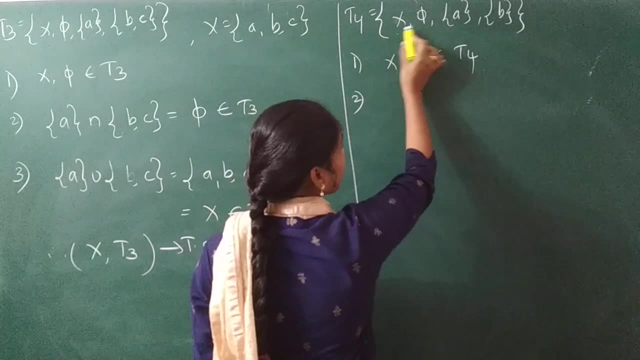 We will check. Yes, The first condition is x comma pi Belongs to tau 4.. It is clear And come into the second condition. If you take these two And these two here, This is intersection. This is a. 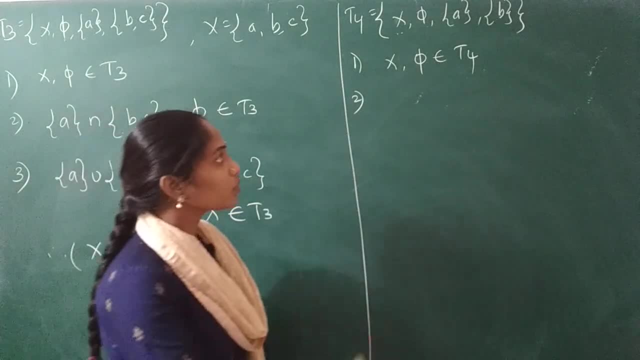 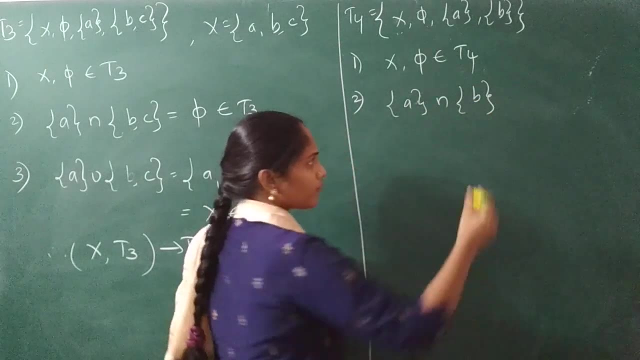 And these two intersection. This is b? Yes, It is clear, It is clear. Well, Coming to the intersection of these two Intersection this, Is there any common? No, And what is the resultant set? Pi, And pi belongs to t4.. 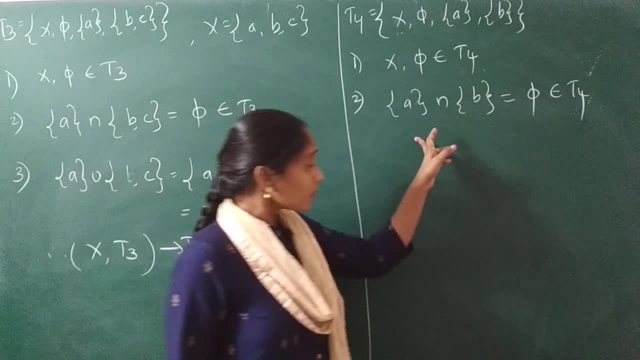 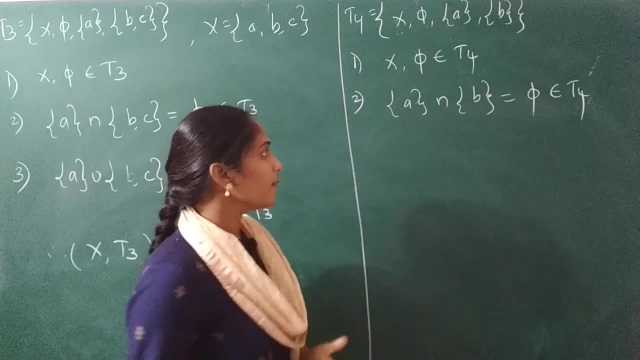 Yes, The intersection is also Is also satisfying. the second property, That is, Finite intersection of members of tau, Is again a member of tau. Let's go to the third condition. So same Check for two sets Union Union. 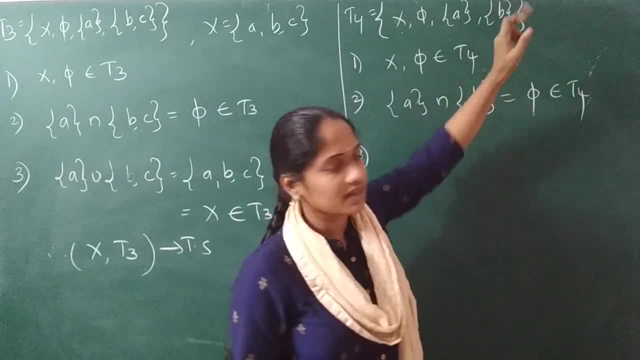 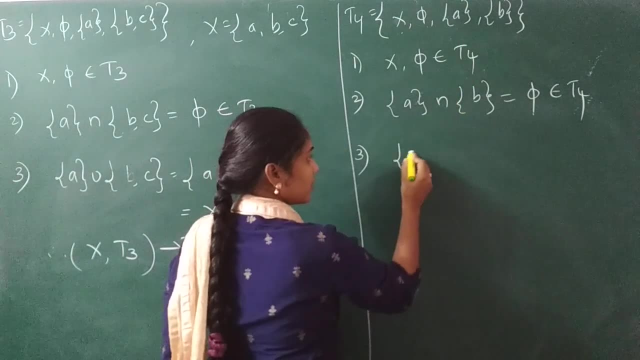 It is x. If you take the union, It is x. If you take this, both unions, It is x. Coming to the pi. This a Coming to the pi union, It is b, But coming to these two Sets. 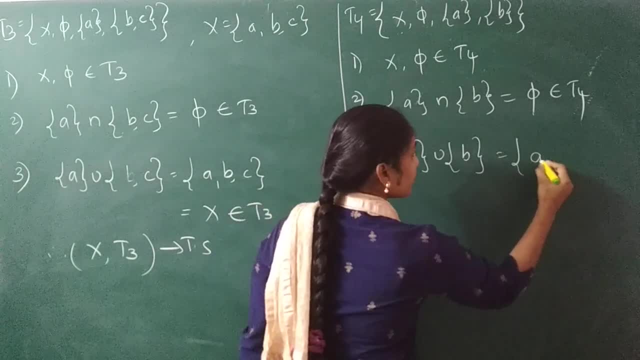 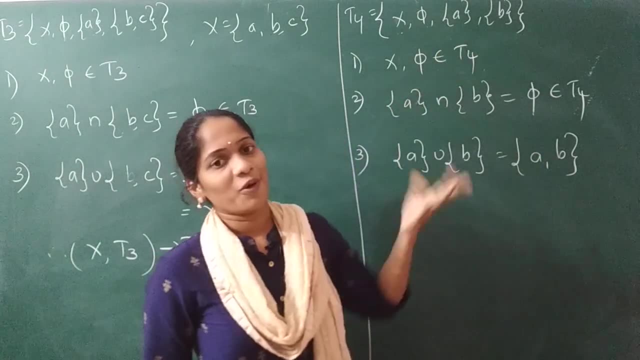 Union. And what is the resultant? A comma b And go to that A comma b. Whether a comma b is in tau 4? No Here. That's why I have Written the two, Two examples to compare here. 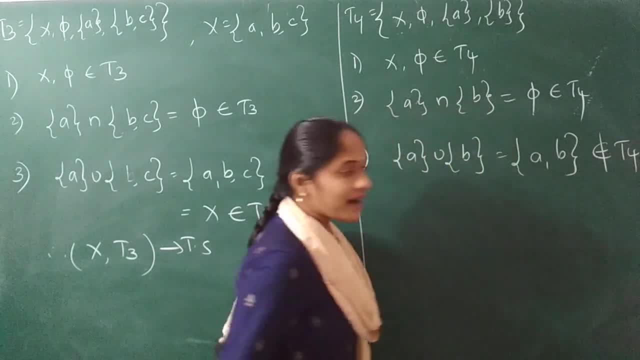 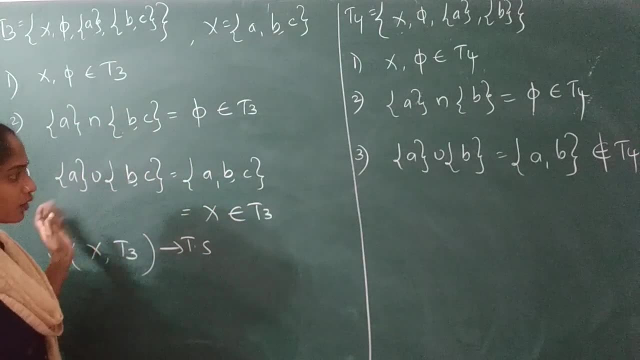 So which does not belongs to t4. But You have written: This is belongs to t3. See here, When you are doing The union, You got here A comma b comma c. Yes, I agree with you. 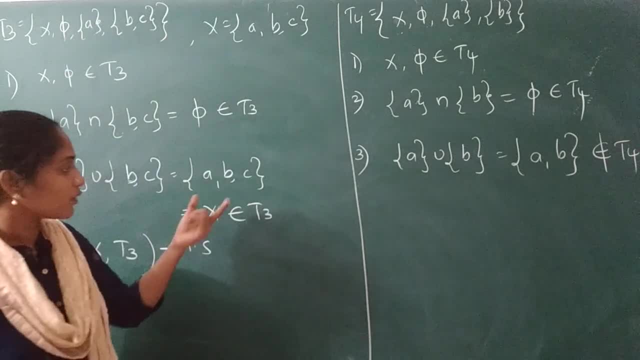 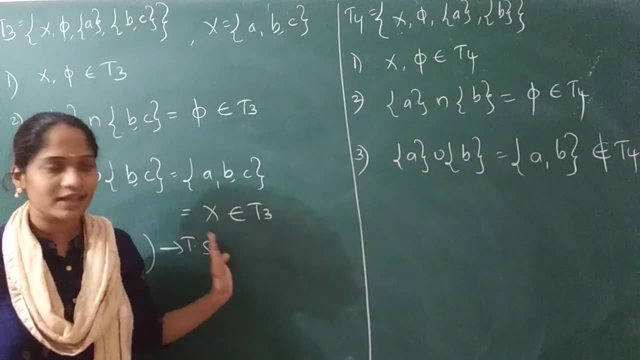 A comma b, comma c is not there in tau 3.. But what is a comma b, comma c? X And x is in tau 3.. In this way I have told you that x belongs to tau 3.. But a comma b, comma c. 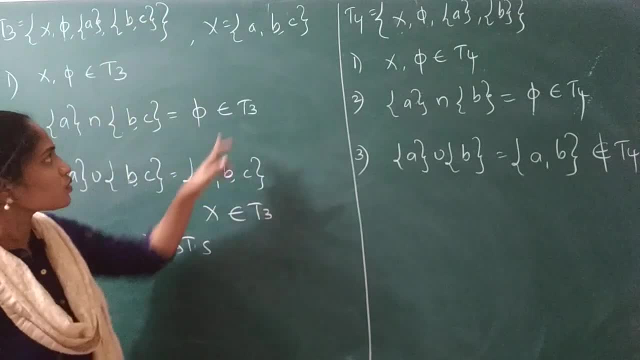 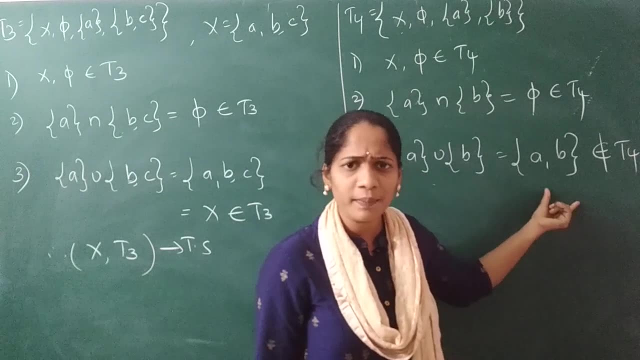 This set is not there in tau 3.. But this set is nothing but what X. But here, Same Same procedure When you are coming to the union. A comma b Here. a comma b is not there in tau 4.. 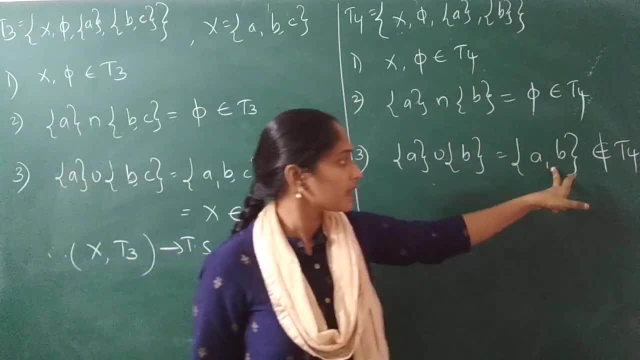 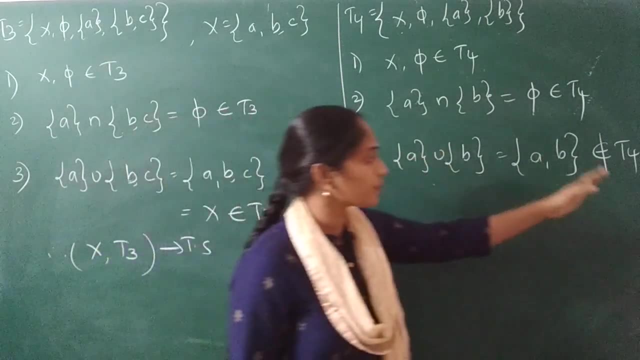 And a comma b is not also x. So what? you can say? that A comma b does not belongs to t4.. The third condition: What is that Orbiter union of Members of t4 is again not a member of t4.. 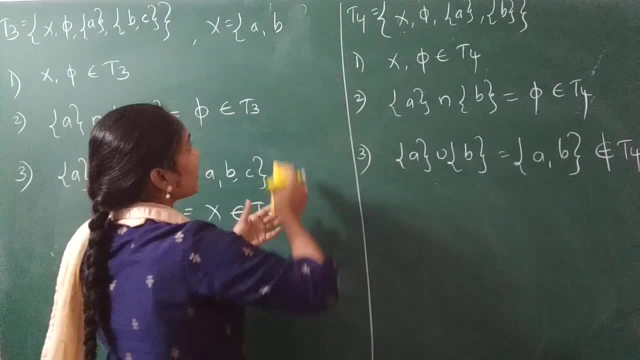 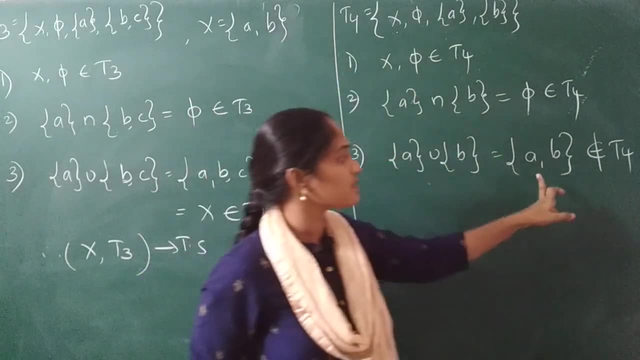 If, If in case The x is only a comma b, If in case The x is not a A comma b, A comma b, Then you can say that A comma b Is equal to x And x is a member of t4.. 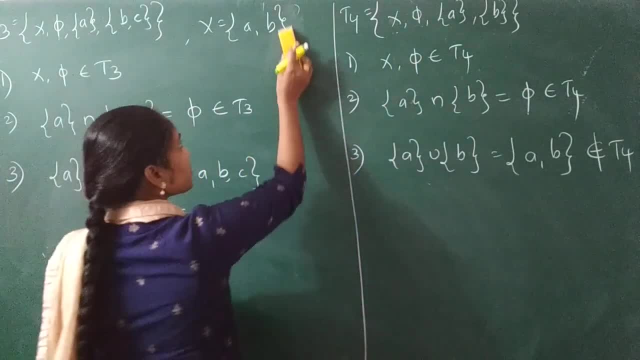 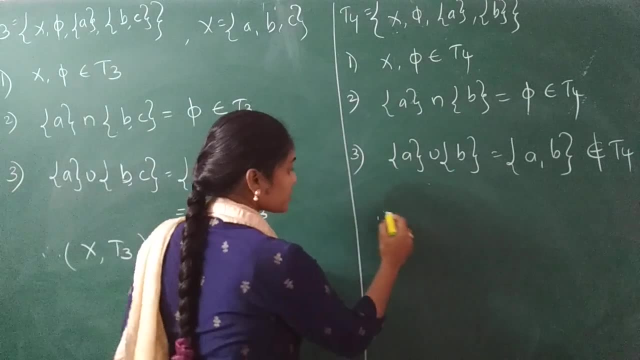 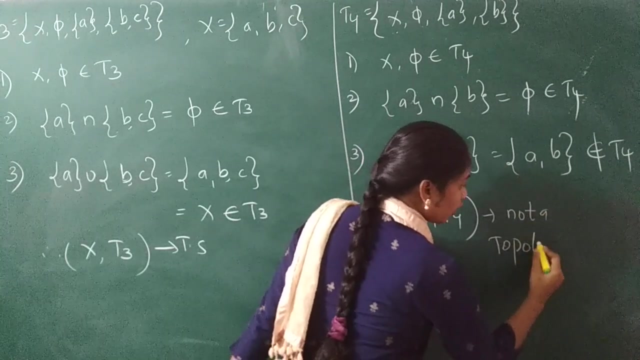 And this is nothing but a topology. But coming to here, Our x is A, comma b, comma c. This does not belongs to t4. Then the conclusion is X. X We put with t4. Is not a Topological space. 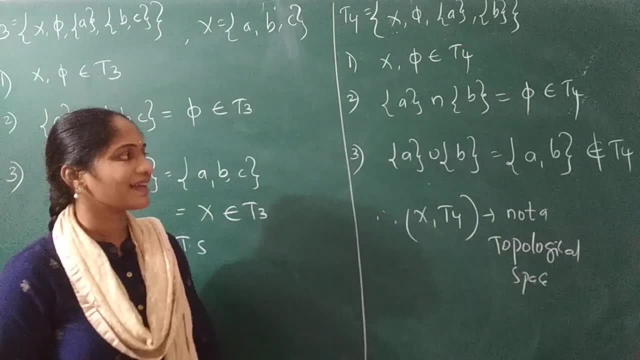 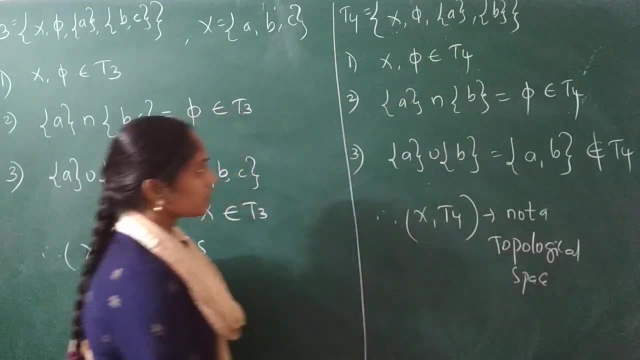 Is clear for you. You have to check the elements, The sets, Just whether they belongs to that given topology or not. Now, So these are some examples. I think this is clear for you. Let's see the another definition. Let's see: 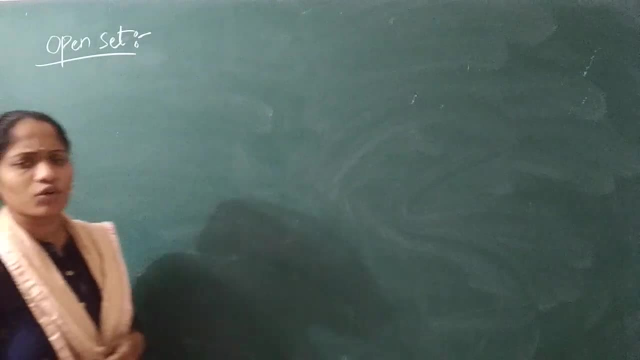 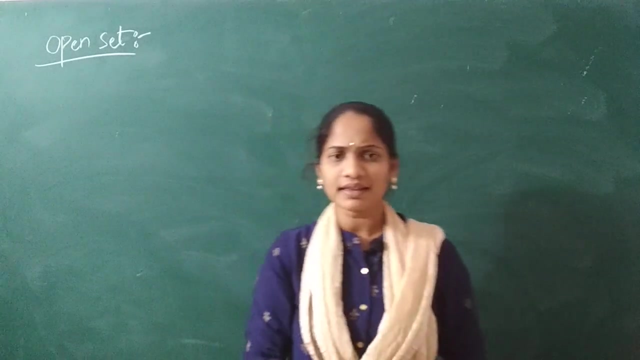 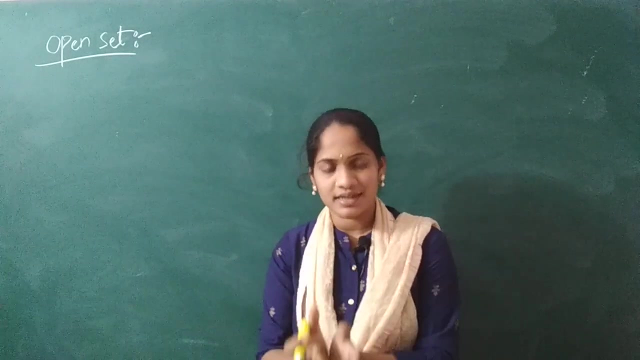 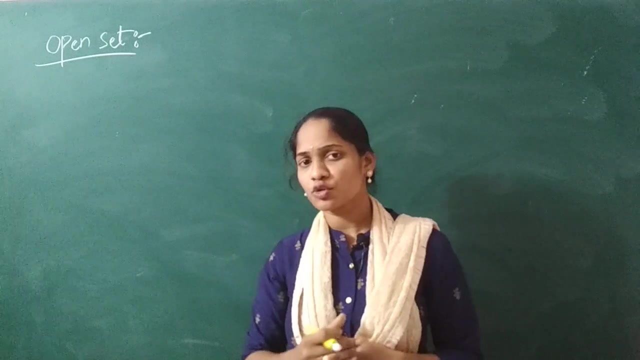 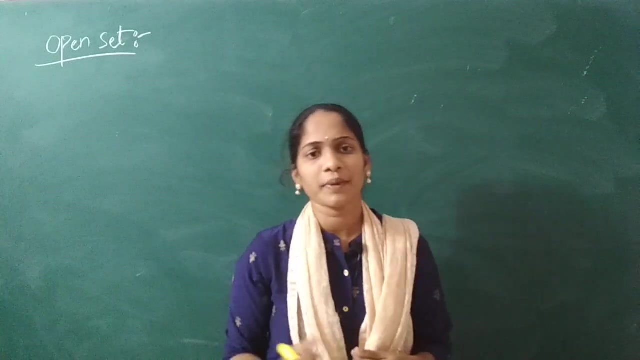 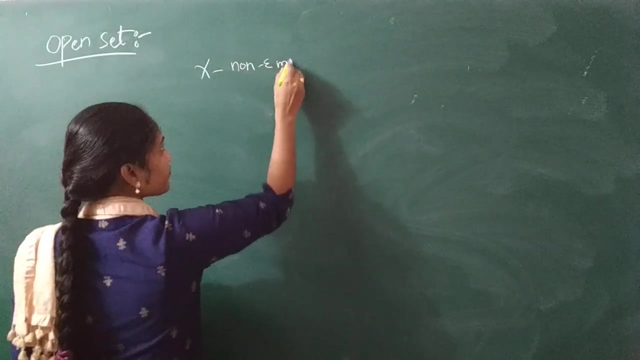 Let's Let us discuss the another definition: Open set. You know, open set definition, Right, Open set. It is so simple Because, Just, I think, in metric space, Okay, In metric space law, You have to, You have to consider the neighborhood and you have to say that if x belongs to g and g is, g is an interior point, g is a subset of a and the metric space logo and kuchu is the mic open set definition. concham, different down to me and I mean I would create jdangani and the at log, just to me. but here it is so simple because here what is x? x is any non empty set, right, x is any non empty set, and now it is in a topology. 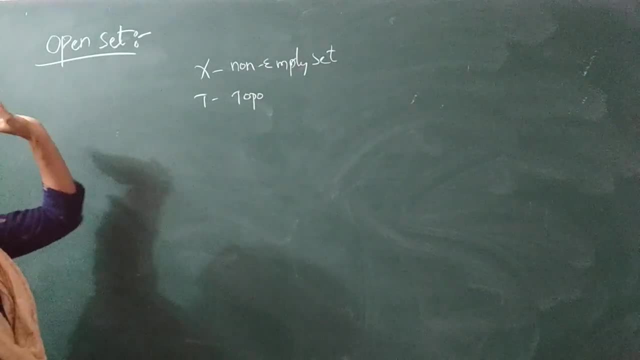 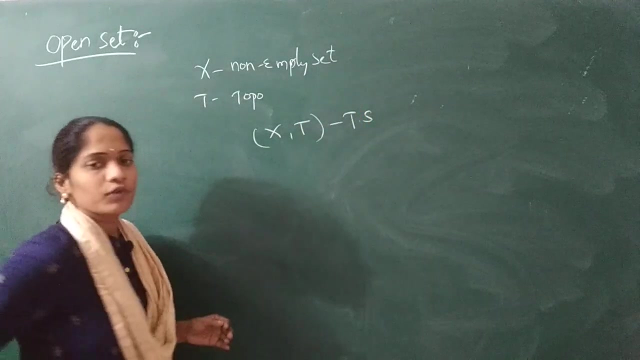 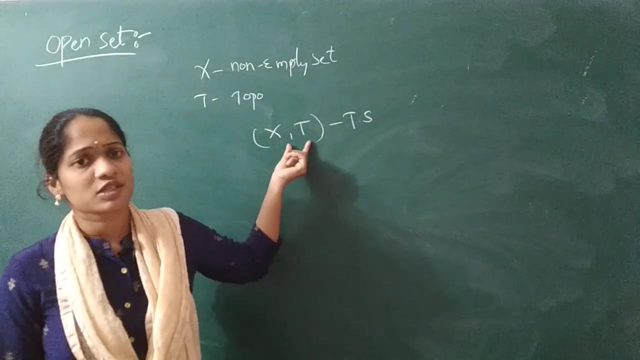 Right, So not topology Here. Coming to the definition open set, You have to consider x comma tau should be a topological space, Got it? So you are here: x comma tau topological space, If you consider this topological space. 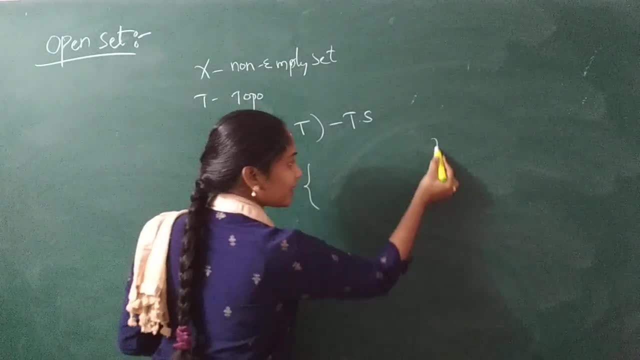 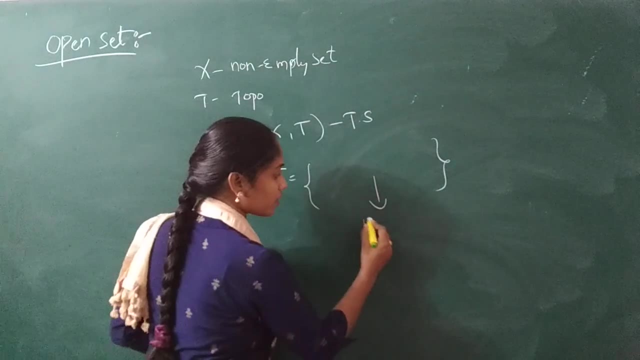 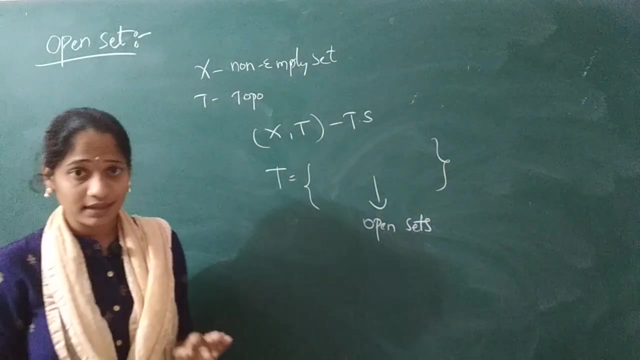 Then the members Got it. What you are written in the flower braces of tau. The members of tau are known as the open sets. These are all known As the open sets and the members of x are known as the points. Is that clear for you? 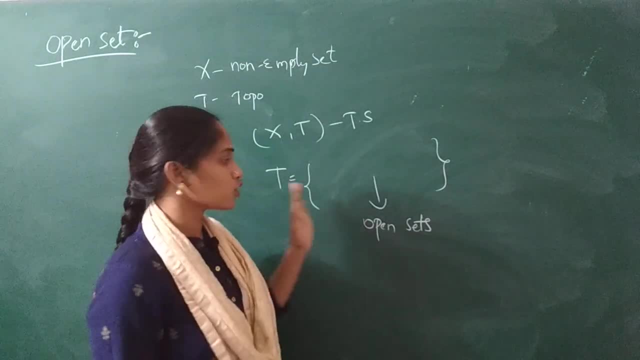 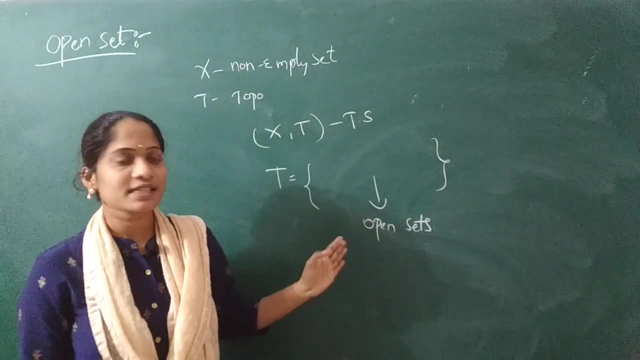 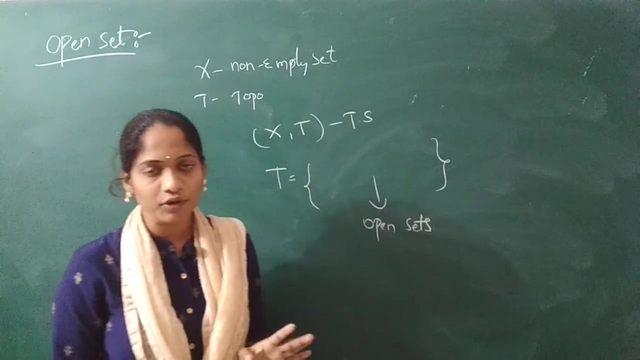 So simple. Yeah, Wait a second. Your topology, low topology, Normally topology. Let me just come down. So our subsets are the open sets. I got it And that is a very important You have to remember when you, when you consider x comma, tau, to be topological space only. 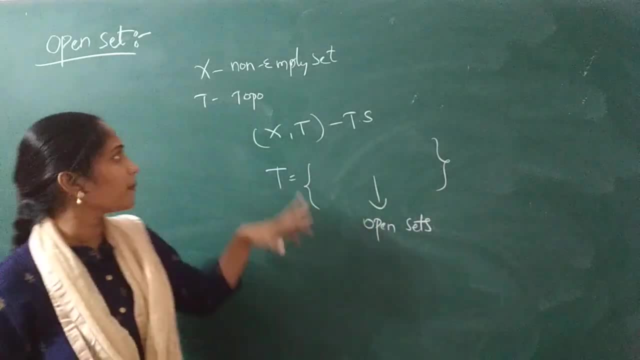 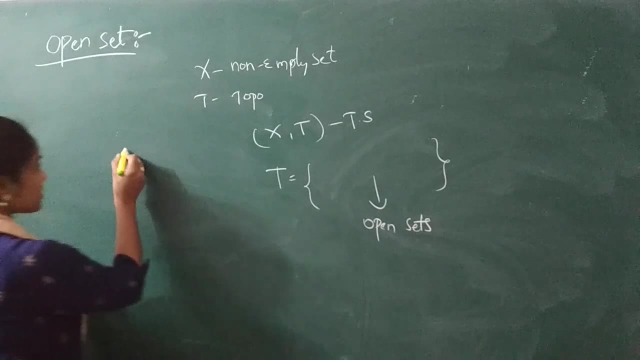 Then the members of tau are known as the open sets and the members of x are known as the points Right. Let us small example means nothing, The previous example. Let us see that. What is x? We are consider a comma, b, comma, c. 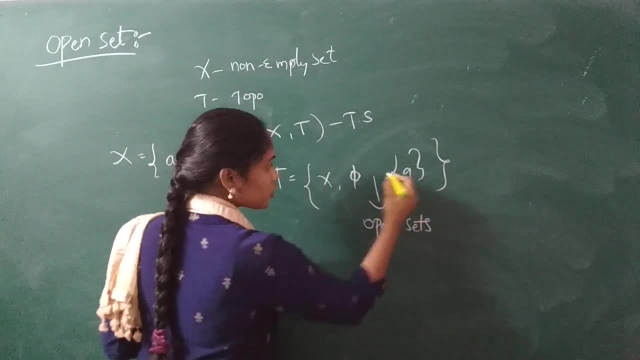 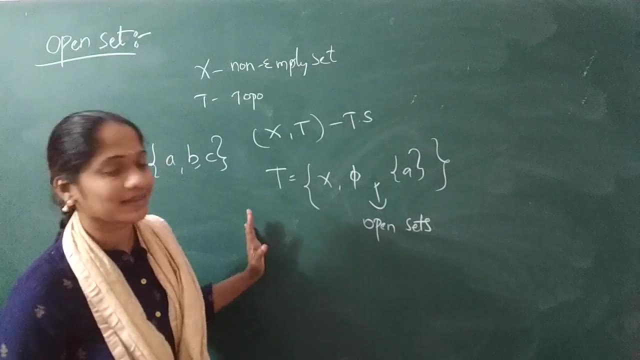 I have taken some. Let us take the single term set a. So here these are our first of all, These are the subsets of x. When you prove the clarify, that is the three conditions, and then we do our three conditions Prove. 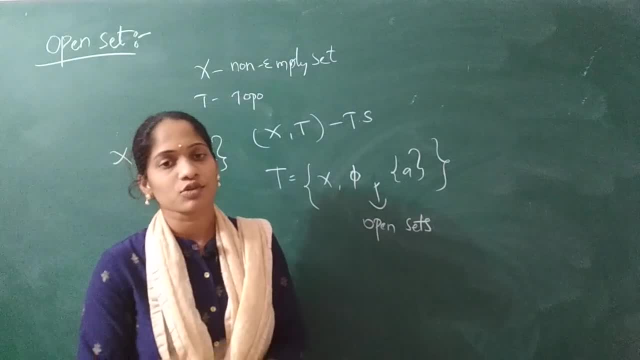 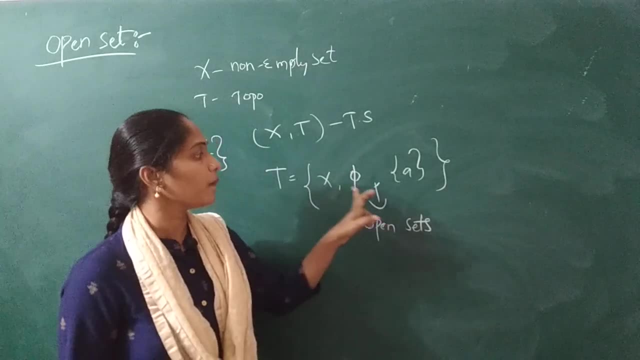 After that, this is the topological space. So then all the elements in the topological space are open sets. Now, open sets are x, pi, singleton, set a. These are all open sets, So same compared to that closed set. 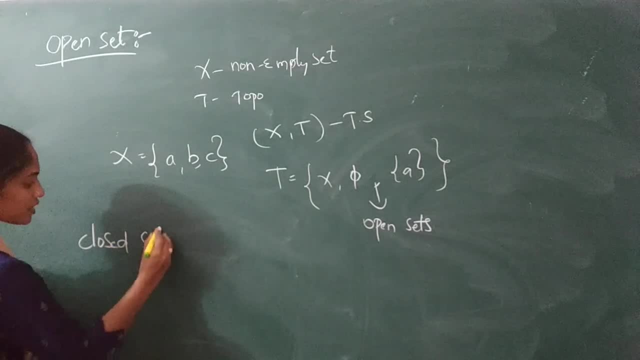 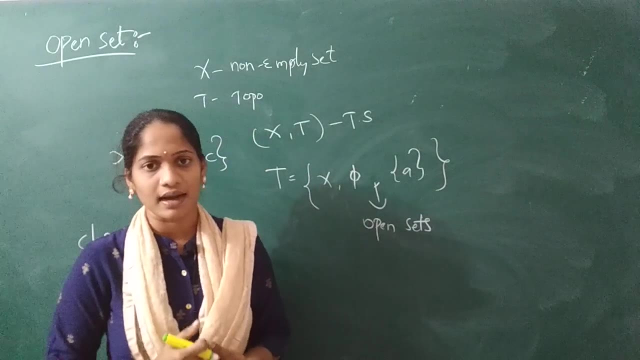 See how the open set is, So the same closed set will also be there. The matrix space has a very close connection to it, But there it is still theoretical and diagrammatical. But there it is still theoretical and diagrammatical. 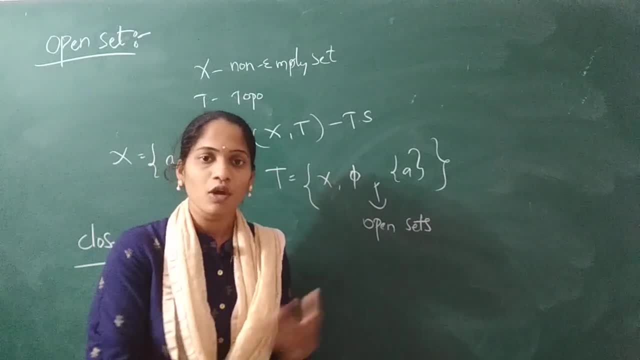 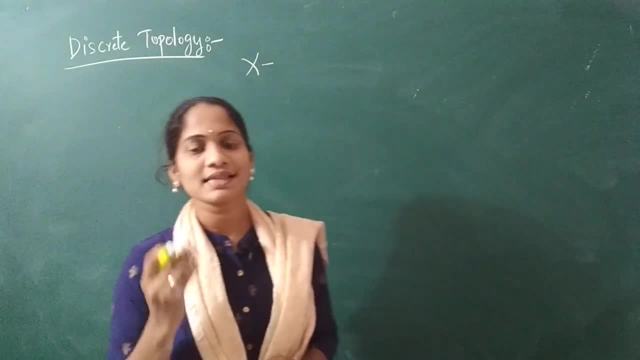 So what we are saying about the open set is that we are saying about the closed set. So what we are saying about the open set is that we are saying about the closed set x. what is that? any non-empty set. and next, you have to consider tau. what is tau? you have to. 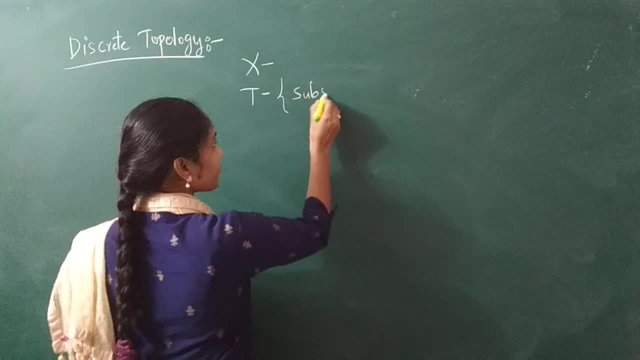 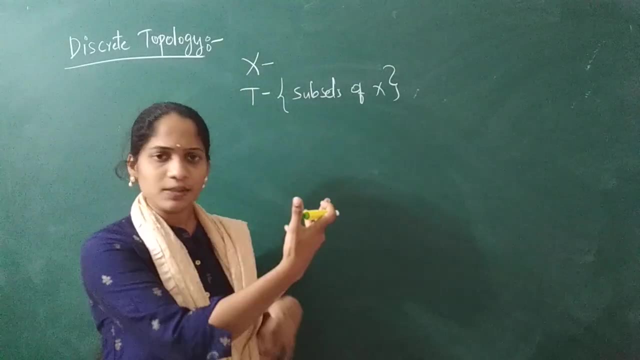 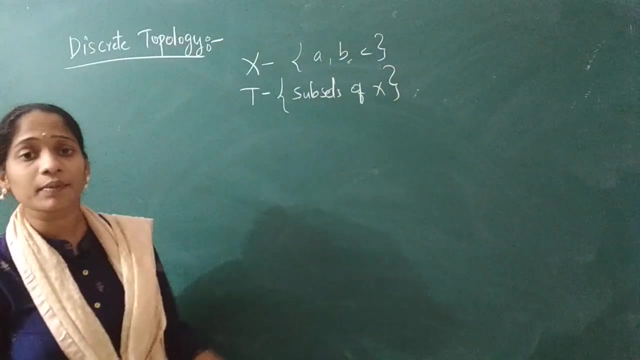 remember always what is that? subsets of x. so here you are considering tau to some subsets of x. if you take x b, any a comma b, comma c, so that means subsets a, but in that case we have written just only singleton set a or only singleton set b or a comma b like that. but 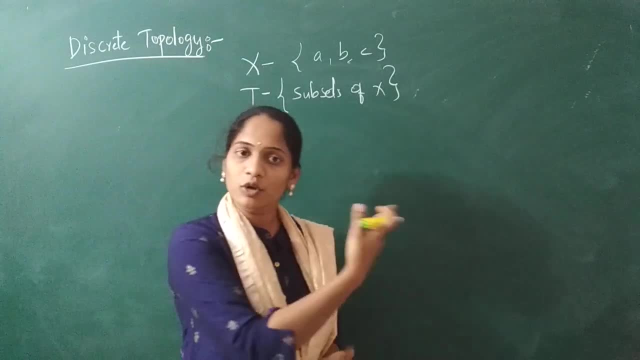 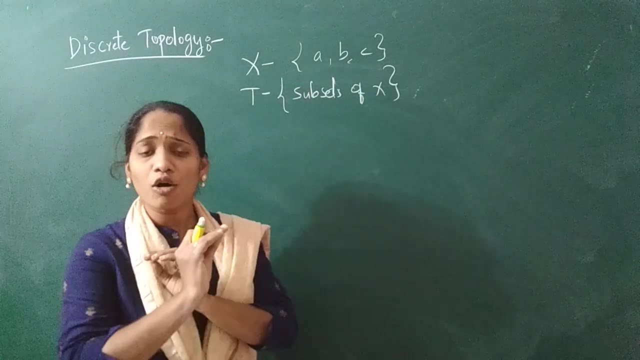 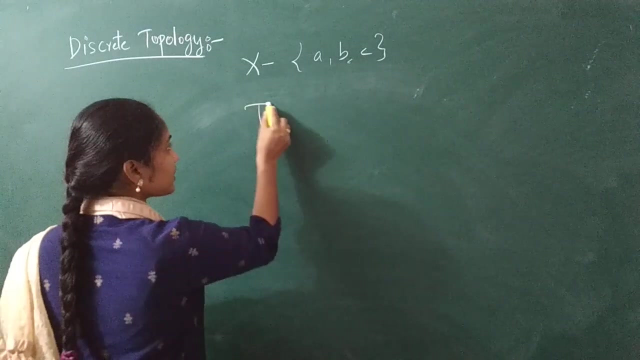 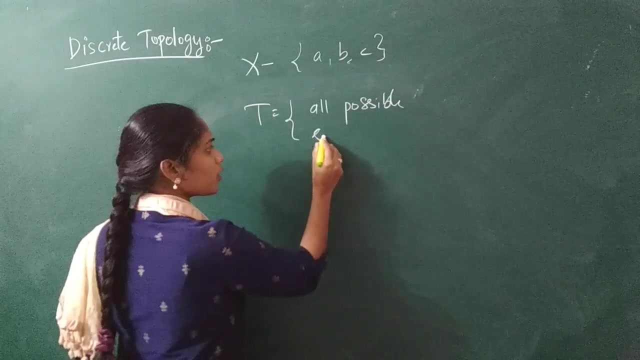 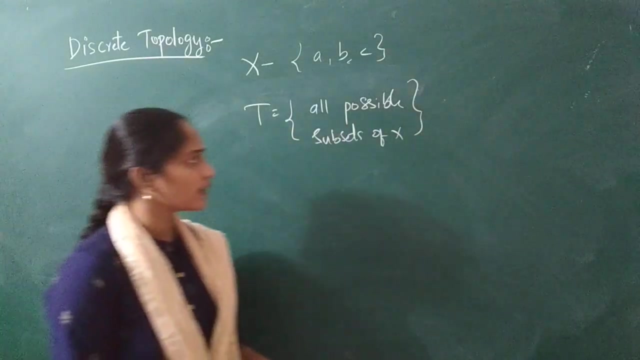 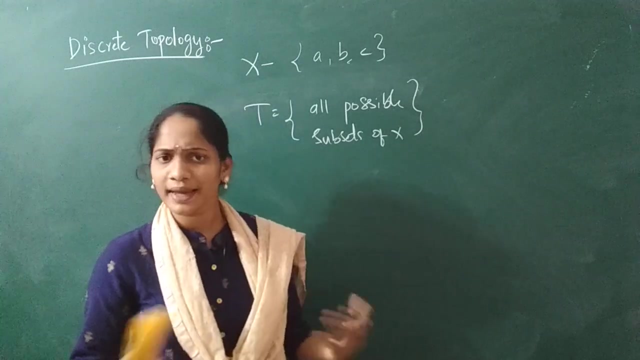 but here discrete topology means all possible subsets. you got it here when you, coming to the discrete topology, that tau should consider all, all possible, all possible subsets of x. got it here when you consider only only some, just only one to two subsets. maybe it may be satisfies the topology or may not. so it is none of the matter. but if you consider 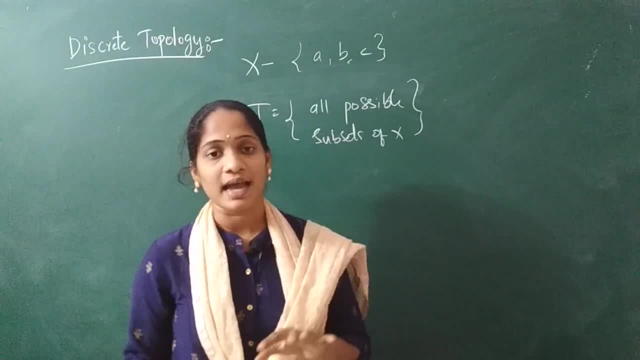 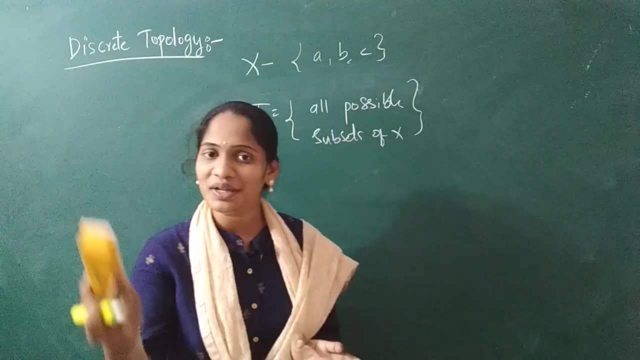 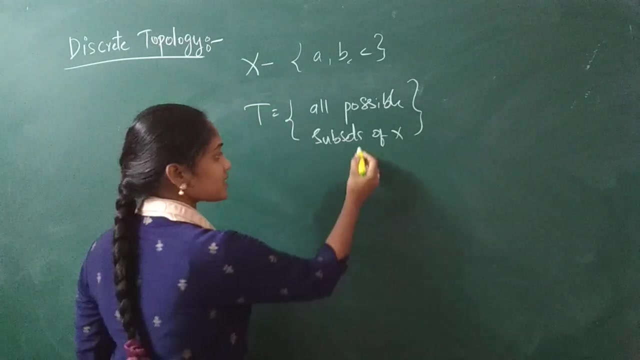 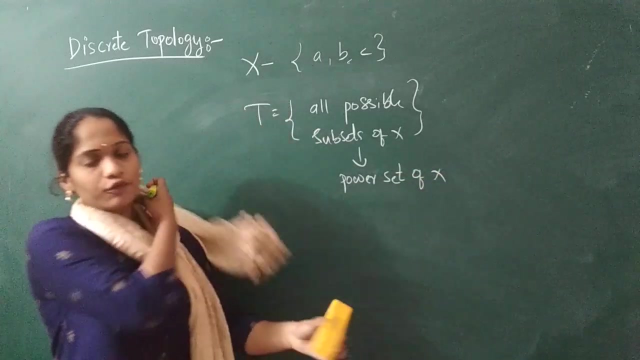 all possible subsets of x and that all possible subsets of x, and that tau is known as a discrete topology, or simply you can say that all possible subsets. what is the simple definition- yes, power set of x- and what you can say that what is this power set of x if you consider all possible? 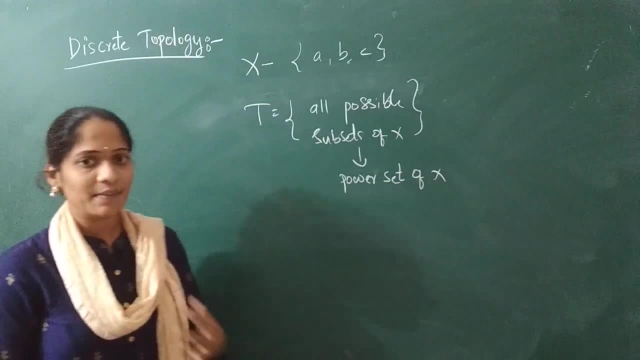 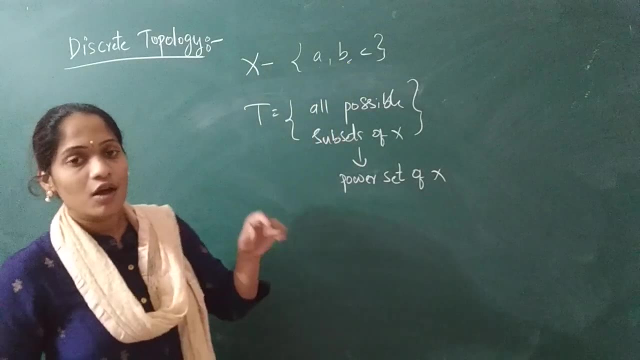 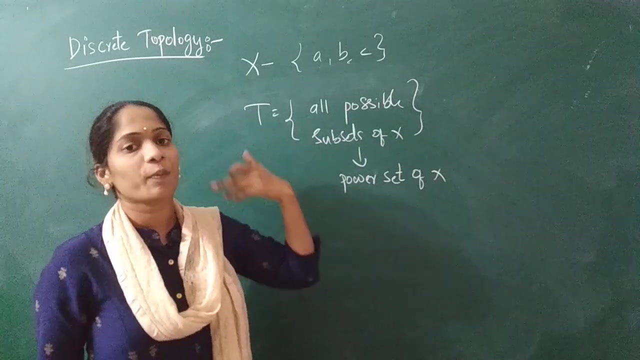 subset, or simply you can say that power set. let us see example, it will be clear for you see. so same here. you have taken x, c, a, comma b, comma c. so how many elements already we have discussed. now the members of these are no points and the members of tau are known as the open sets, if you consider. 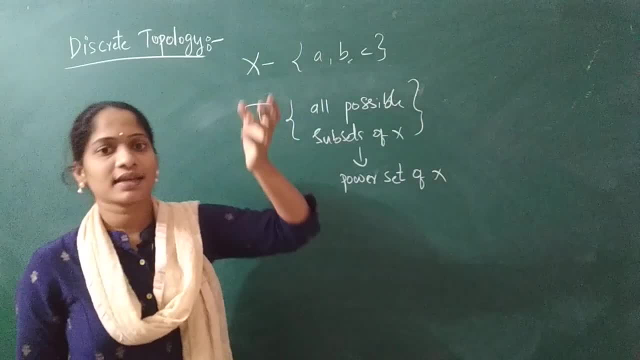 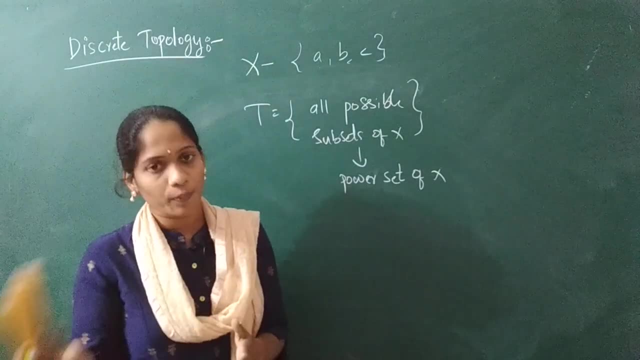 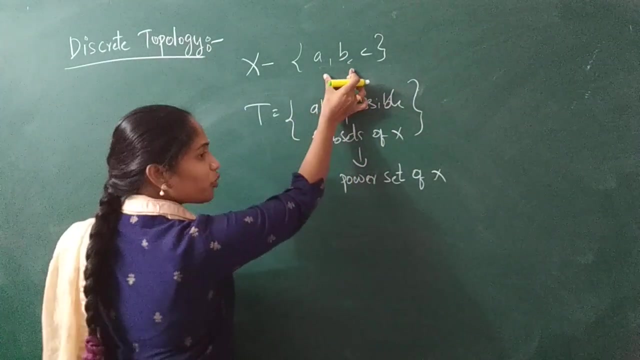 these points? how many points are there? that is members you can say. you can say members, elements or points, but if you consider x, that is x comma topology, then that x is the points and tau is the open sets. considering so these elements, how many elements are there? three elements compared to the. 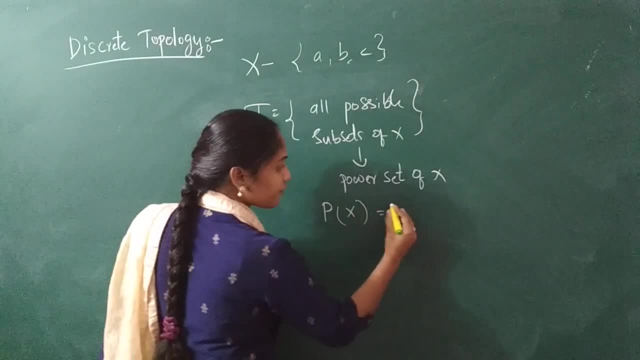 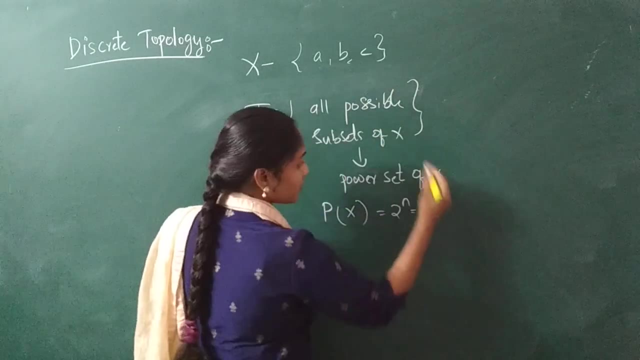 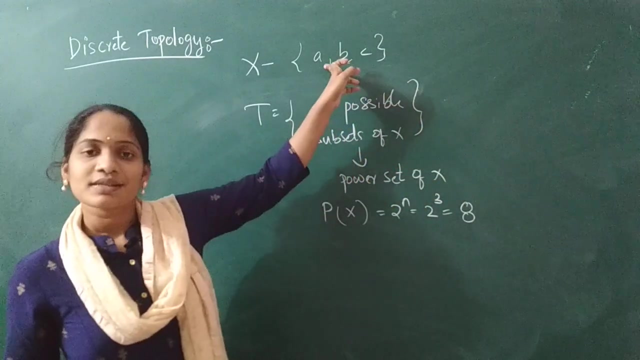 power set definition, that is p of x. what is the definition? yes, two power n, n is number. that is opposed to integer. how many are there? two? that is three. is there three cube? that is yet now. how many possible subsets should you will get yet possible for this set x, and that set is known as the discrete. 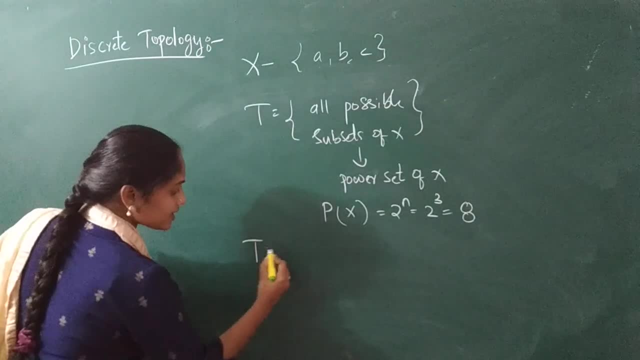 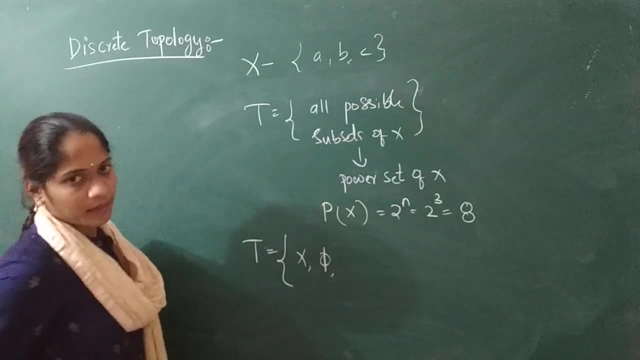 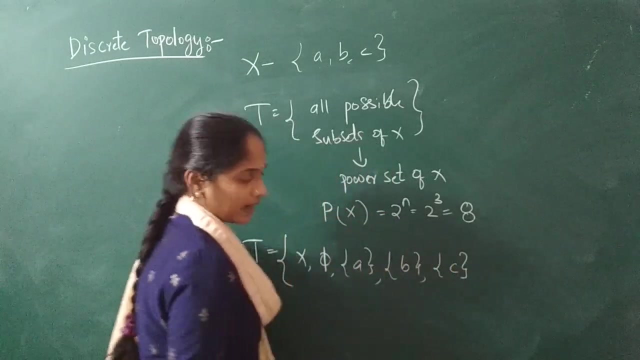 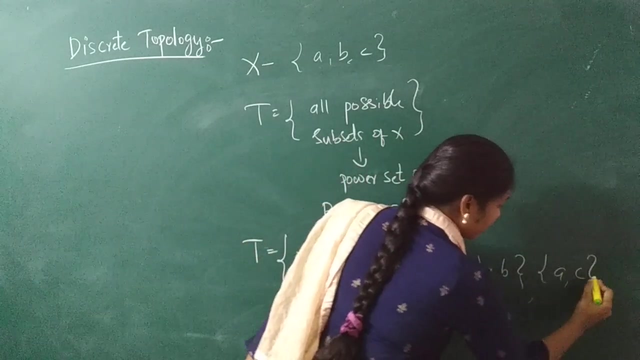 topology. so let us consider the subsets here, and i make eight subsets also: x is the uh compulsory, x comma pi. and let us take the singleton set a, singleton set b, singleton set c, and next they take the ordered pair: a comma b, a comma b, a comma a comma b and a comma c. next is b comma c. how many? 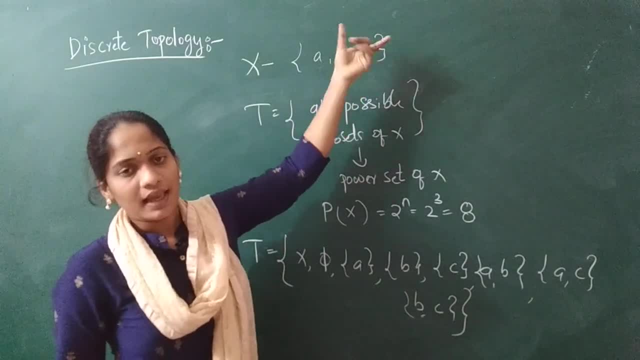 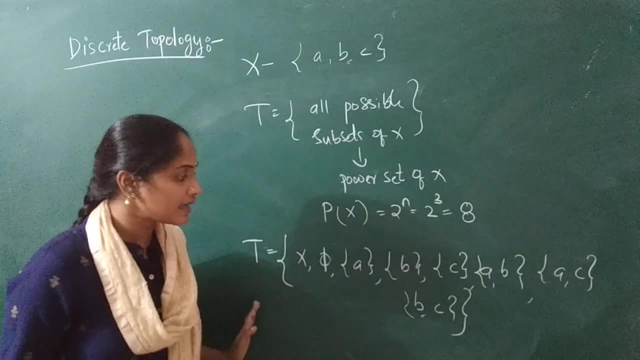 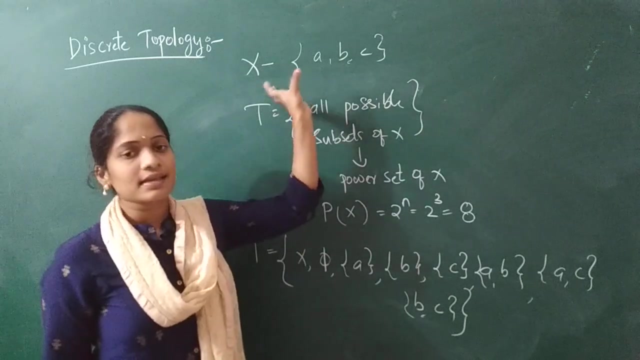 you have, you got. let's, you can take a comma b, comma c, a comma p is nothing but x. now let us count one, two, three, four, five, six, seven, yes, so these all possible? what is the word here? all all possible subsets of x is known as a discrete topology. you can say that x comma tau is a. 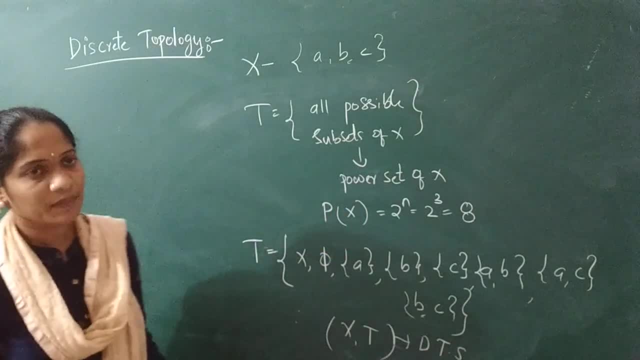 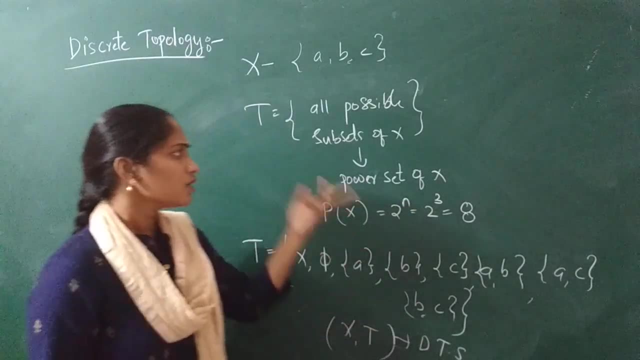 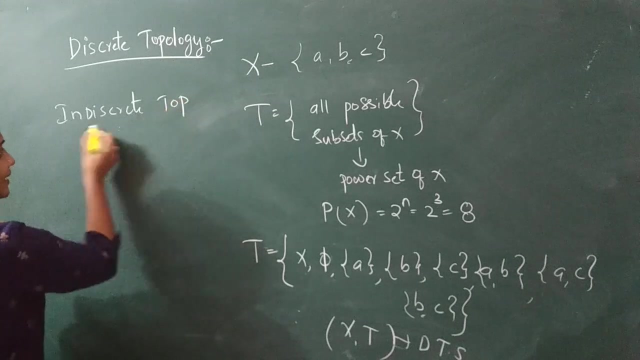 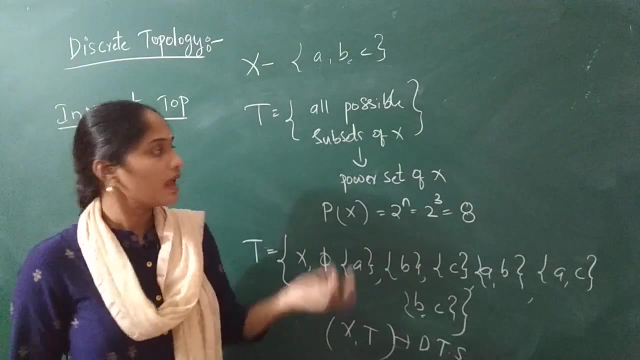 discrete topological space. or simply, if anybody asks you what is a discrete topology, power set of x is known as the discrete topology. so same coming to here in discrete topology, these also important in the indiscrete topology. what is indiscrete topology? yes, you have to consider X, any non-empty subset, and tau is a subsets of X. and now 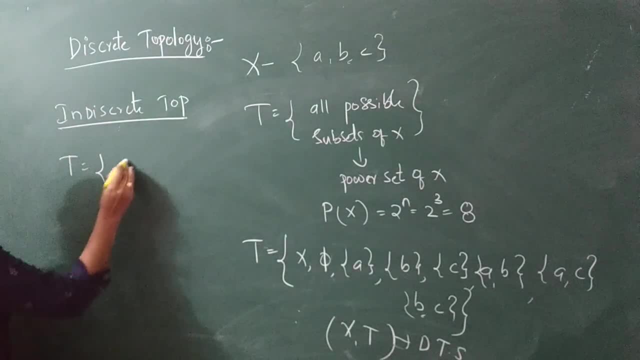 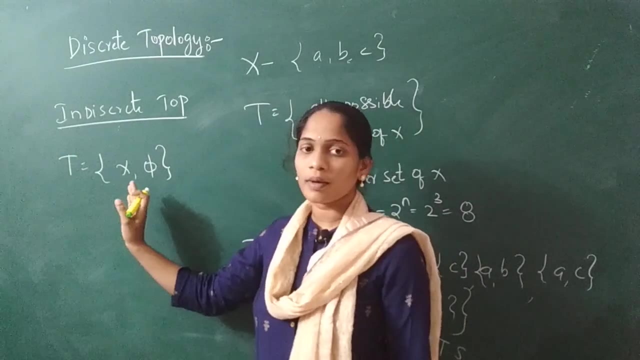 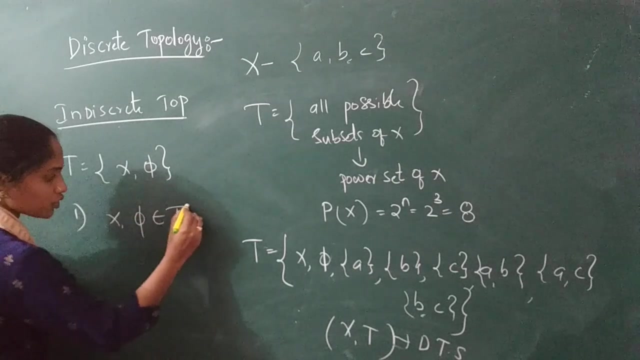 if I take, tau is equal to X comma pi. only how many sets are there X comma pi and that X comma pi? this tau satisfies the condition. the first condition is that X comma pi are belongs to tau. yes, the first condition. the second condition, its intersection. what is intersection pi, which is also belongs to tau, if you take? 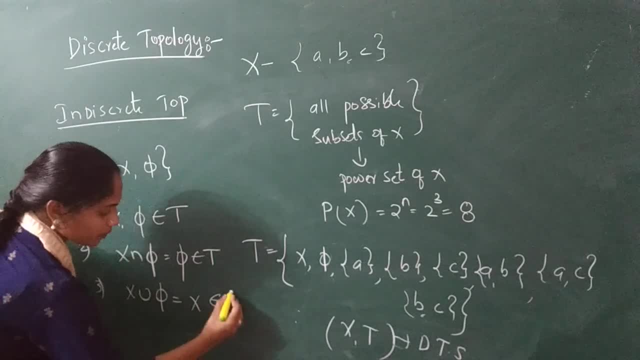 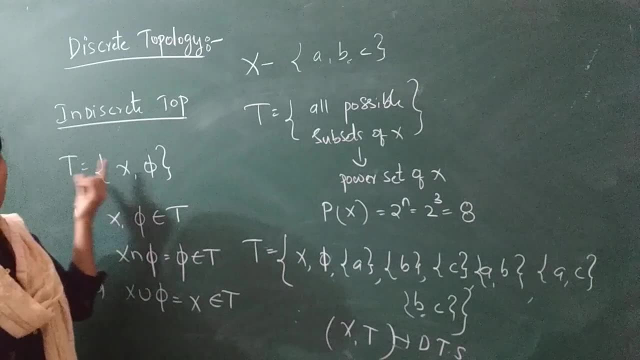 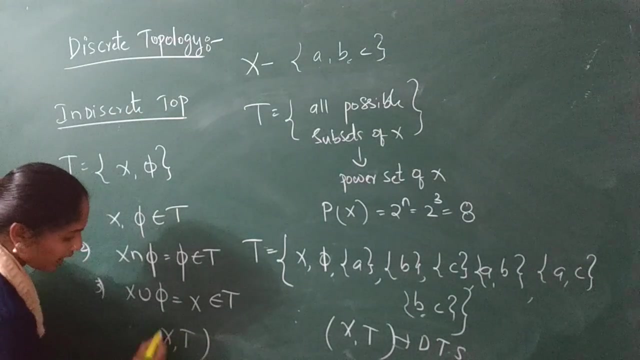 the union is X, which is also belongs to tau. yes, the three conditions of topology are satisfying. and these topology, that is, tau equal to X, comma, pi is known as indiscrete topological space. so therefore, the algebraic structure is X, comma is known as indiscrete topological space. got it so same what you put. 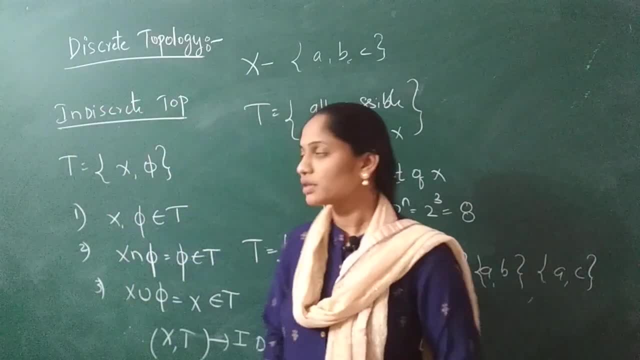 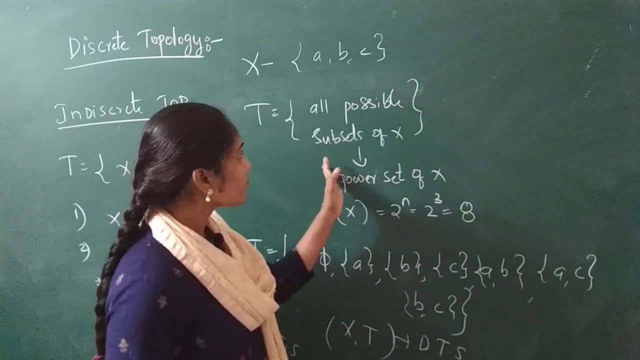 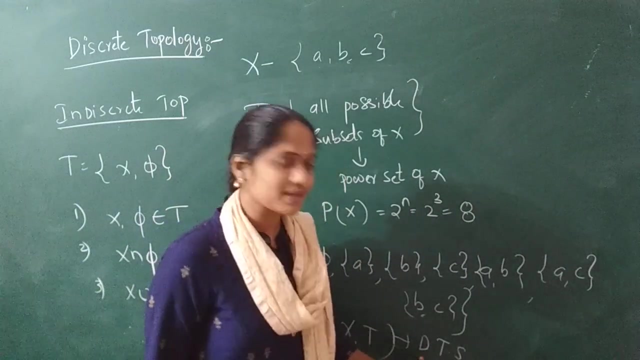 in tau. it means tau is X comma pi. that's why I satisfied these three conditions here. you can have the doubt that please take possible subsets. does these make them topological є? since it is a topological space, we can call it discrete topological space. if you check this, then your topological space is tells us that. 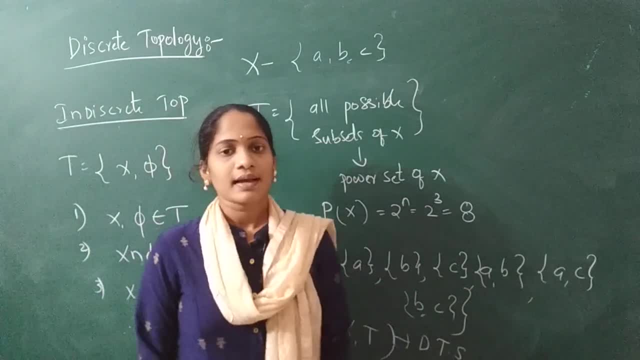 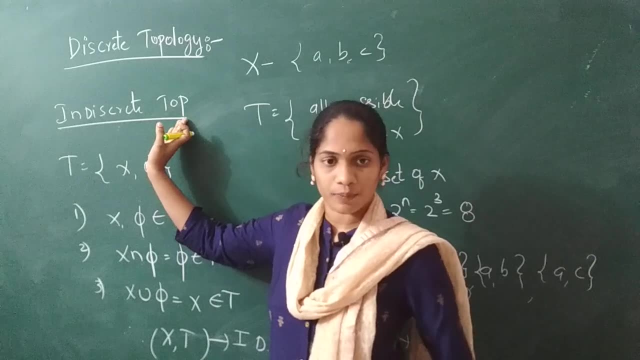 So discrete topological space. But the word is the power set And all possible sets should be there. Subsets should be there. Same when we come to indiscrete what should be there in tau X pi. 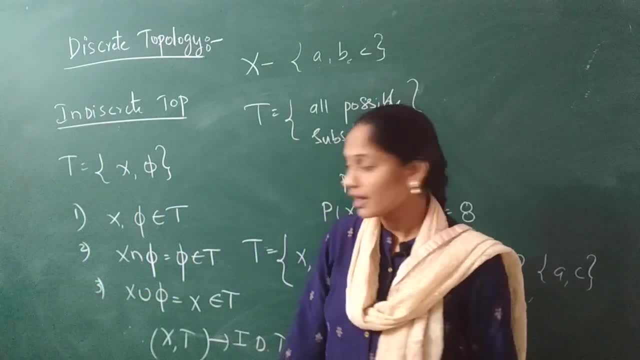 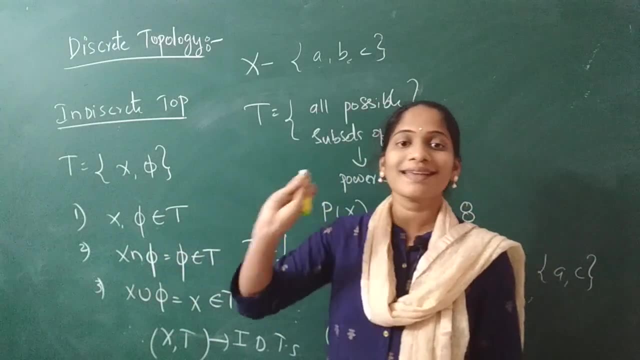 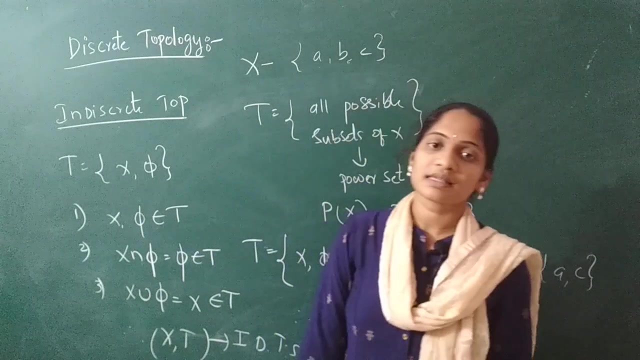 So that is indiscrete topology. First topological space should be there or not. So satisfy the topological condition. Yes, three conditions are satisfied. The only sets X, pi should have there in tau. Then that tau is known as indiscrete topological space. 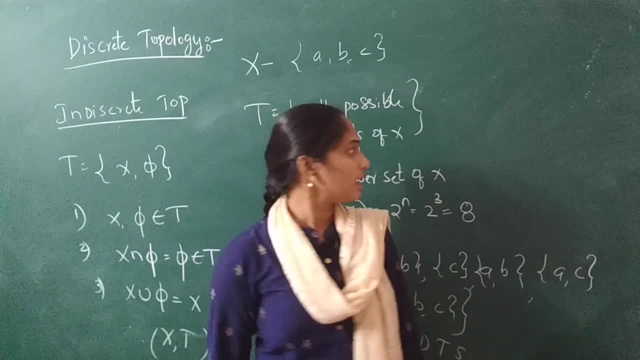 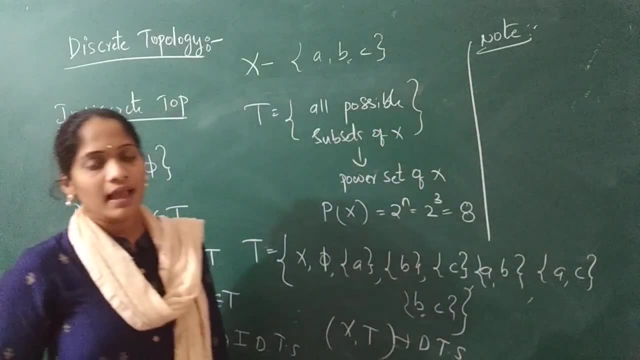 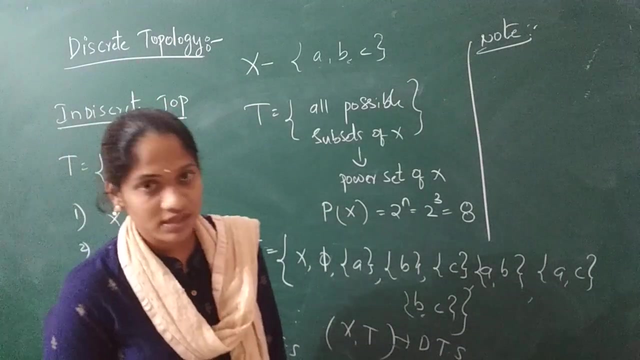 So this is your discrete and indiscrete. So here, one note is there which is important. I am saying that here, at one condition, at one stage or anything, this indiscrete and discrete topology will coincide What I am saying here. 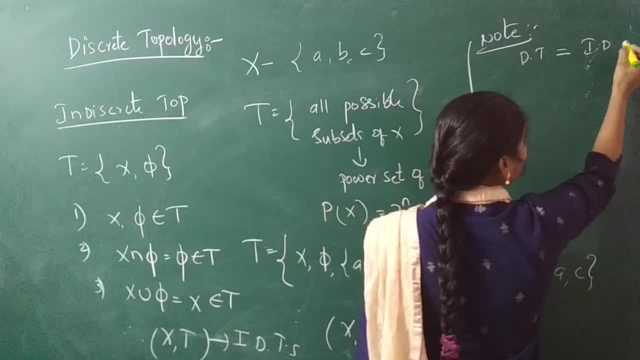 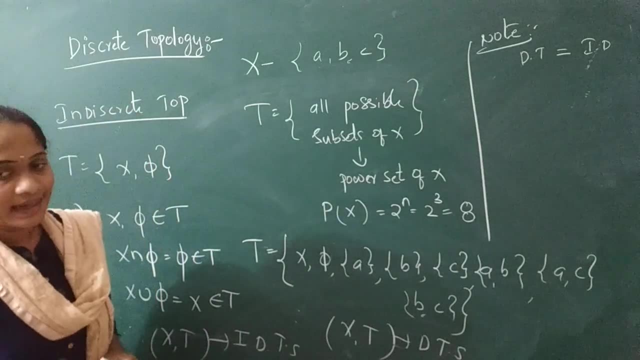 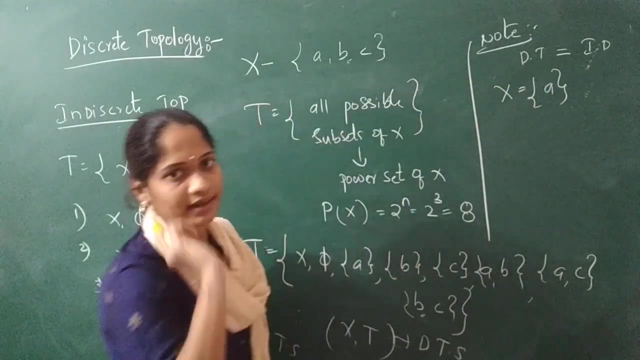 discrete topology and indiscrete topology will coincide If these two match. at what condition? What do you say? Yes, if you take X, the non-empty set X, to be only the single term set, Got it. If you take only the single term set A in this X. 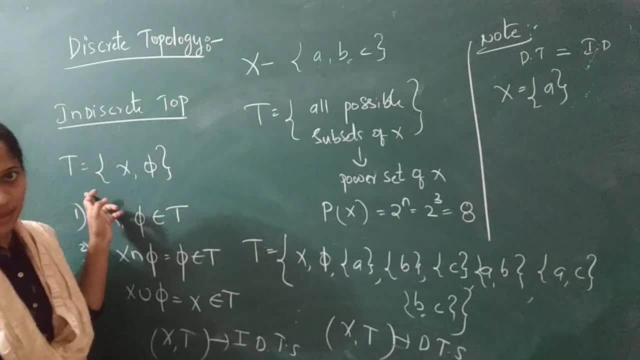 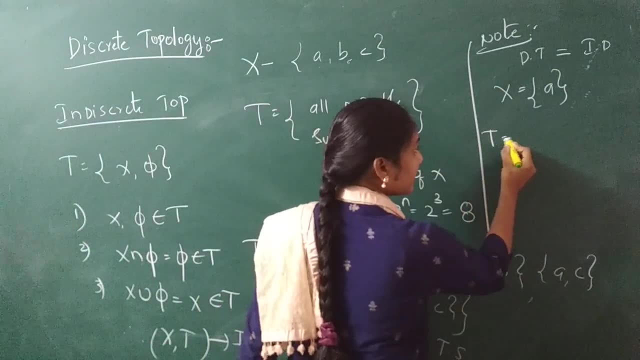 then I am saying that these both topologies- tau, will be there, right? If these two also coincide, what will happen to you? Let's see how. First consider tau. What does this mean? Indiscrete topology- let's see. 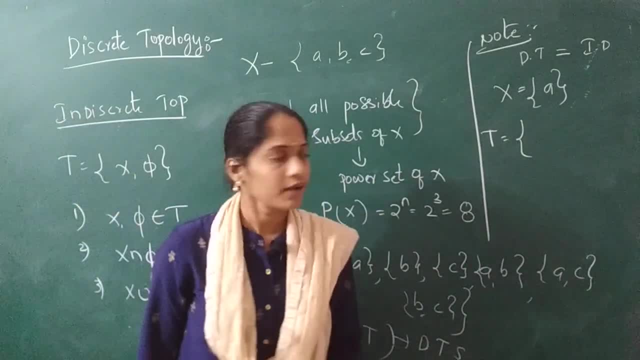 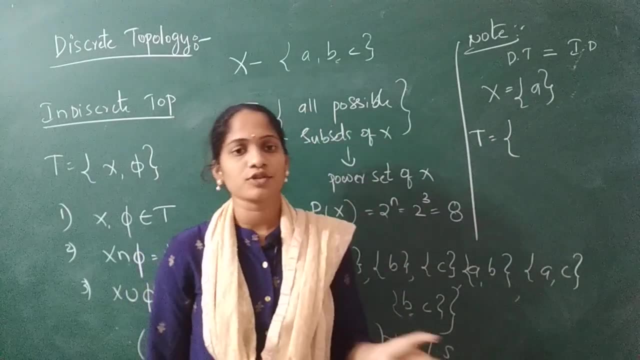 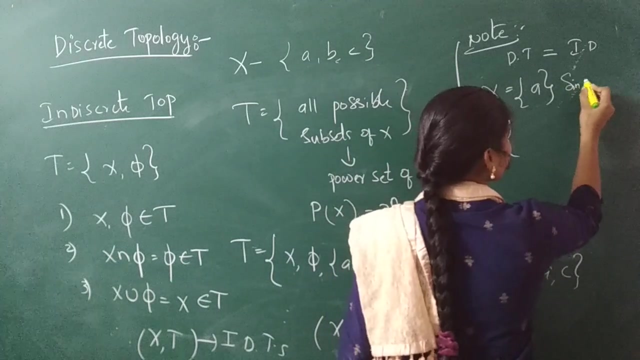 What does discrete topology mean here? See, I took a non-empty set of X. Now what I want to say is discrete indexes and topologies if two coincide at one stage. when you take X as the single term set, when you consider the single term set, 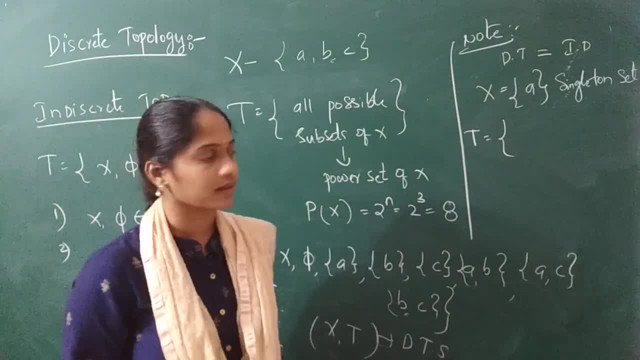 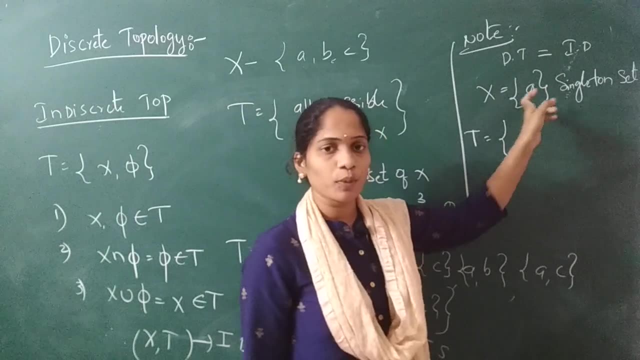 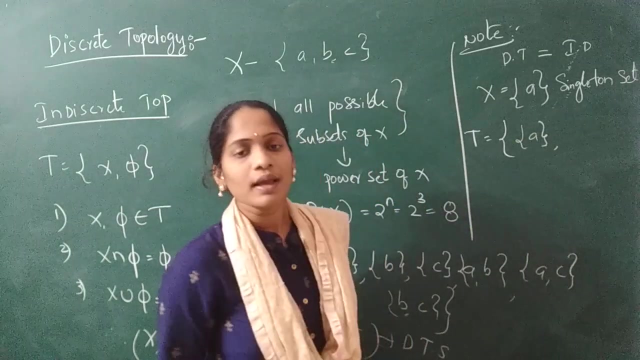 discrete topology and indiscrete topology will coincide. So now we are looking at discrete topology. What is discrete topology? All possible subsets, All possible subsets of X. What is there? You have only one single term, set A. What else can you say? 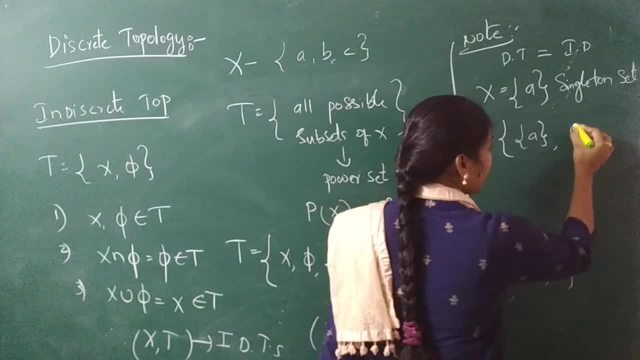 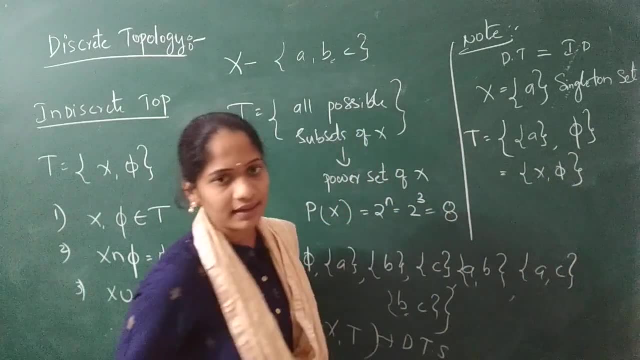 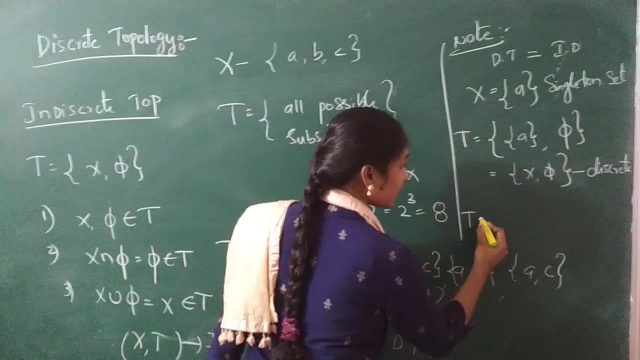 Pi- Empty set- is subset of every set, So pi is compulsory. So now, what is X? Is it X, X, pi? Is that clear? What is this? This is discrete topology, right, When you are coming to the indiscrete topology. 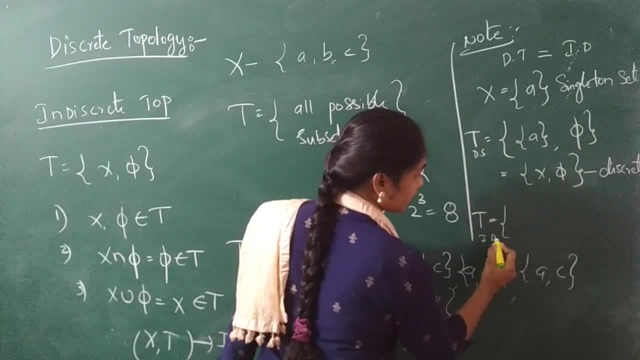 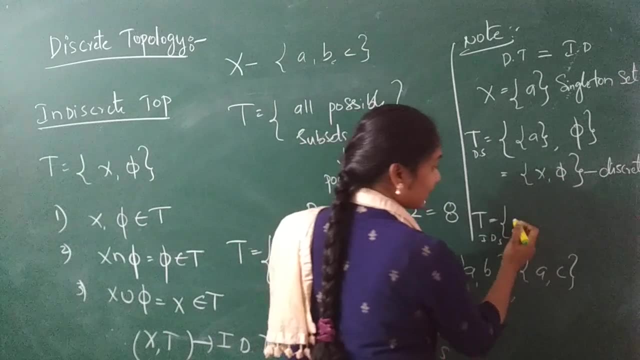 this is discrete topology And this is indiscrete topology. What is indiscrete topology? How many sets? you have to consider X, pi Here directly. pi is the first empty set And you have to consider here A only, And A is nothing but X. 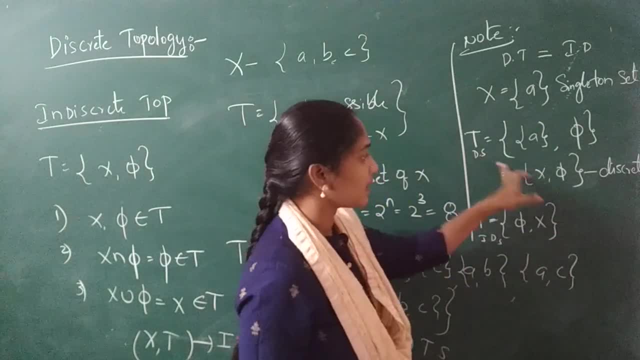 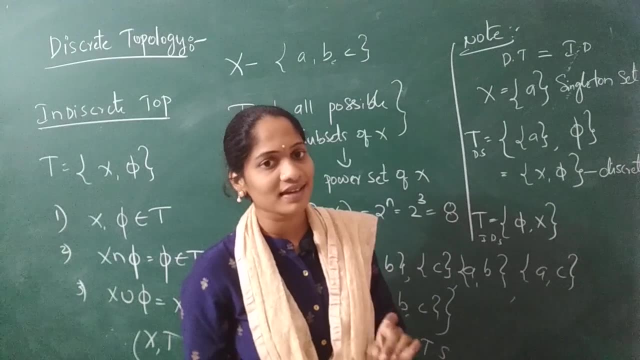 Yes, If you are coming to the discrete, it is X pi. If you are coming to the indiscrete topology, it is also X pi. So now what? you can conclude? that yes, when you consider X to be a single term set. 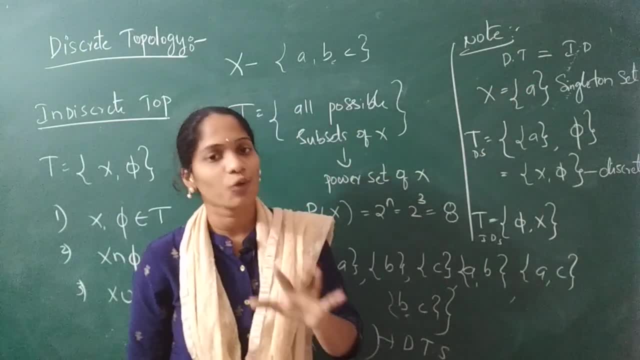 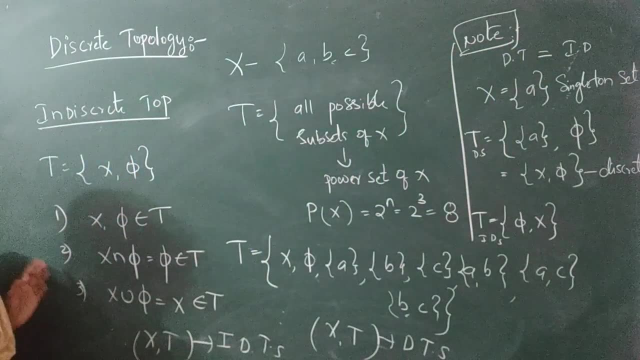 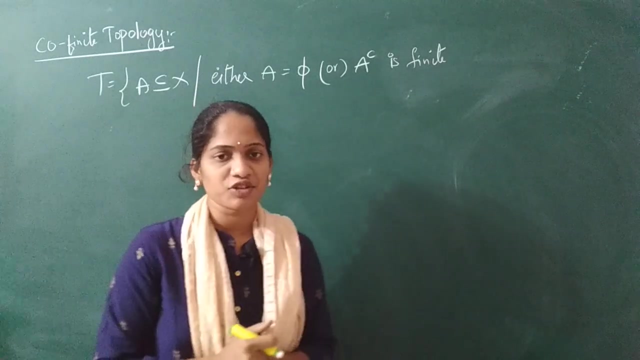 the discrete and indiscrete topologies are getting coincide. So this is a very important note Should be remembered. So this is about the discrete and indiscrete topology With examples. let us see the co-finite and everything. Let us see a small definition that is co-finite topology, right? 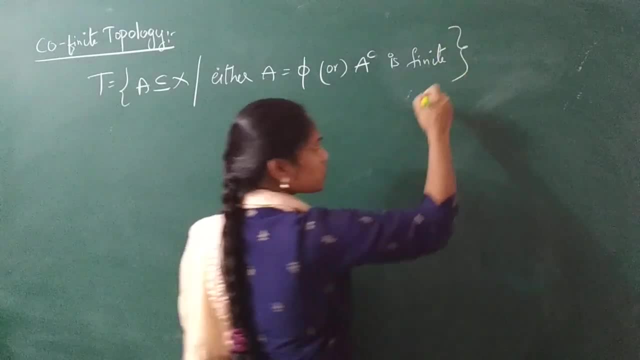 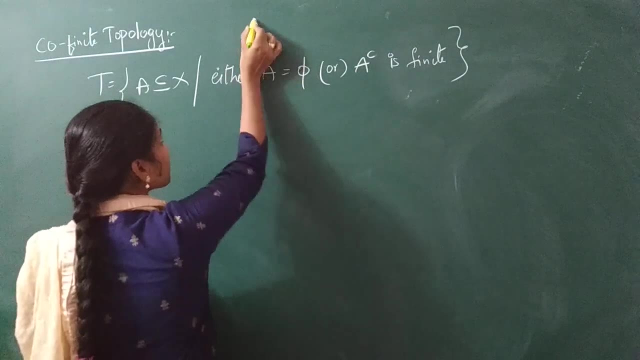 Co-finite topology is used a lot by you already. You know that, I think. So what is this? Just nothing. but you have to consider here: X is infinite set. You have to consider X to be, X to be some infinite set. 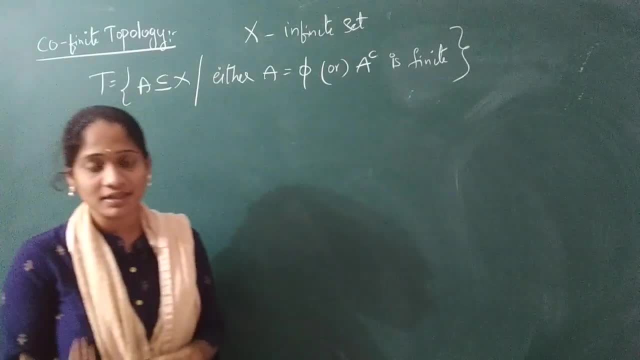 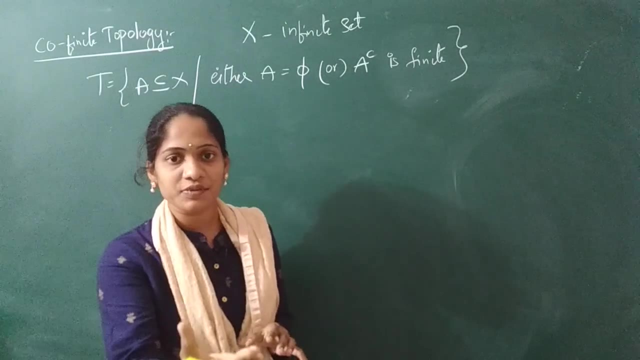 So next the tau should be how the tau should be considered. The tau should consist of all empty set and all subsets of X, and that all subset that the complement should be finite. Got it? So you take topology. What should be in topology? 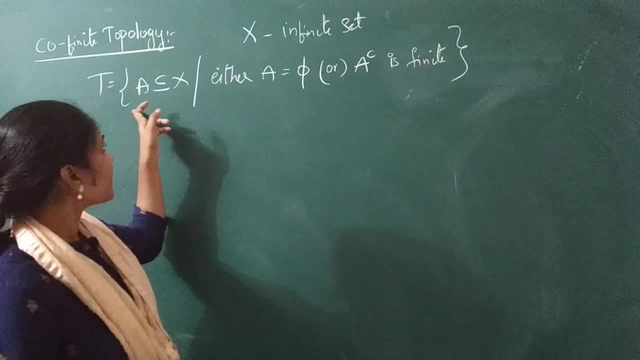 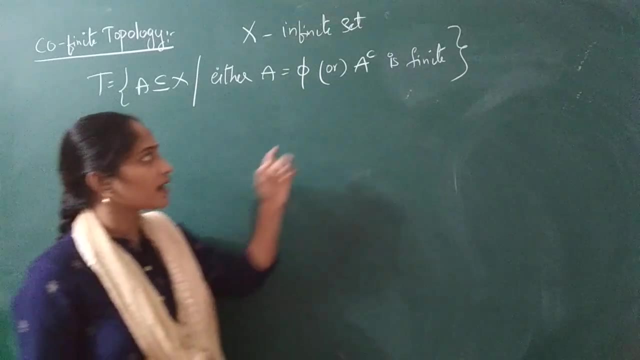 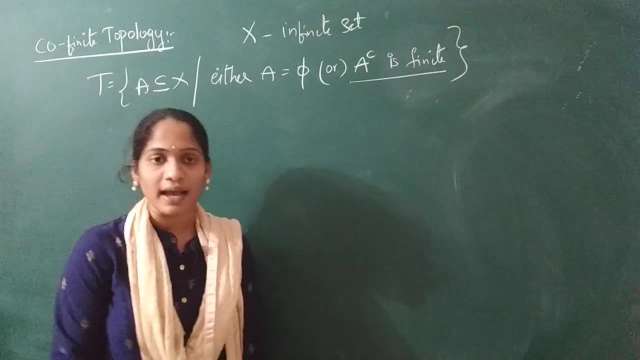 Pi should be, Empty set should be. And what is A subset of X? Yes, All the subsets of X should be there. The condition is that all the complements should be finite. So if this condition is satisfied, in particular, 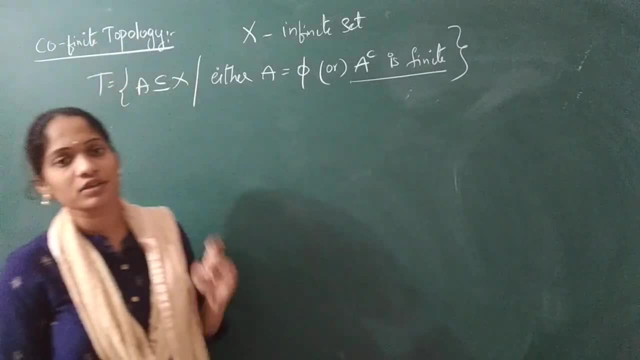 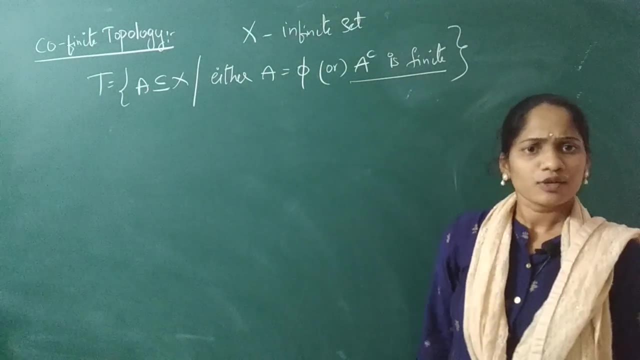 what do we call that topology? Co-finite topology? Simply, you have to remember that the subsets of tau, their complements, should be finite. Right So same. in that way you have co-countable topology. The same definition is applicable here. 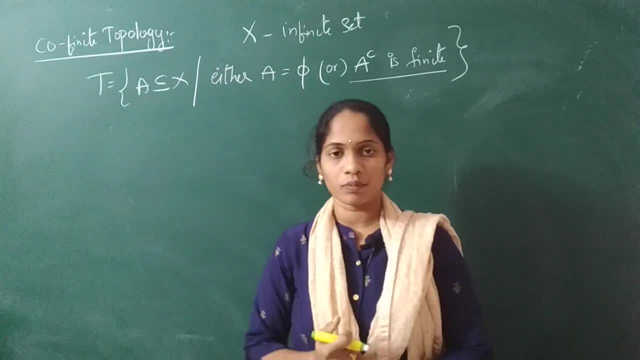 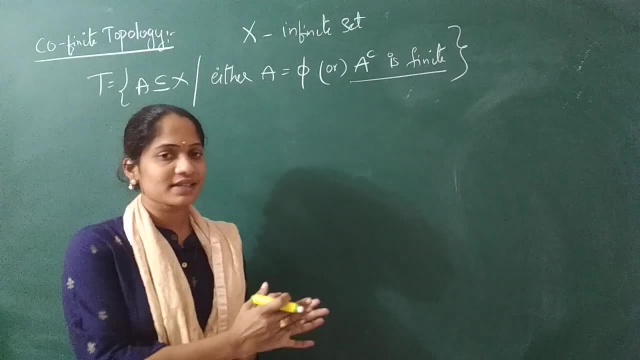 Instead of the finite, it should be countable, The complement should be countable. So here, in the previous topics, what we have? I have just only told you that open, set and closer. only some example, one-one example. 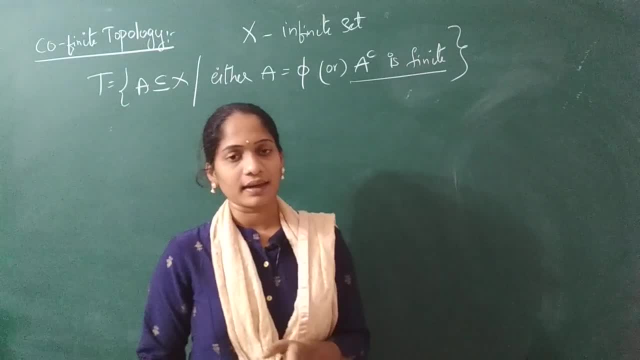 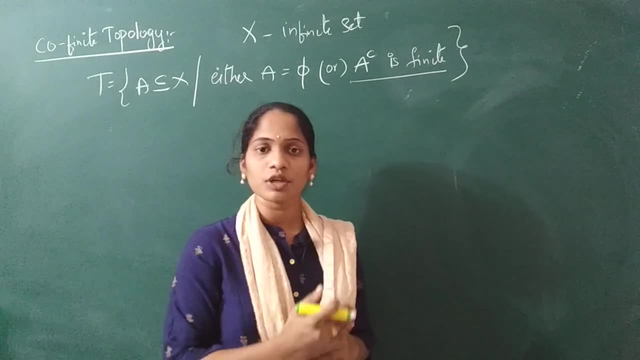 Here now I want to say you that both open means if you take an X, like this, if you take X, non-empty set, so in that we can write open sets, We can write complements using open sets. 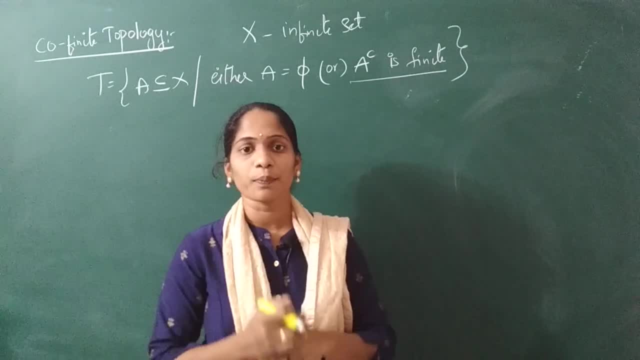 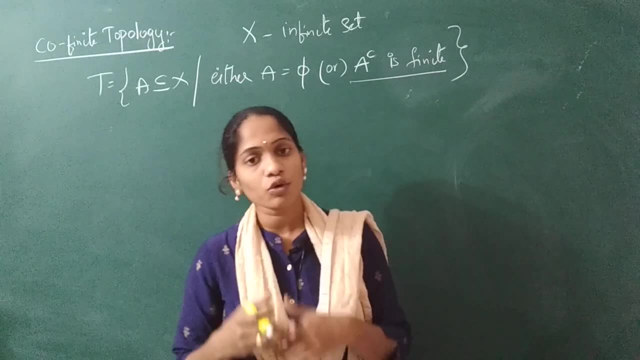 and close sets. So what I am saying is both open and close sets. are there Means one set? is it an open set or a closed set? Like both? are closed sets Like one set if we take it in X. 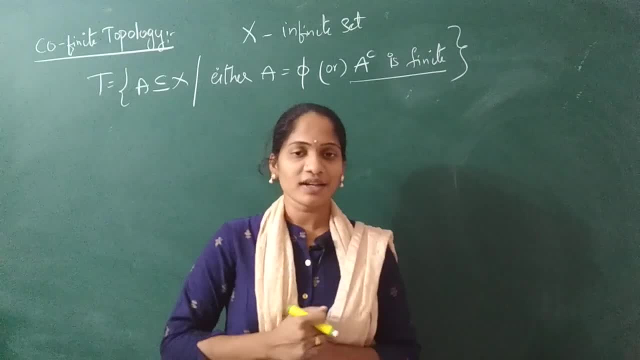 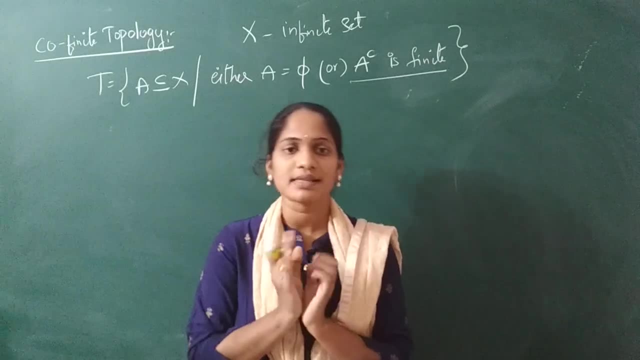 it is not open, it is closed. There are such sets also. So let us discuss now Means. let us do an example. There is no definition, Just only for clear picture. I will give example for you, Right? So there is here. 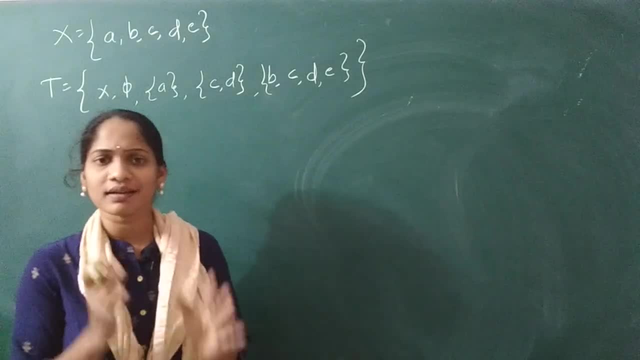 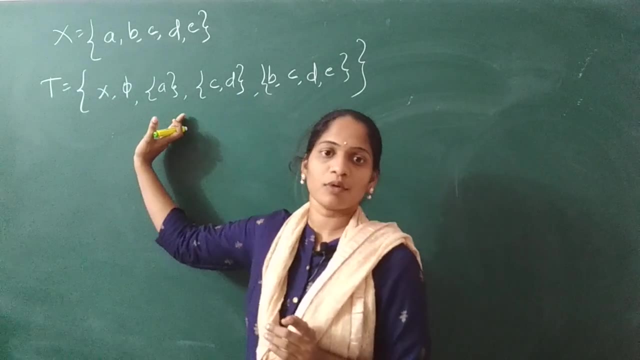 one example for you which picturize very, very clear picture for you. Because till now, what did you know? There is a non-empty set X. We took Tau, So Tau. if we want topology, we need three conditions to be satisfied. 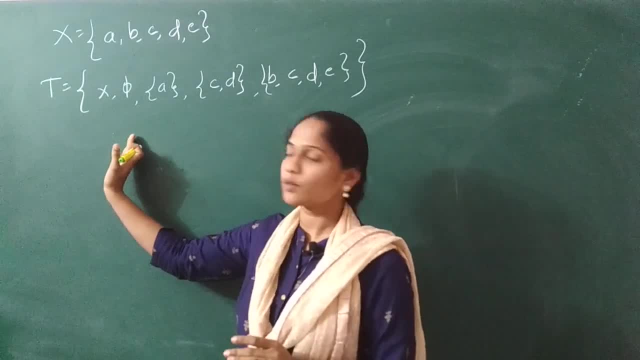 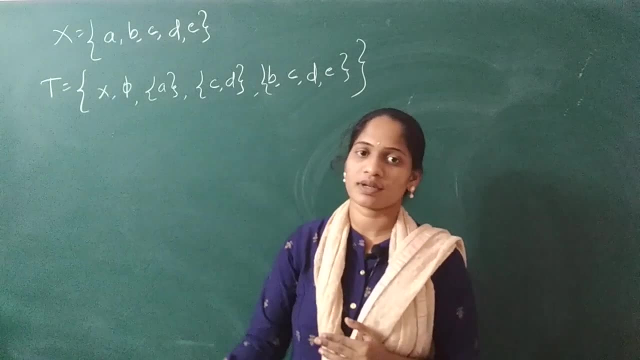 If three conditions are satisfied, so that Tau, we call it topology, and X, So if that condition is not satisfied, we know that it is not topology. So just like that, we also said open set and closed set. So open set is simply: 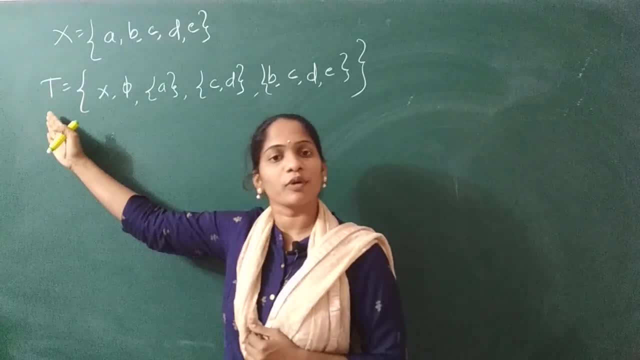 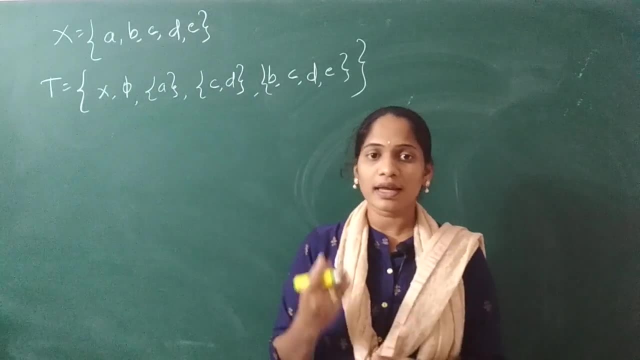 what I told you all these members means Tau topology. these two are called open sets, So one of those complements closed sets. we learned till there. So here one note means like small note. 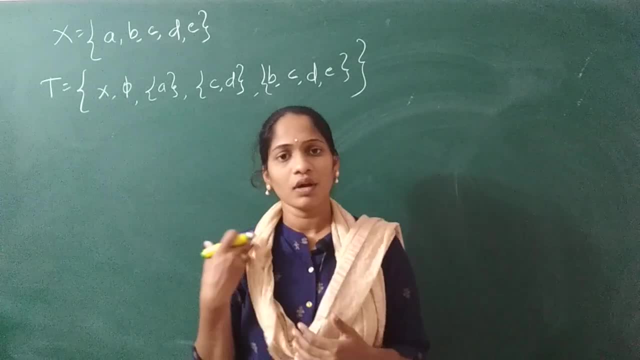 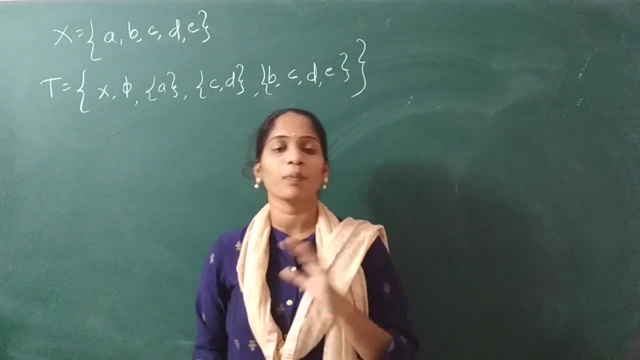 one point important means: you can do it in exams. you can do it in MSA exams, anywhere, competitive exams, anywhere you can get such clash, Whether this set is both open or closed, whether this set is neither, or is there any sets? 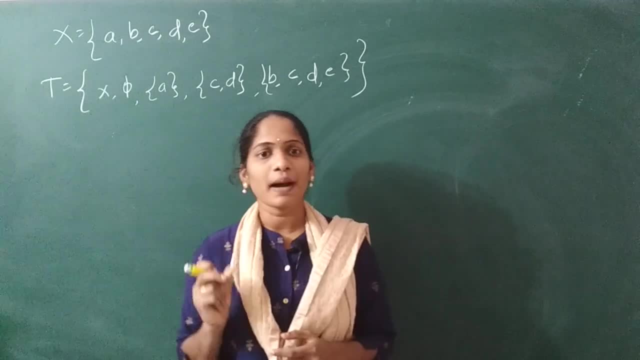 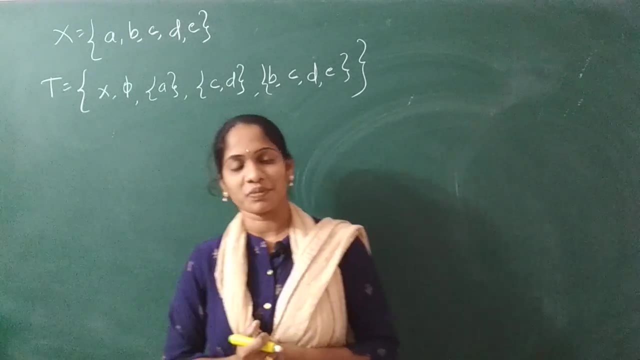 both same open and closed. So when we get such marks we will be a bit confused. Yes means there is a chance that one set is open and closed. Now clarification course. this example is for you, So here. 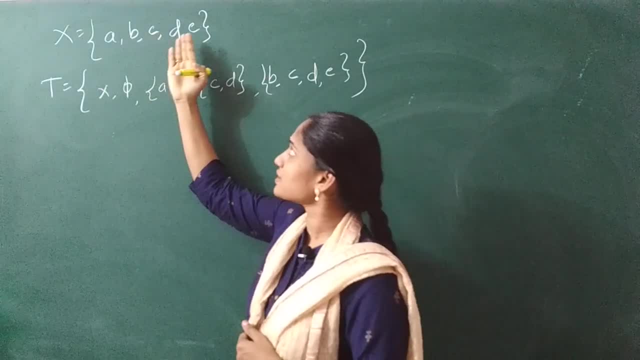 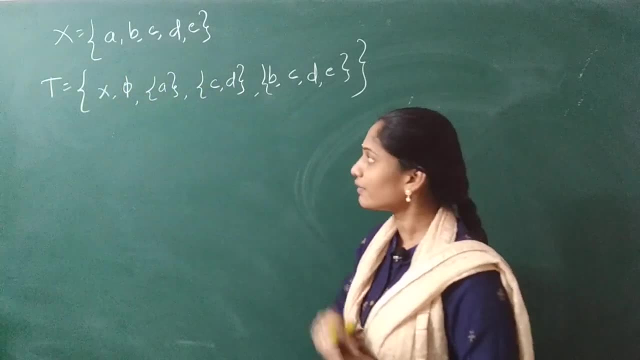 what is here? I have taken a comma b comma c, comma d, comma e, Now five elements or five points in the set x Right, And I have taken some subset. These are all what subsets of x? So now, 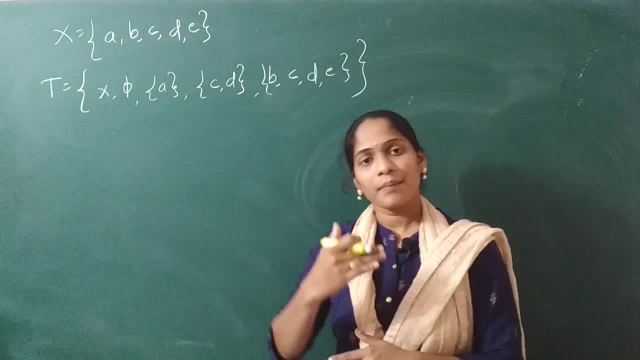 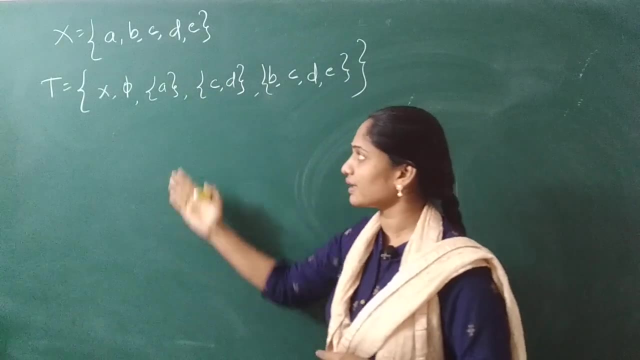 I am telling that and I am not proving the topological space. I know I have already done this is a topological space. If you want to do, you can. you can check the three conditions whether this becomes a topological space or not. 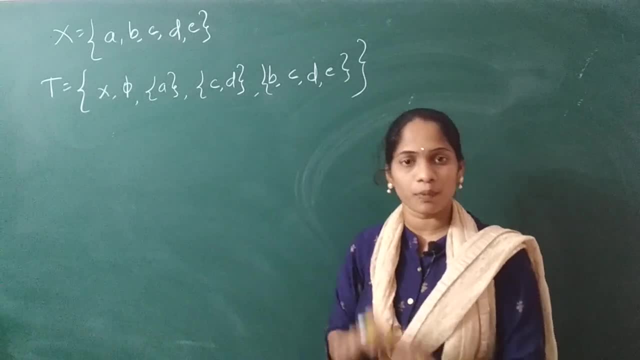 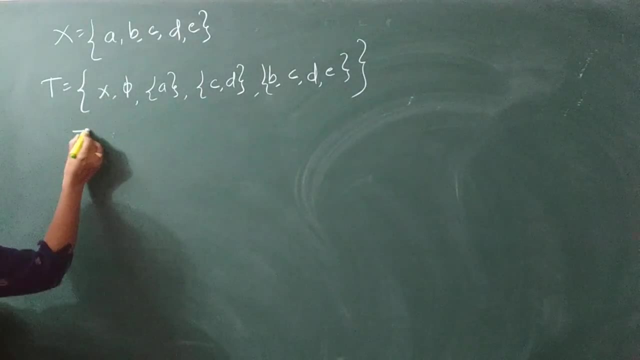 So now here, I want to check only the open and closed resets, whether they are both same or neither same or not. So now these: as this is a topological space, I am writing here: Yes, I have proved that. 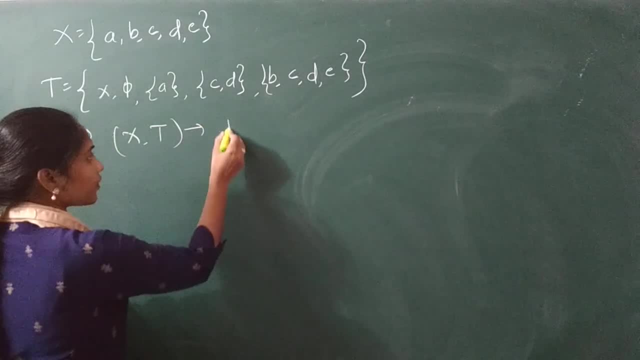 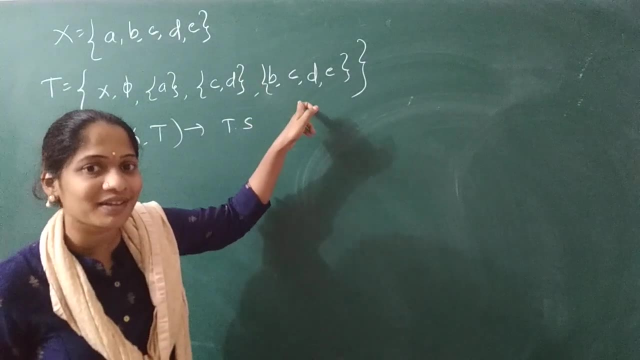 this. tau is a topological space and algebraic structure equated with this is a topological space. So, as it is became, this is a topological space. The members of tau are not nothing but yes, open sets. So clearly. 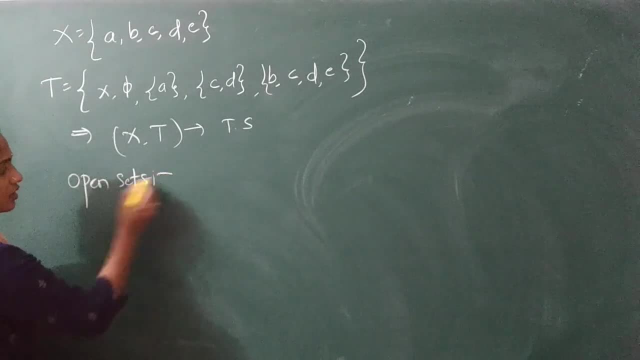 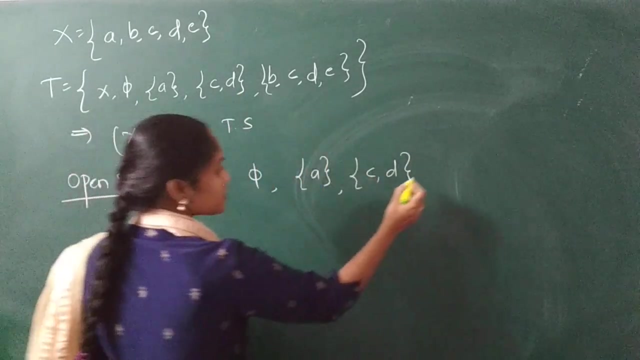 or directly. you can write open sets. How many open sets All these are becomes open sets, right? So right here, x pi singleton, set A, c, d and next b, c, d, e. So these are all open sets. 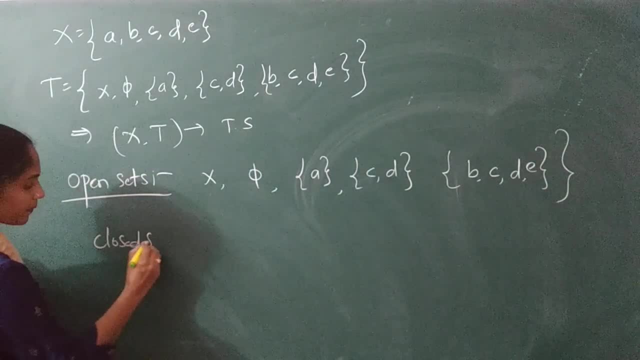 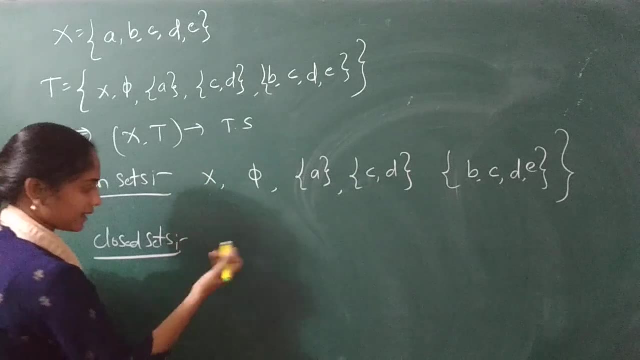 right Now we want to write the closed resets. Closed resets- Already we have discussed. closed resets are nothing, but they are complements. What is x complement? Yes, it is pi. and what is the pi complement? Yes, it is x. 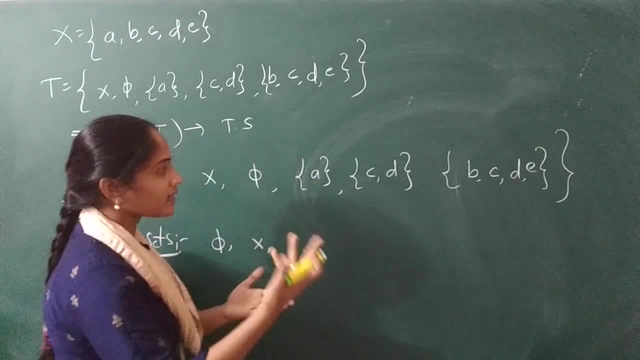 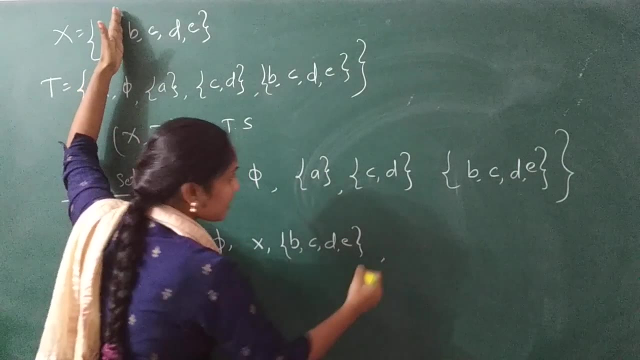 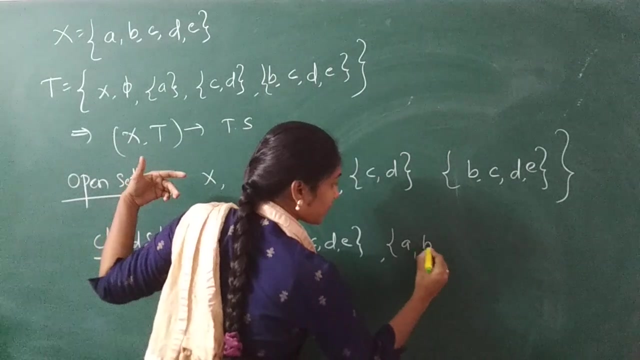 and what is the a complement x minus a? If you take out the a, how many elements b, c, d, e? Yes, if you take c d complement x, c, d, and how many elements a, b, e? 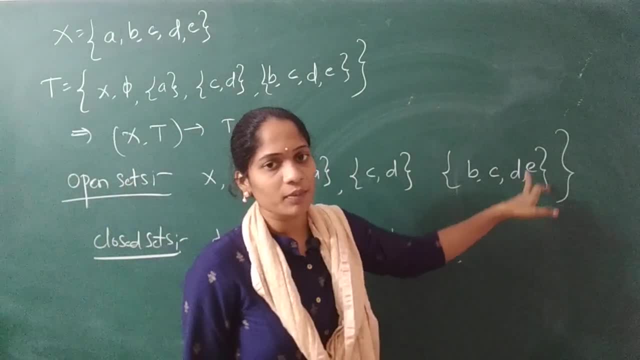 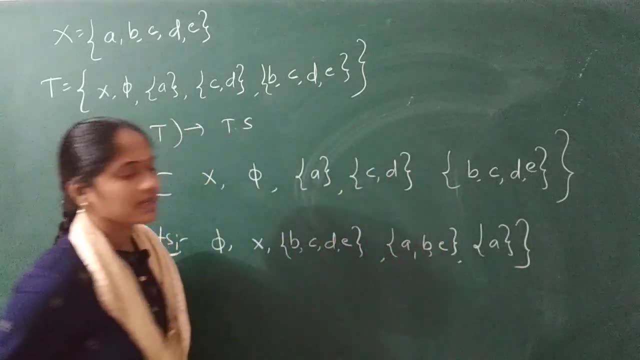 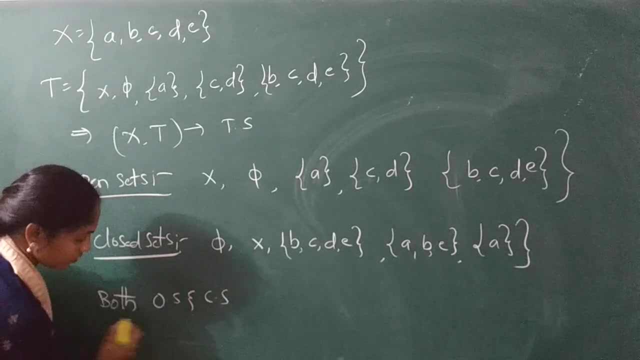 b, c, d, e, complement. If you take out all these elements, what is that? Singleton set A: Yes, So these are all the closed resets. So now here let us check both open sets and closed resets. 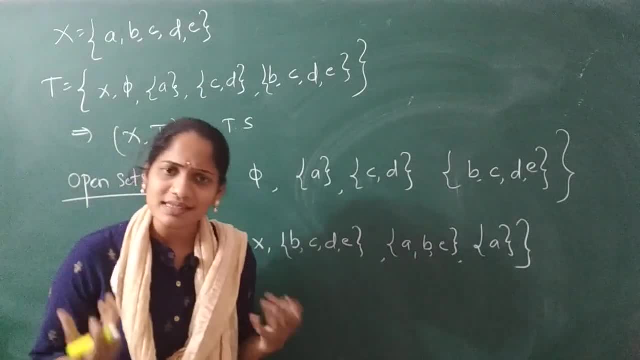 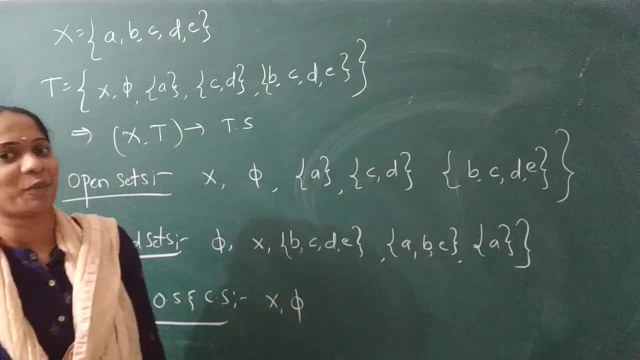 Both. Both means the same IAT unit. Yes, it is clear that x, pi are always the open sets, If you take the indiscrete topology. yes, you have to go. When you do this, you have to get some idea. 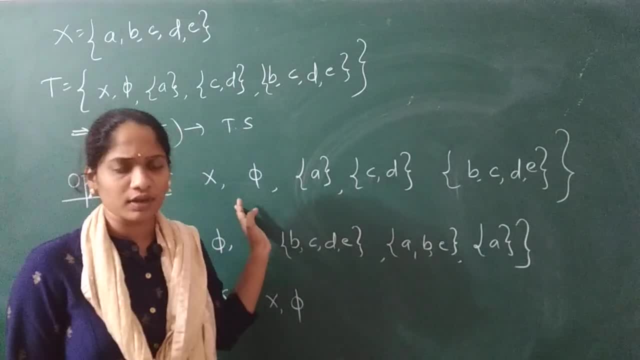 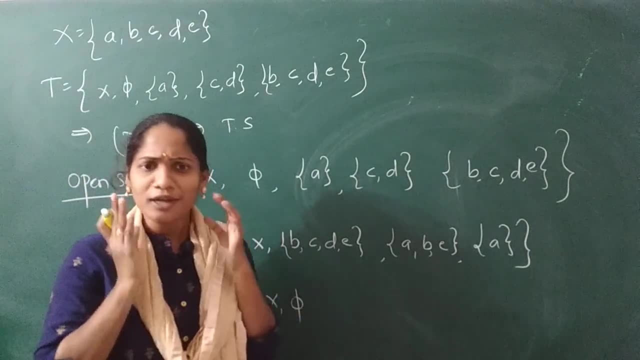 What did I say about x pi? If you take an open set, it will be open and closed. Only topological space on x pi. Only topological space on x pi. Yes, that is nothing but indiscrete topology. 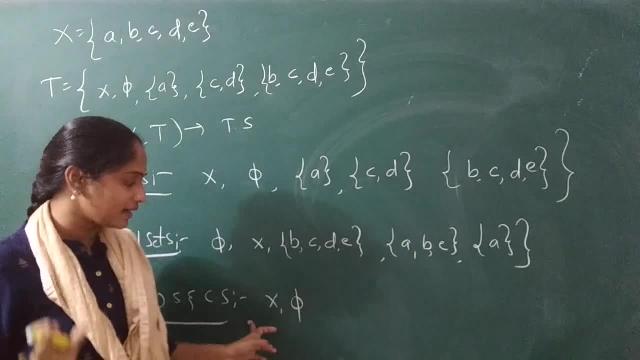 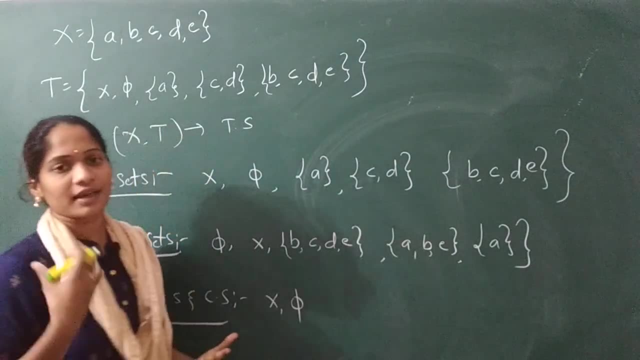 So if you take such indiscrete topology, that indiscrete topology is always open and closed resets. Yes, you are very sharp students. What did I say about x pi? You have to take x? pi as indiscrete topology, So that becomes always open and closed. 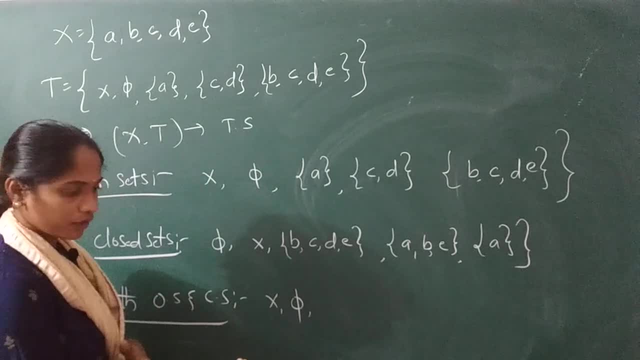 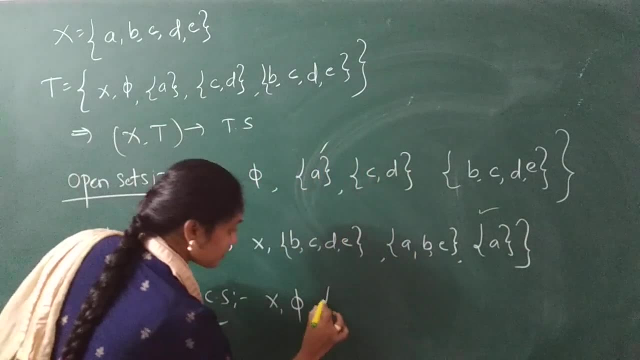 So let us leave it. So now, what do I have to do? Both open, So x pi. If you take the singleton set, whether it is there, Yes, Stick, Yes, Both open and closed. Is there any other set? 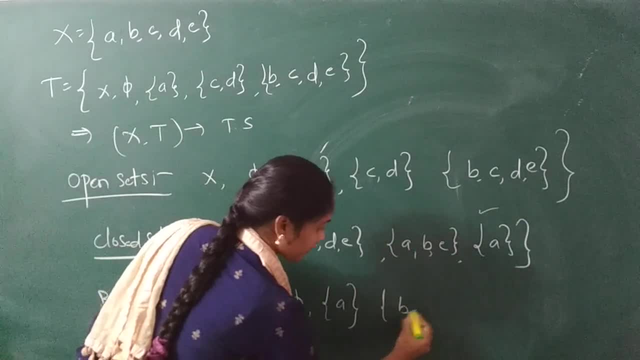 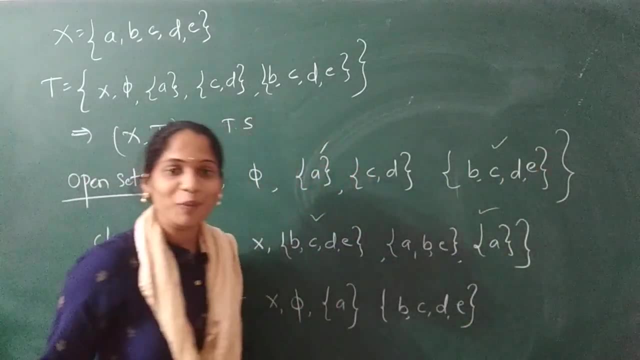 Yes, B, C, D, B, C, D, B, C, D E. So these are the both same sets, Both open and closed, Both closed sets, Right. So both of these are also open and closed. 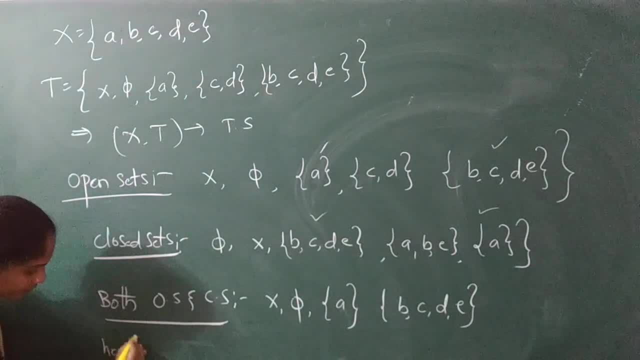 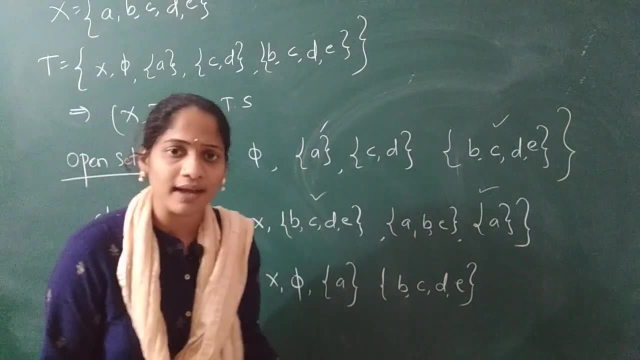 Right, Let us see the neither, Neither nor. Neither open set nor closed set. What does that mean? It is not open set and not closed set. What is that, madam? Is there anything else other than open and closed sets? 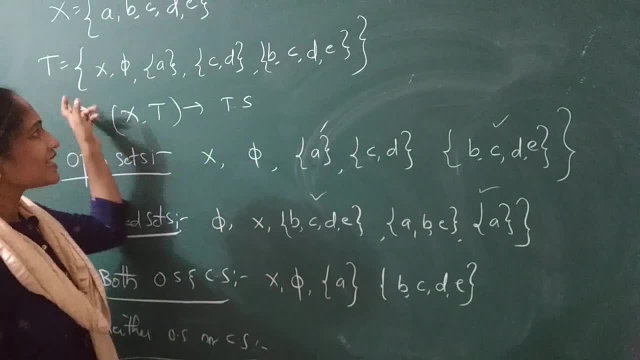 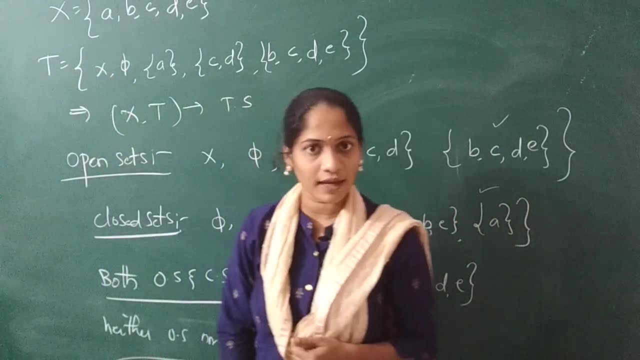 Yes, What is that point? You have to got that The topology we have taken is not a power set, It is not a discrete topology. If you take a discrete topology, then what will you get? All the subsets will come. When all the subsets come. 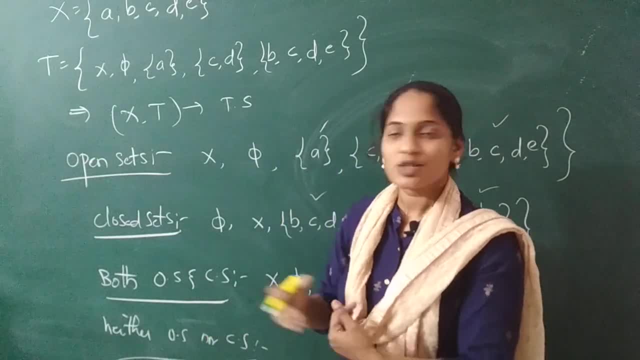 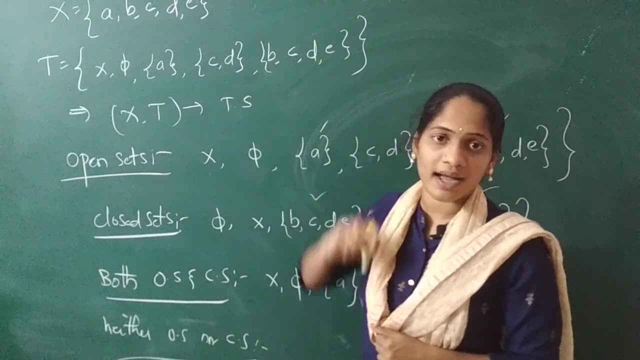 surely you want it to be open or closed, So I took a normal topology here. I took a normal set. It is not a discrete topology, right? So, other than this, you will also have subsets for this set, right? 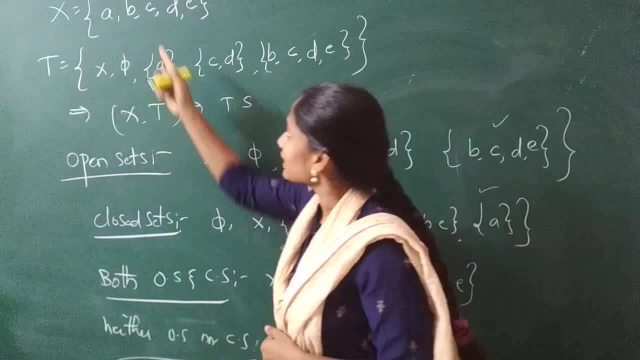 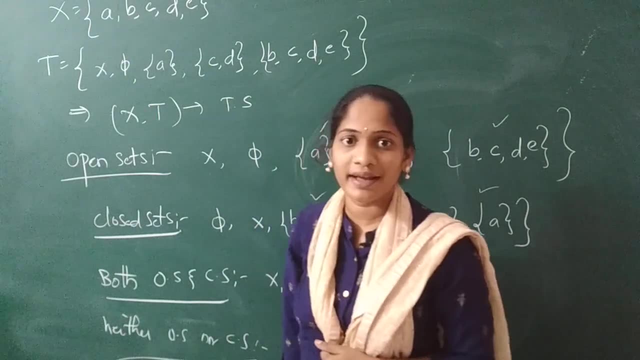 Yes, You took singleton set A. Do you have singleton set B? Do you have C? Do you have D? Do you have D? If you missed 4,, what is here? 5.. It is a 2 power 5 element. 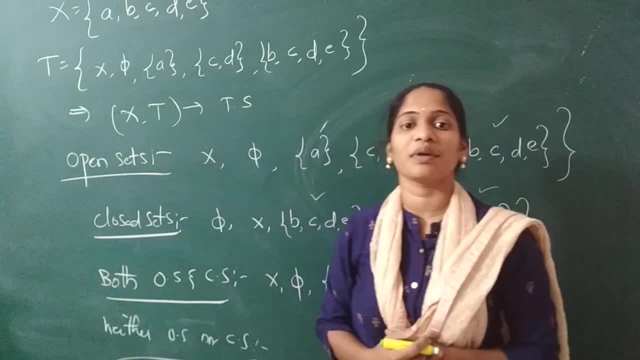 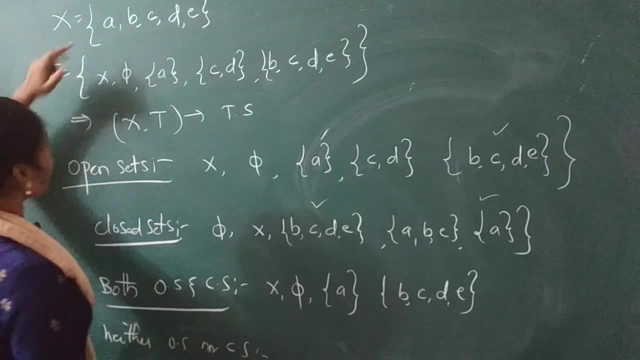 So what do you have here? There are many other elements, So all these subsets will understand this also. Yes, Let's write a few points for your clarity. So here X is yes, It is a pi. A came as a single template, A. 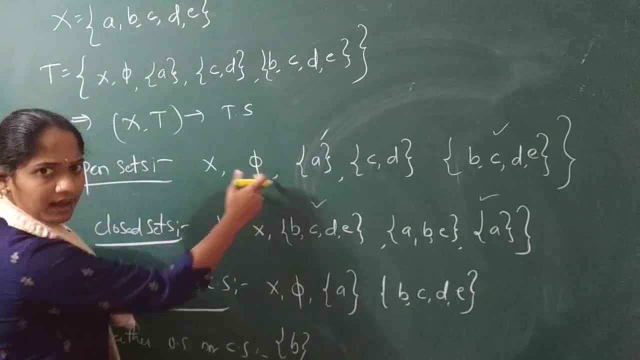 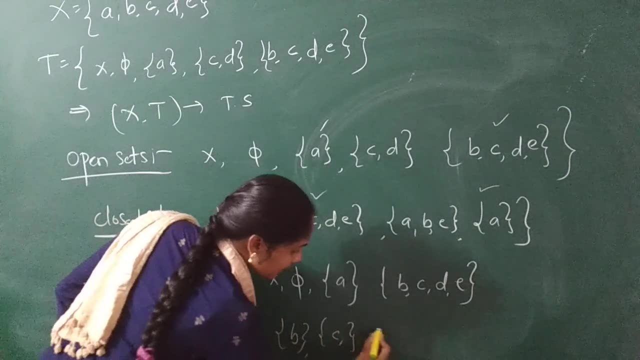 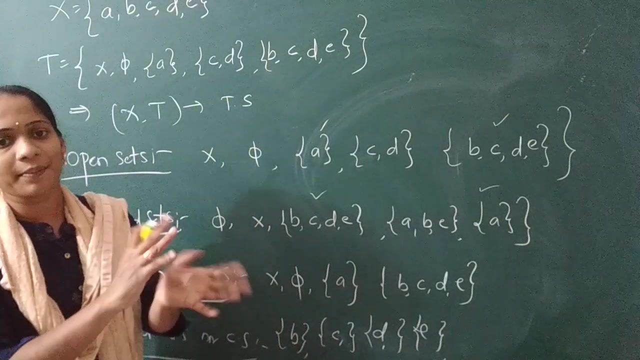 What should come next? B Is B open set, Is it in open set or closed set? Not closed card. let's see same C and D also. E, also singleton set: unknife. a open card or closed card in card, double shoot them: a comma, B, a comma, B, a comma. 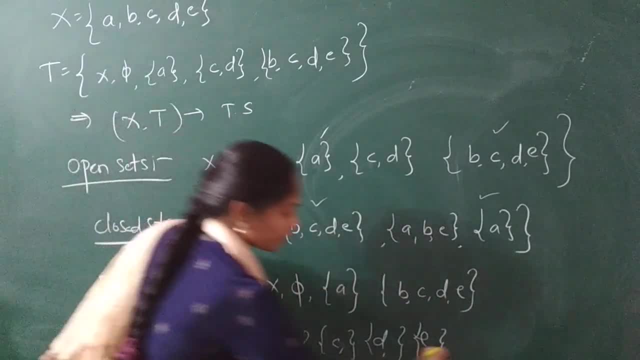 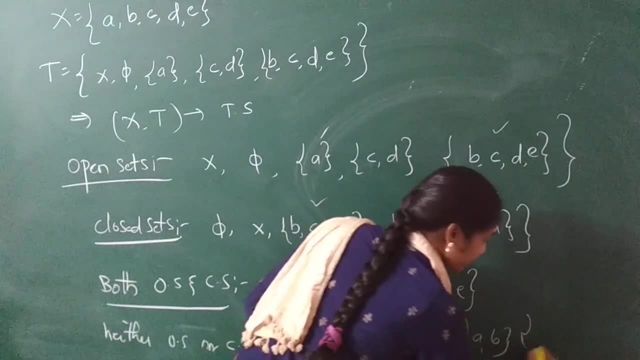 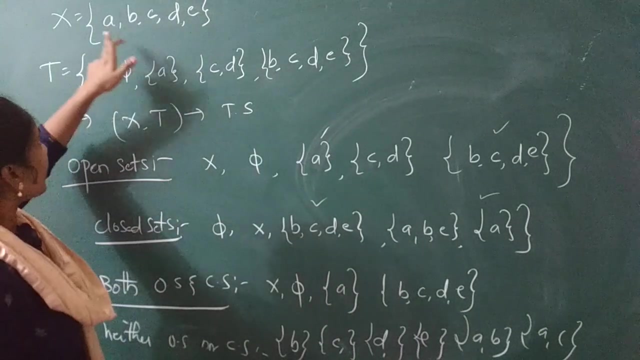 B in the economic. oh my, be a comma, be a, do so. a comma B, so same a comma C. let's shake. a comma C, no a comma C, I don't know. a comma D, a comma E. then go to the three, three elements. I said ABC. where is the nate years ABC? is that ABC or a? 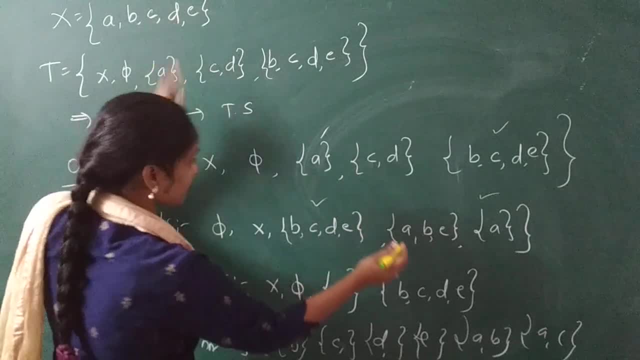 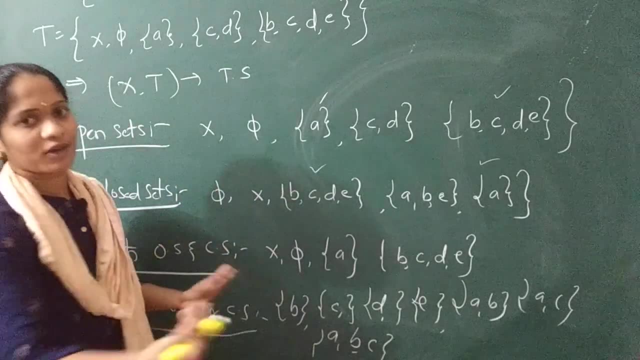 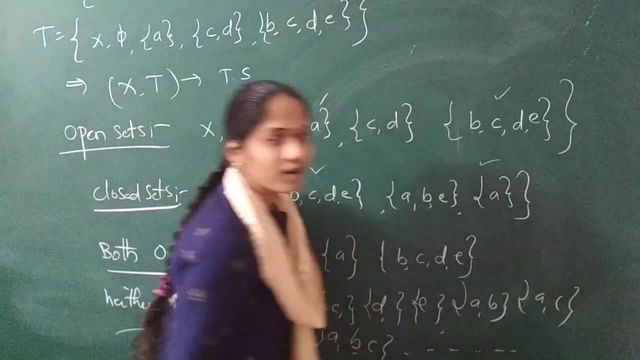 B, e. let's check C comma D, see come it is e. so there is no a comma B comma C here. so a comma B comma C if you take a B, D, AB, DS, there, no, so how many? and so on. so there are some sets which are neither open set. 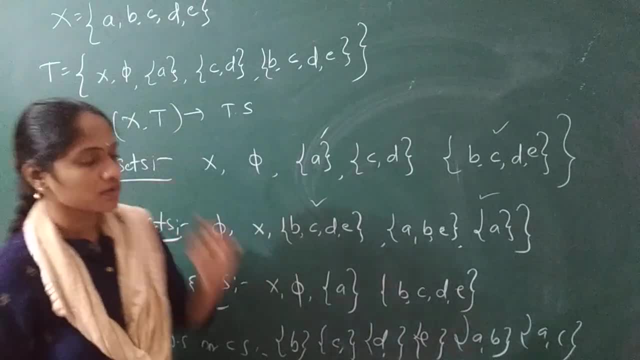 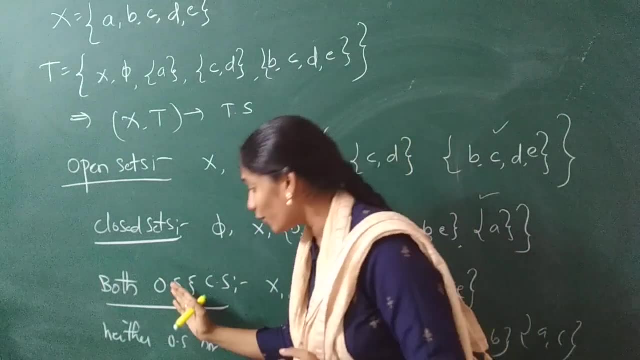 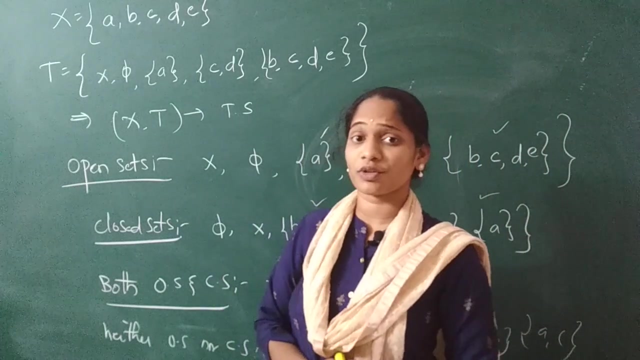 oh, nor closed resets got it. so me Rocco set these content on empty set. our topology la una carcana. me open, sets close. yet Susie conni sets make both open, close. java choo conni, motham kaka pochu in coca chance and incook example. to me, clarity is turning a chapter on and I example. 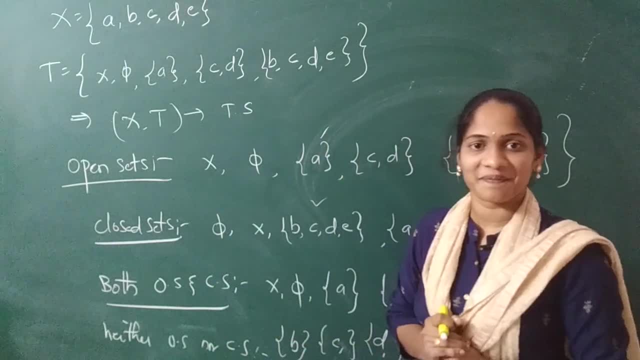 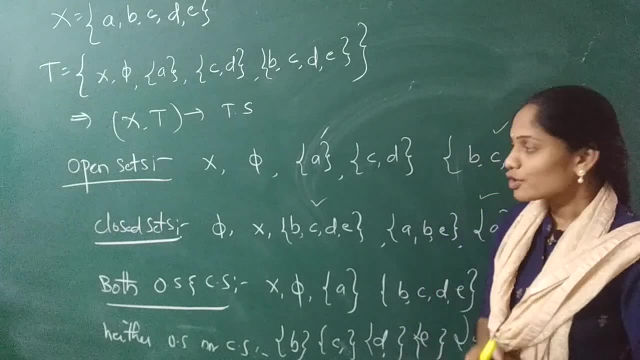 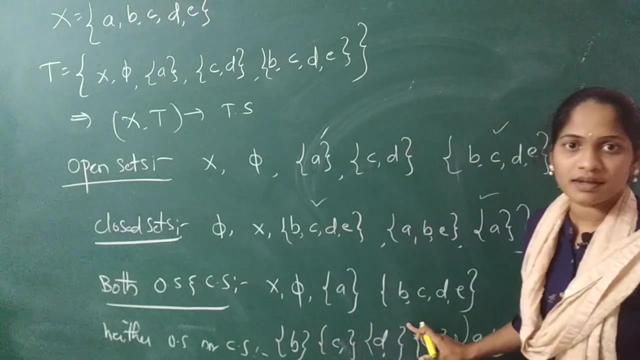 lo same open and close the sets away on die, Adam, I turn the economy condition only. if we open, sense you could compliment. closes, it's a chica da, so ala carcana, same an anirazi, and to me cave it. opens it's a. you say we preach any, both open and closed, on the same away of stay in. 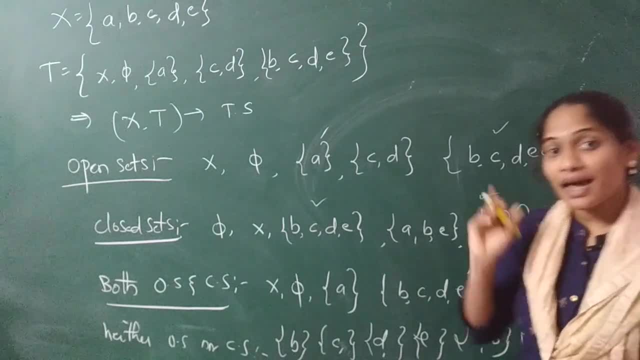 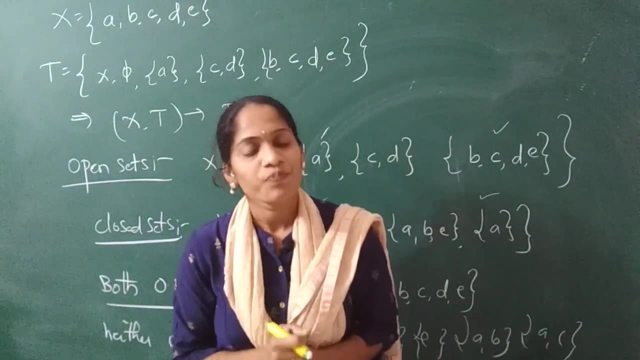 the matter and think extra subset said same window. so Alan took example good untenna and a coin side in the killa. it a discrete in discrete, me coin side. I know a lot of example me topology of it is couldn't a same me cool, open set. 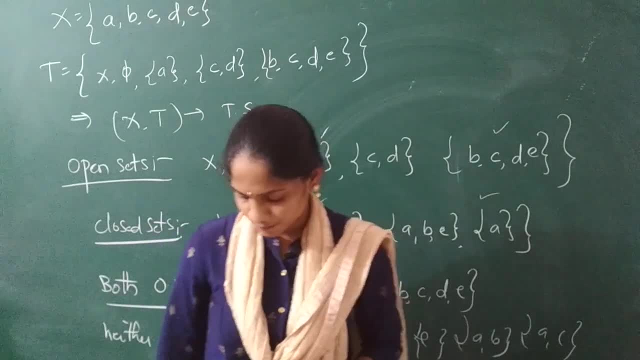 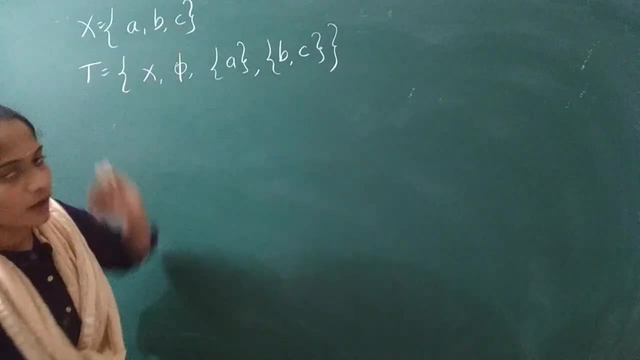 closes, it's gonna coin seductive. let's see that example. now you let me see some example. just I have told you I have taken X is equal to a, comma B, comma C and I have taken tau equal to X, PI, single terms at a and single ordered. 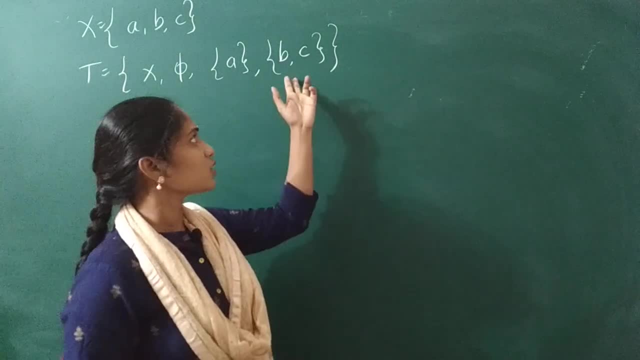 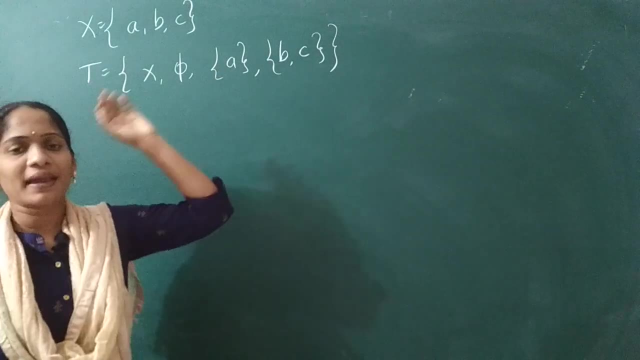 pair, that is, B, comma, C. so now I am saying that this is a topological space. already we have did it done. what is that? if you take the intersection, yes, if you take the union, maybe at the point of these two sets you have to check out. 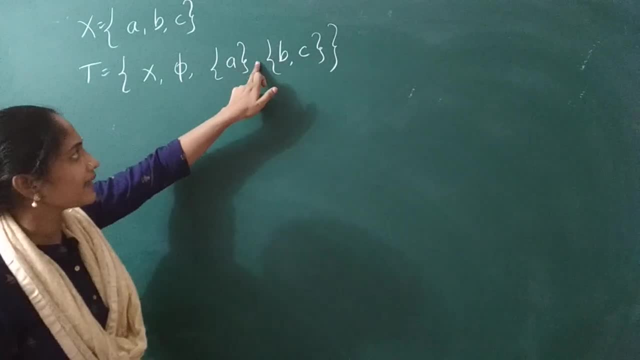 whether the intersection and Union belongs to that set or not. if you take the intersection, there is no common sense. if you take the intersection, yes, if you take the union, how about, if you take the intersection, if there is no common sense? if you take element which is pi, are there, it belongs to tau. if you take the union, it is a comma b, comma c. 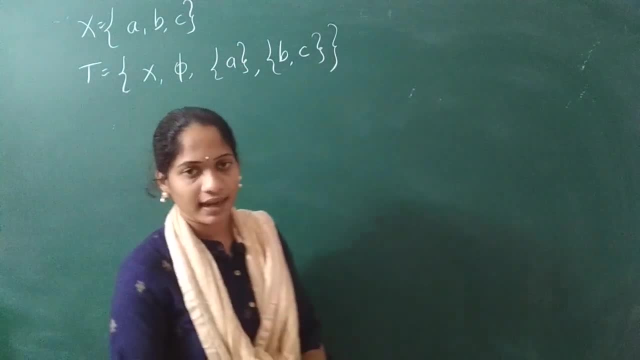 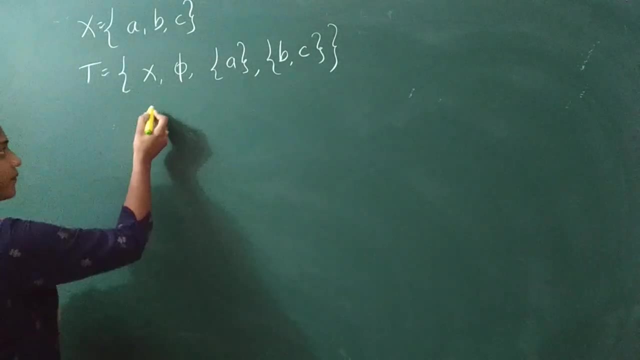 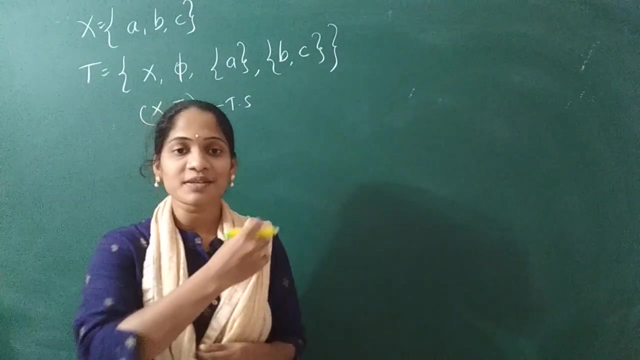 that is nothing. but x. x belongs to tau, yes, the second and third conditions are satisfied and that t is known as a topology. so therefore, what happens here? x, comma, tau is a topological space. right, so now what you have to do. as it became the topological space, the members of 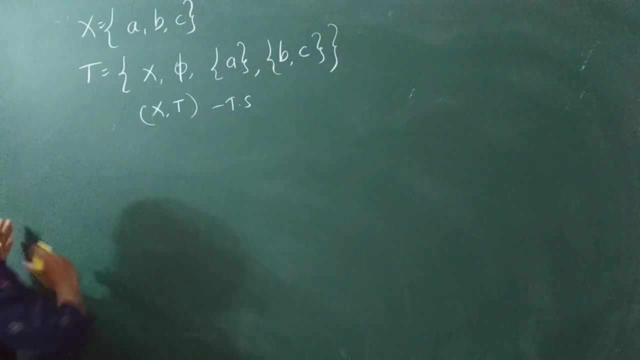 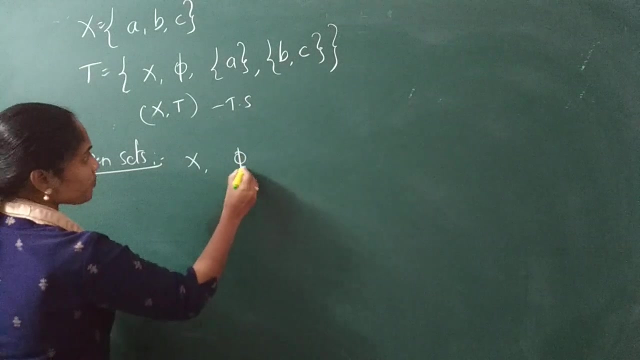 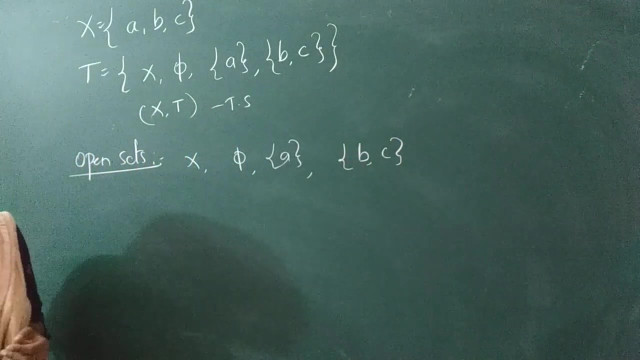 tower, known as what, yes, open sets. so directly, when it, this tau, becomes a topological space, you have to consider these members to be the open set. so now write down what are the open sets. what are the open sets? yes, x and x, pi, singleton set a and b, comma, c. so these four sets are: 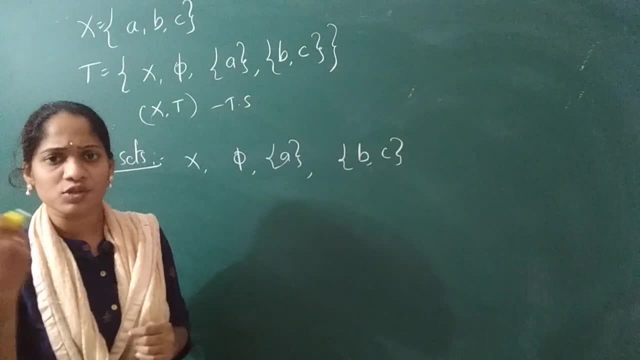 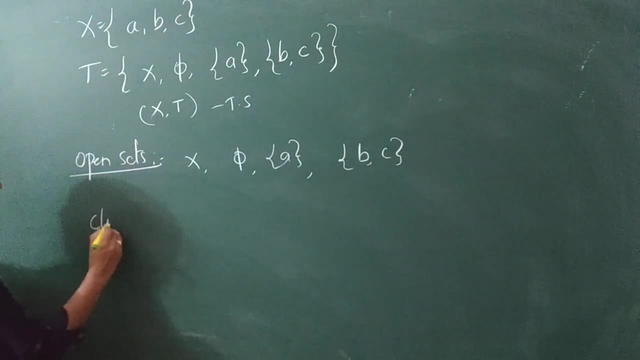 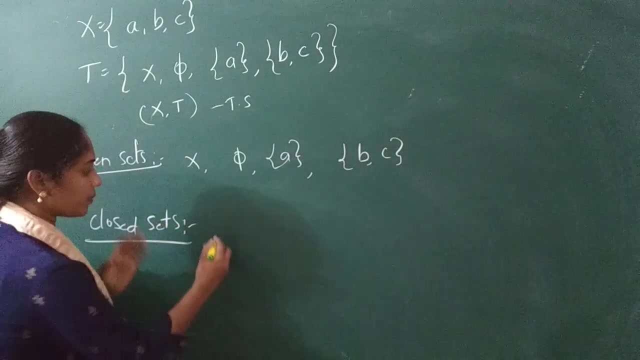 nothing but the open sets compared to the closed sets. what are the closed sets? yes, their complements are nothing but the closed sets. let's find out the closed results also and let's see what happened. what is the miracle is going to be done. what is x complement x? 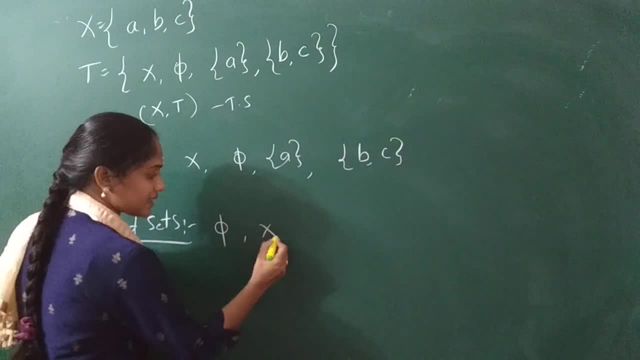 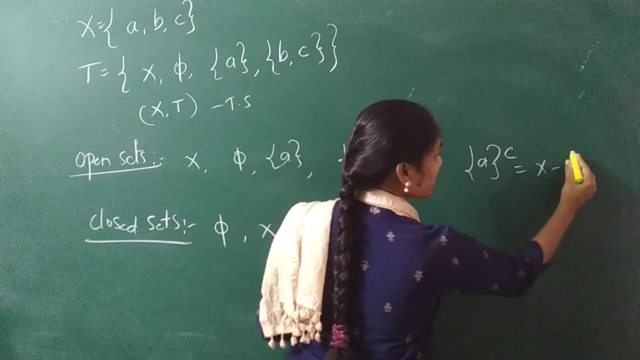 complement is pi, and what is a pi complement? it is x. and what is a complement? a complement is nothing. but you have to do: what is a complement x minus a and what is the set x, a, if you take out the a and next, what is this? b comma c? 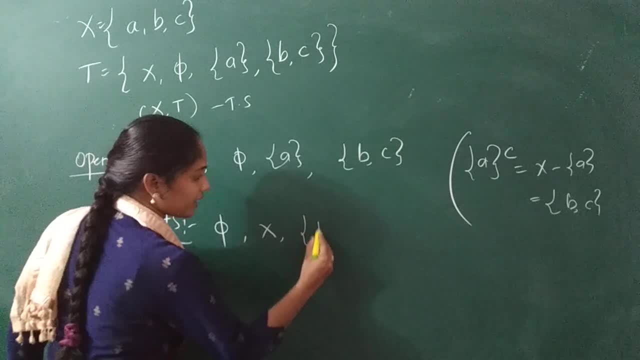 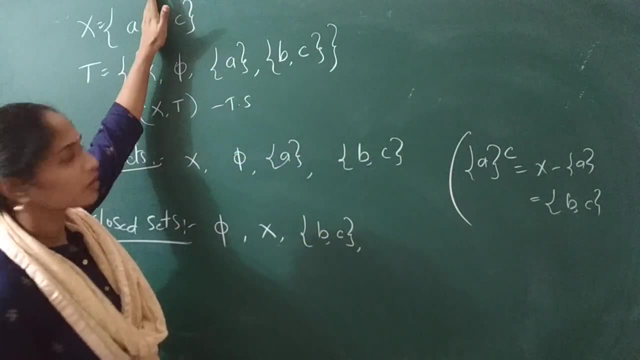 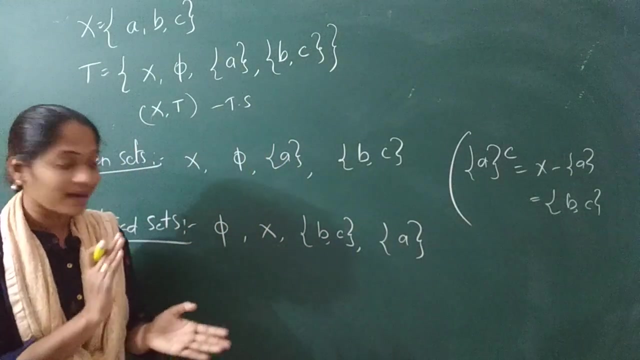 in this way you have to find out. so a complement is nothing but b comma c. if you find out the b comma c complement, what is that x minus b comma c, if you take out the b comma c, and what is the singleton set a? so now let's check whether same sets are there, both open and close: x, x, pi, pi. 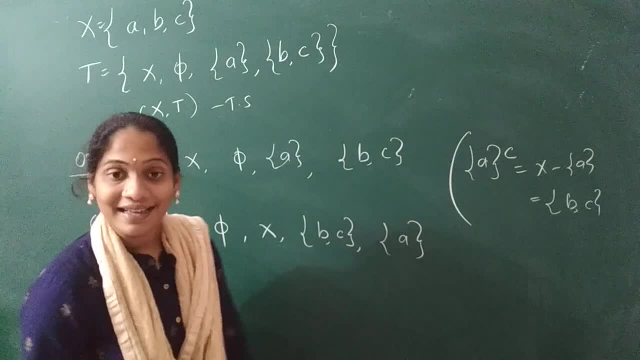 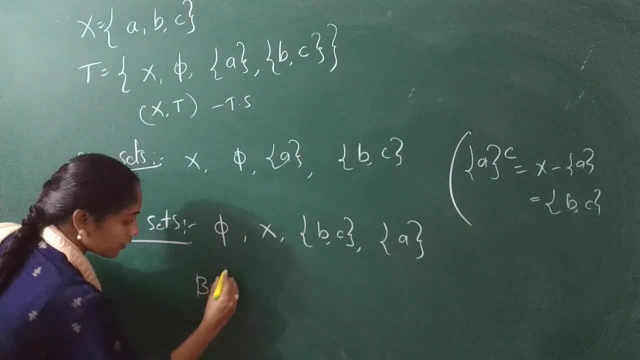 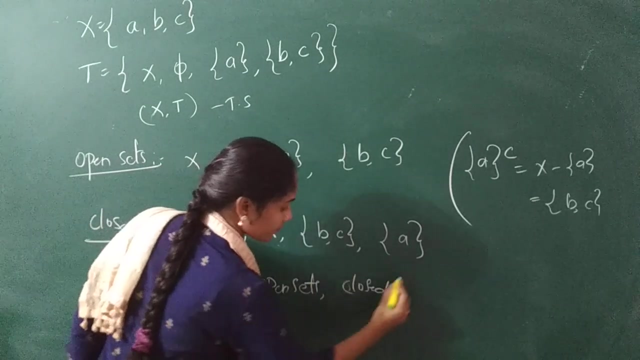 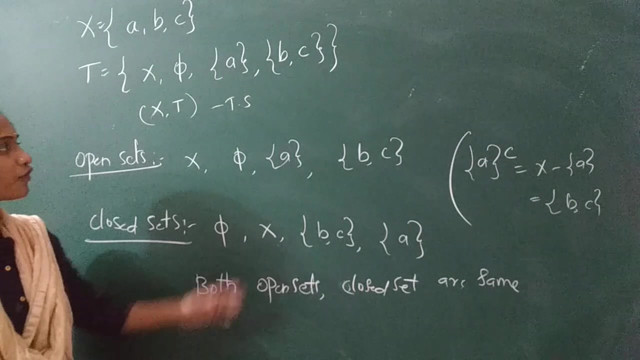 singleton set ends. and how do the b, comma, c? yes, here open sets and closes are getting coincide. so both open sets and closed resets are same, or you can say they are getting coincide. so in this way you can check out or find out the open sets and closed the sets. one example: 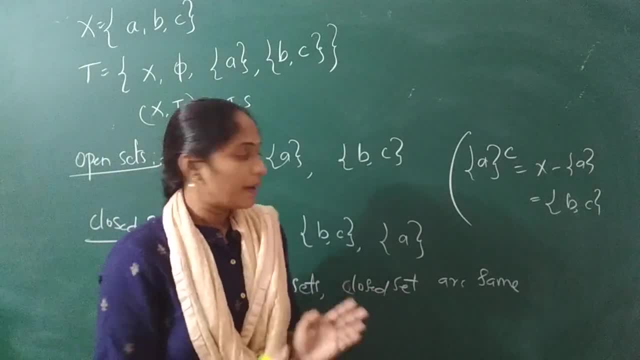 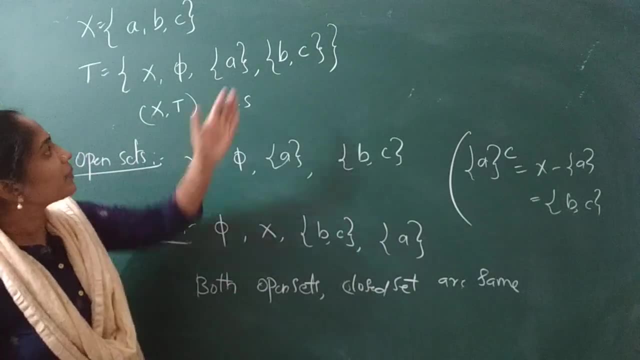 is Till now. we got some same, but some closed sets are same and some are not, So this example says that the same sets are not there yet. If you take different subsets, you may get something different, But for the subsets that I took E what happened to me. 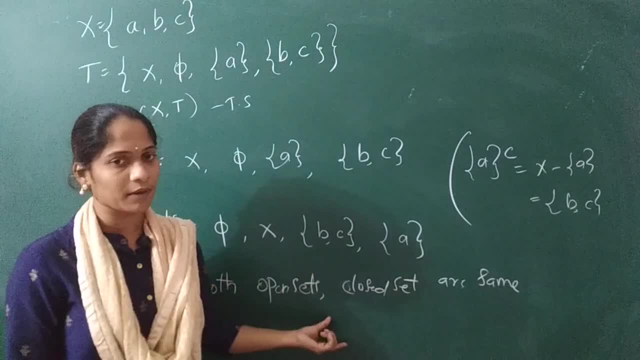 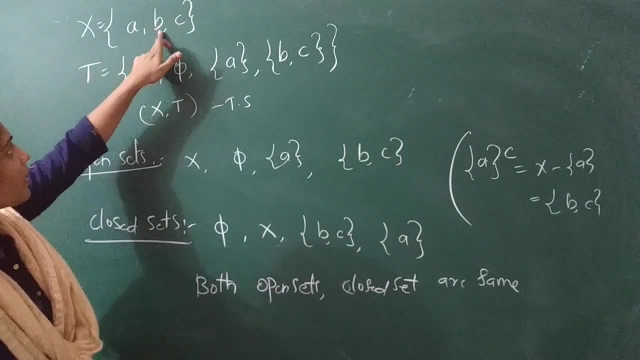 Both open, closed sets and open sets are the same, So neither and none will come here. Will they come or not? Single 10 set B will come. Single 10 set C will come. A comma B will come Next, what else will come? 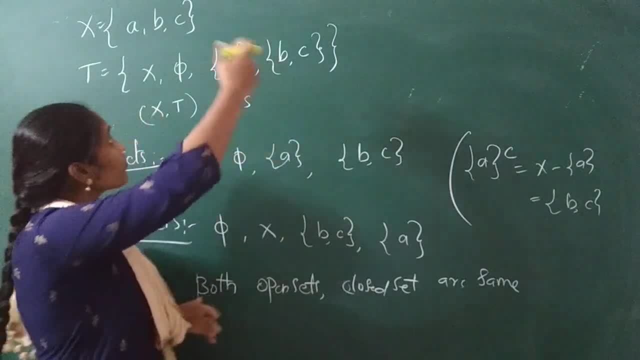 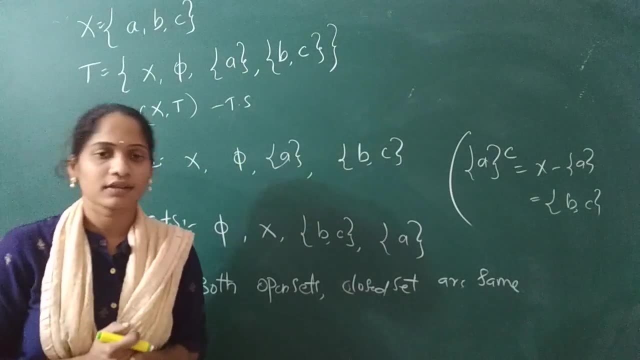 A, B, C and X will also come. So because of that, 2 cubes, that is 8.. So already we have 4 here and there are 4 more sets. What will happen to those 4 sets? Neither and none will come. 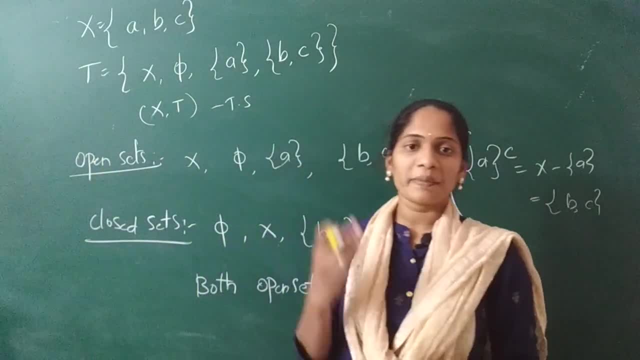 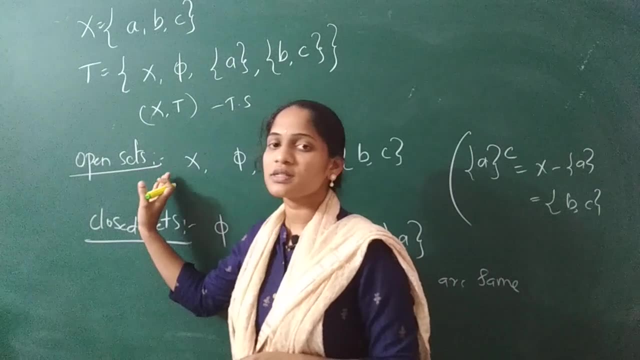 So in this way, if you give X, you have to find out open sets and closed sets. Please remember this again, Please, students. it is very important to check out whether they are open sets or closed sets or not. First you have to check whether this is a topology or not. 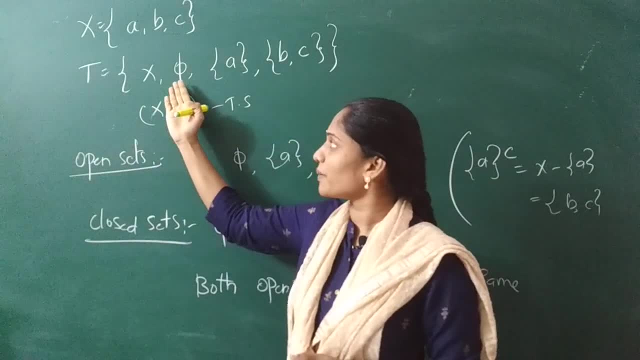 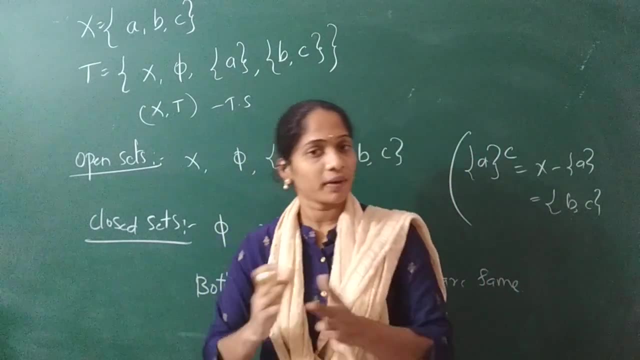 As it has become the topology, then you have to find out. these members are nothing but the open sets. Their complements are nothing. They are nothing but the closed sets. So there are some sets which are both open and closed And there are some more sets which are neither and none. 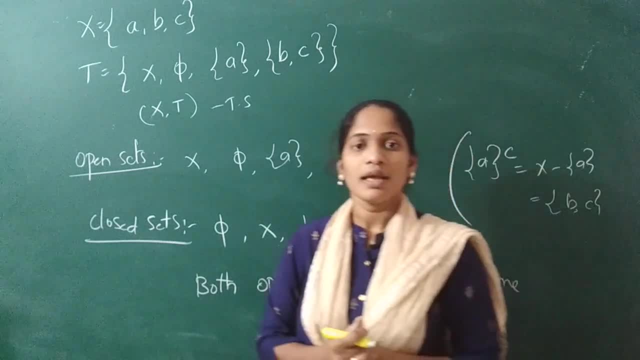 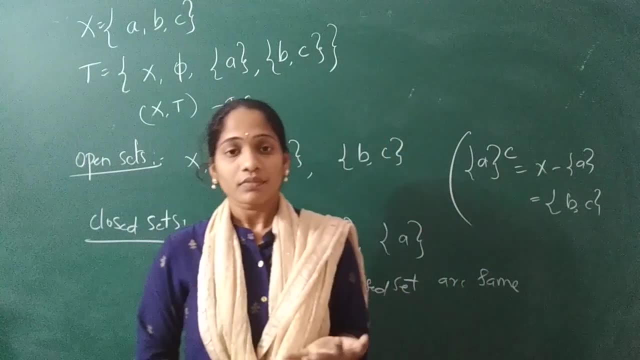 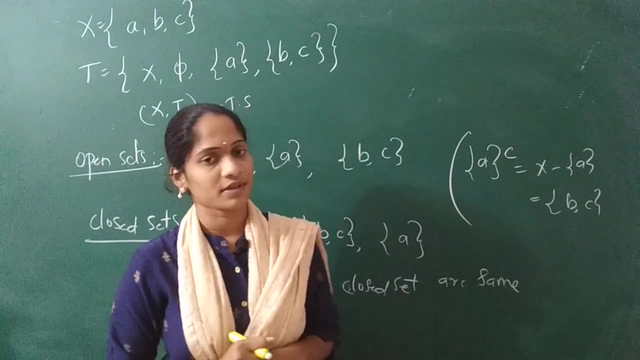 And there are some sets which coincides, like open and closed sets. So this is some definitions, basic definitions in a topology, What we have discussed here- topological space, open sets and closed sets, discrete and indiscrete topology, co-finite and co-accountable topology, with some examples. 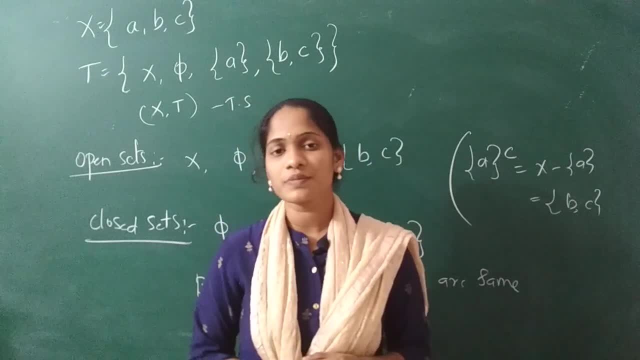 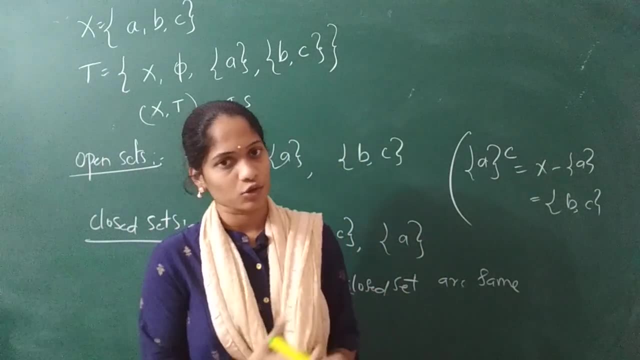 So in the next video I am going to upload some small problems and proofs. there is theorems which may be help you. These are some definitions, which are basic definitions in the topological space. If you want more definitions or examples, you can comment me in the comment section. 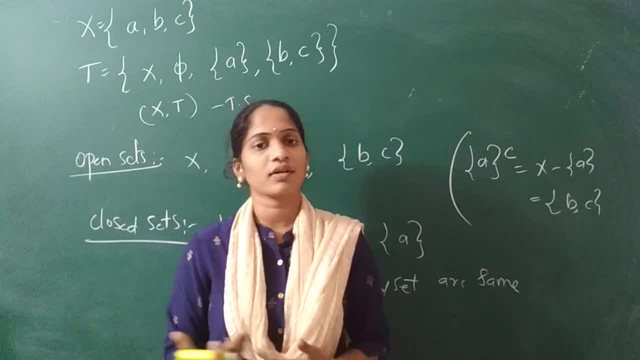 If it is helpful for you or any students or relatives, you can share the videos. Thank you for watching. Please subscribe and share. 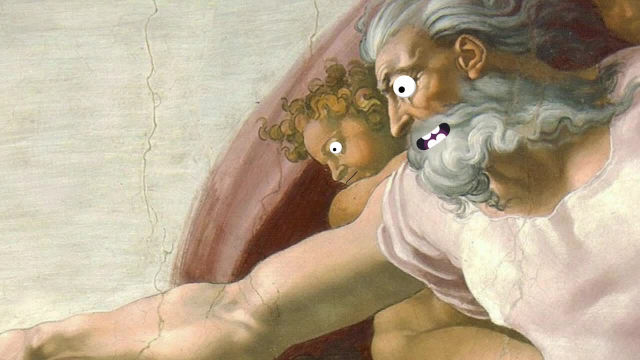 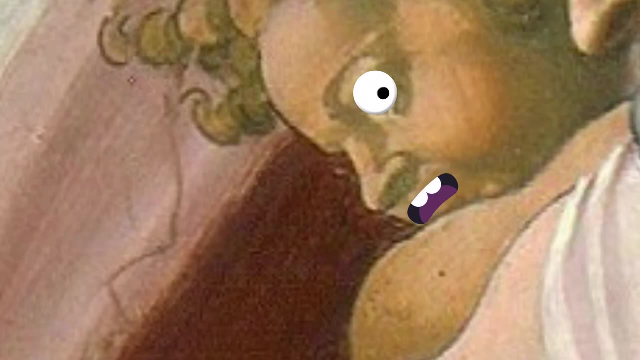 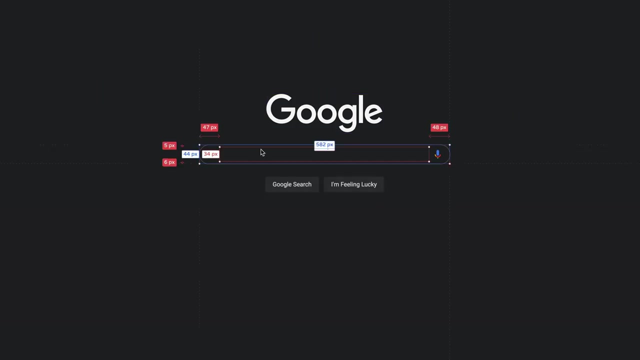 And what will you do upon this world I have created for you? I, uh, I was planning on just building some boxes on the web. Seriously, though, your browser represents each element on a web page as a rectangular box. This concept is known as the CSS box model, and this is how it works. First, you have your content. 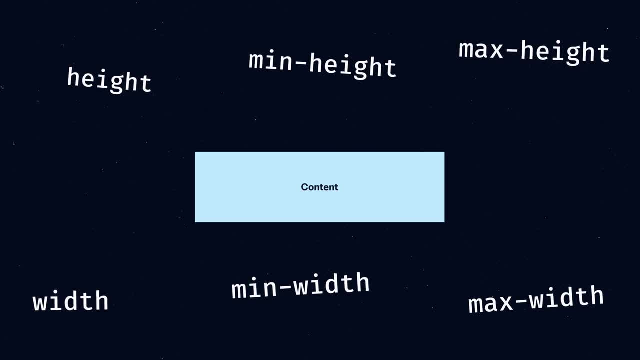 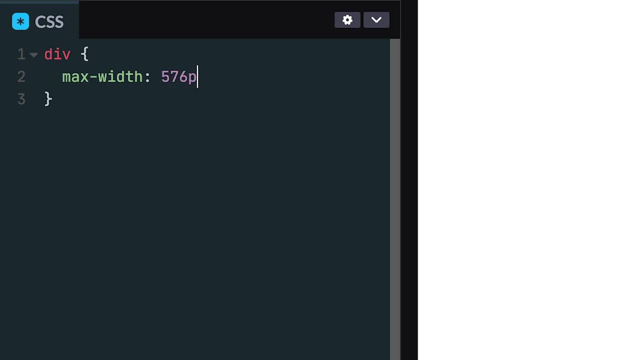 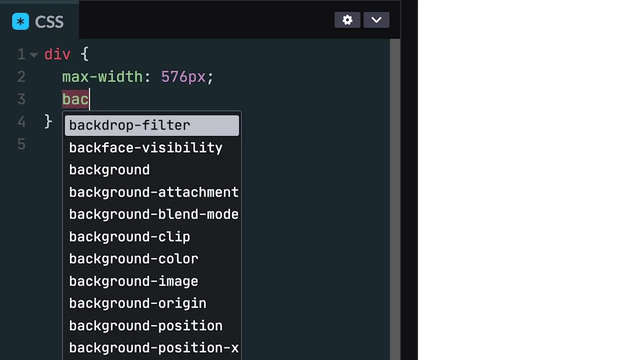 area. Using these CSS properties, you can give a content area a set height and width. For example, let's give this divider a max width of 576 pixels. The height will have the default behavior of taking up as much space as the content needs. I'll also add a background color to this divider, so it's. 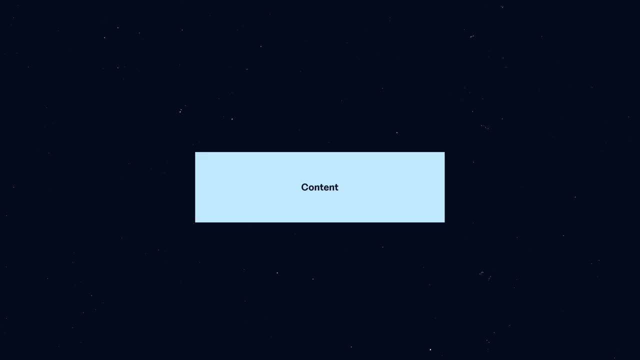 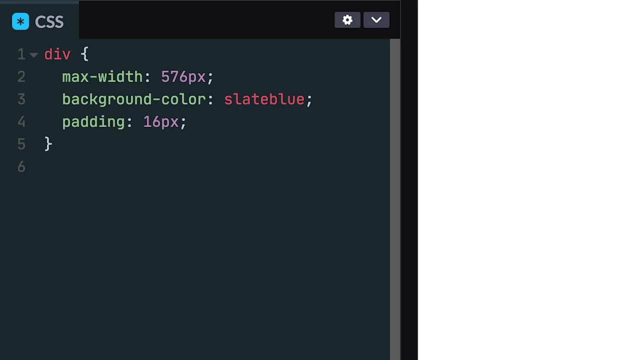 easier to see the box boundaries. Next, you can use padding to clear space around the content. By adding 16 pixels of padding to the divider, you'll see the content now has some extra room from the side of the divider. After padding comes borders. I can add a border outside the